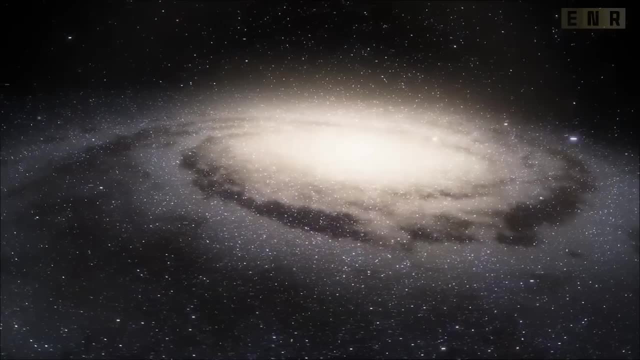 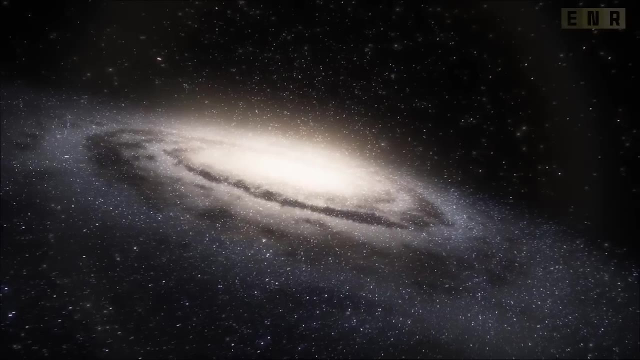 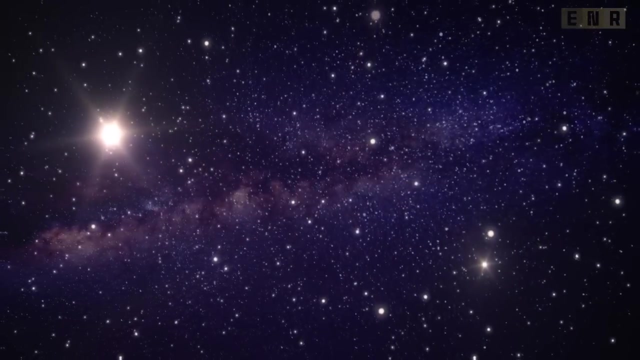 Approximately 12 billion years old. the galaxy is a vast disk with enormous spiral arms and a central nucleus. It is only one of countless galaxies in the universe. Galaxies are massive assemblages of stars, first and foremost. A typical galaxy could contain 100 billion stars. 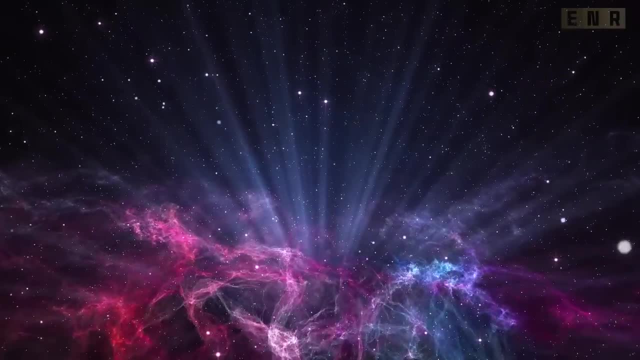 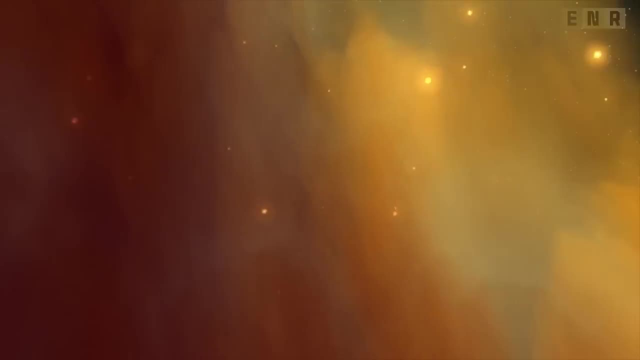 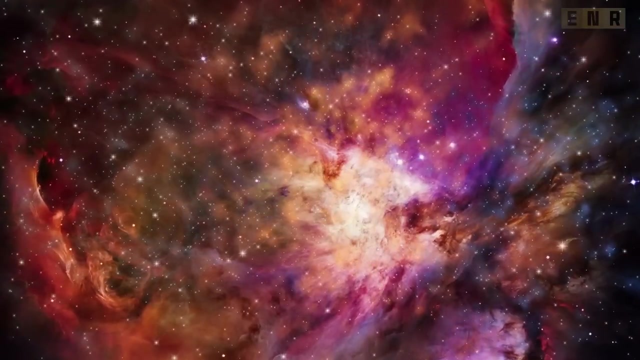 They are actually stellar nurseries, the locations where stars are formed and perish. The stars in a galaxy are formed in nebulas, which are concentrations of dust and gas. Our galaxy contains billions of stars, Many of which have planets and moons orbiting them. 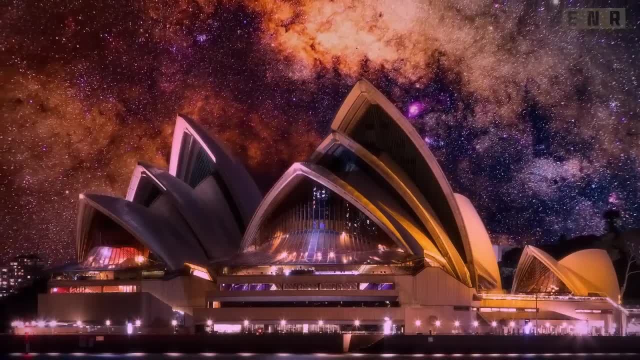 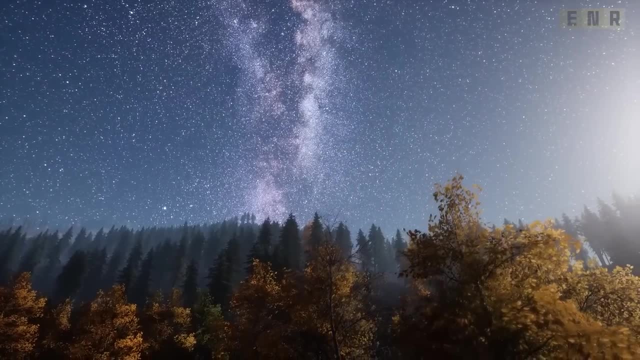 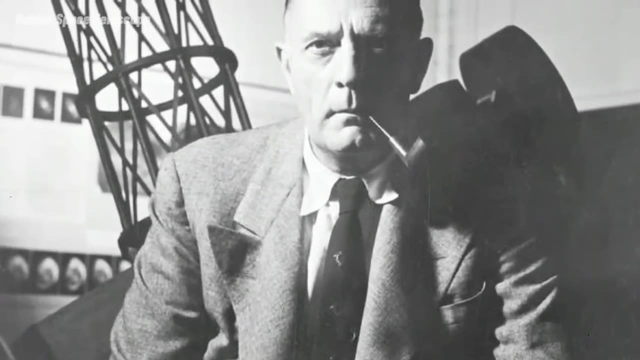 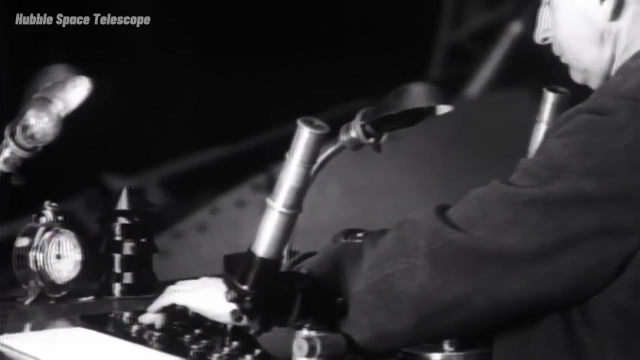 But for a very long time we knew very little about galaxies. A century ago, we believed that the Milky Way was the only galaxy in the universe. In 1924, astronomer Edwin Hubble altered the entire situation. Hubble observed the universe using the most sophisticated telescope available at the time. 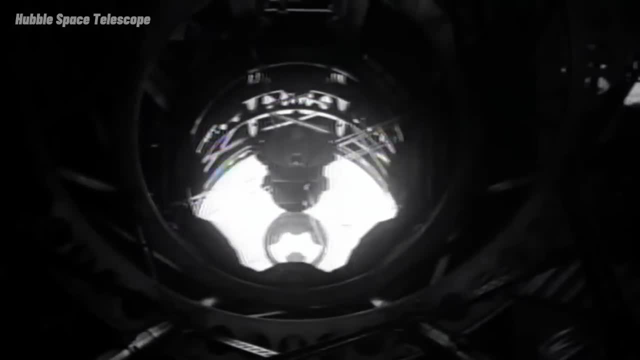 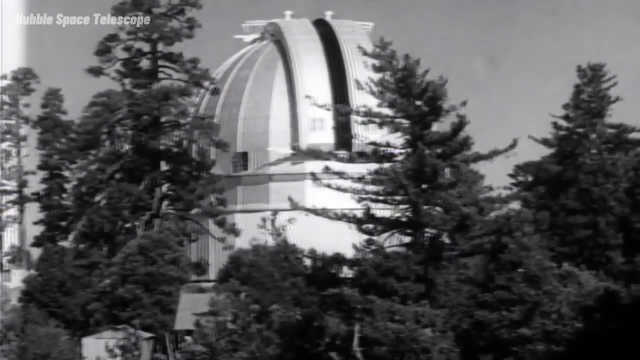 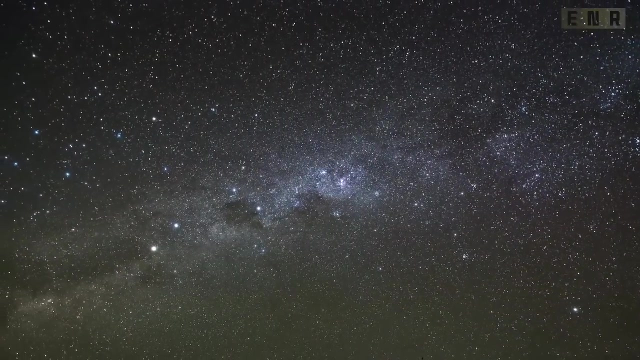 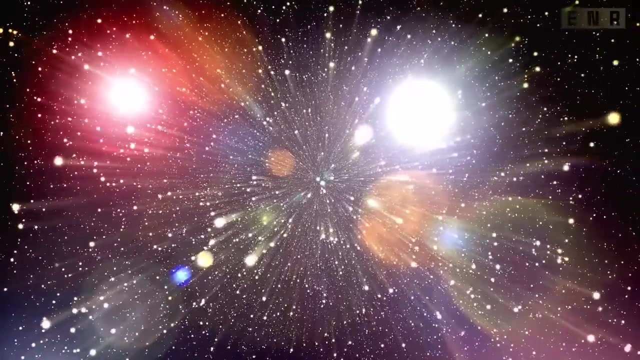 The 100-inch hooker on Mount Wilson near Los Angeles. Far, far away he saw hazy masses of light in the darkness of the night sky. He realized they were not even separate stars. They were entire star-filled cities, Constellations far beyond the Milky Way. 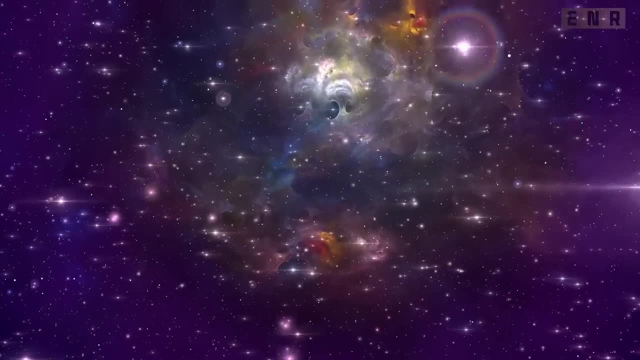 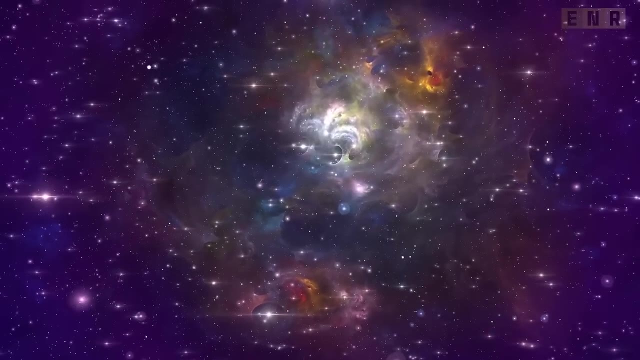 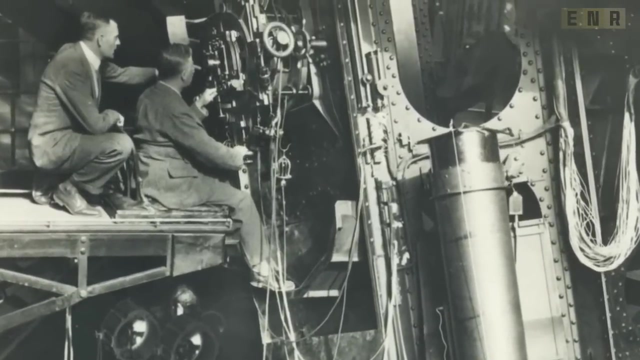 The astronomers received an existential jolt. We went from the Milky Way galaxy being the only galaxy in the universe to billions of galaxies in a single year. Hubble made one of the finest discoveries in the history of astronomy when he discovered that the universe contains a large number of galaxies rather than just one. 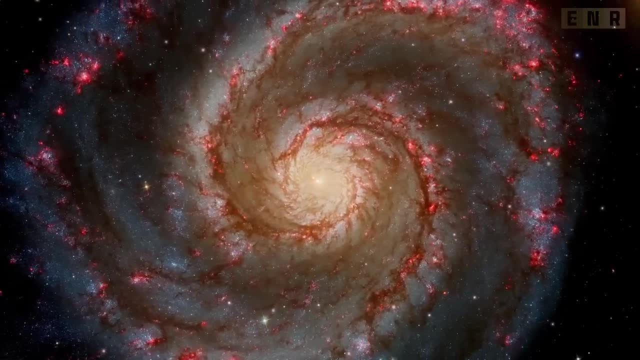 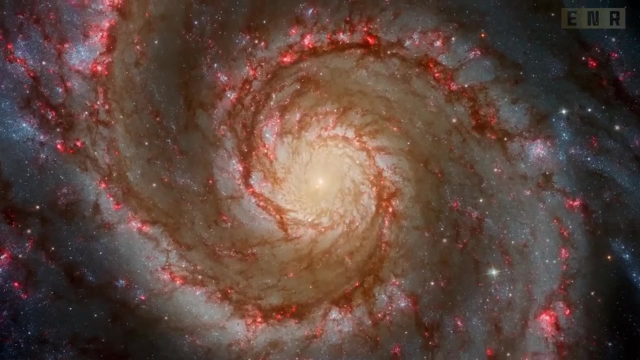 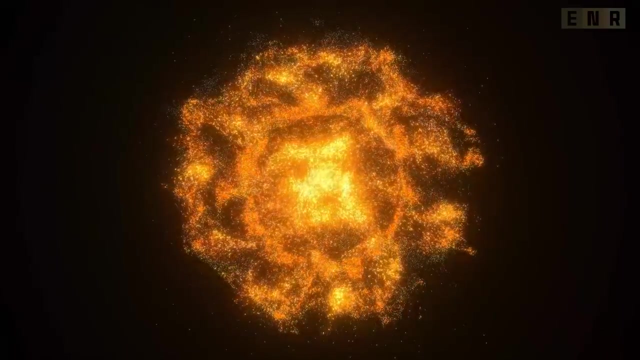 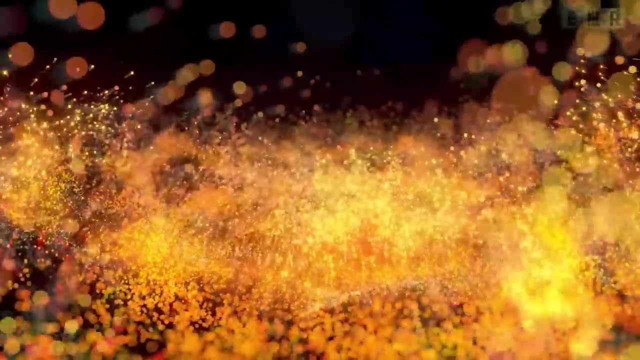 This is the Whirlpool galaxy. It comprises over 160 million stars and is characterized by two enormous spiral arms. In addition, the stars of the huge elliptical galaxy M87 shine with a golden hue, since it is one of the oldest galaxies in the cosmos. 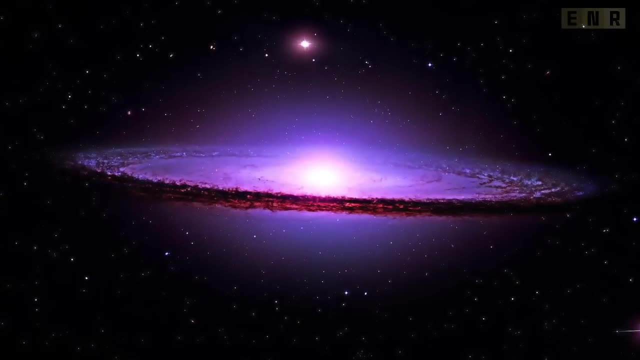 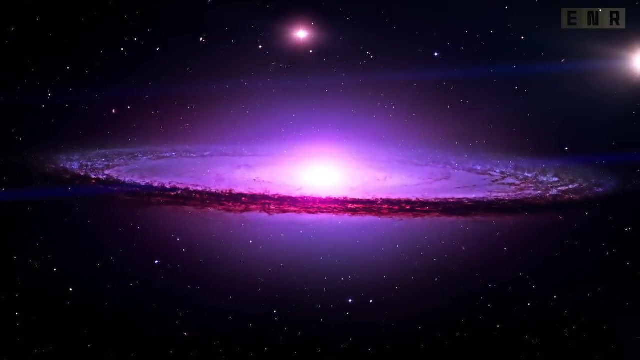 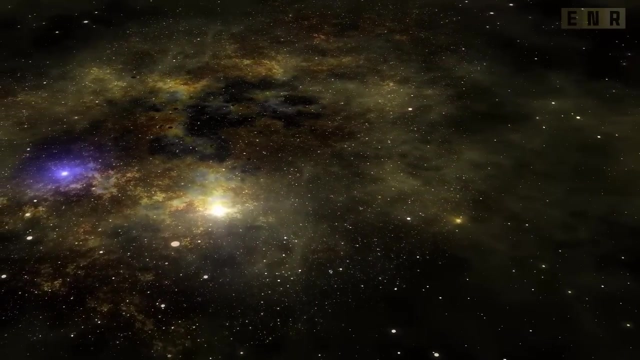 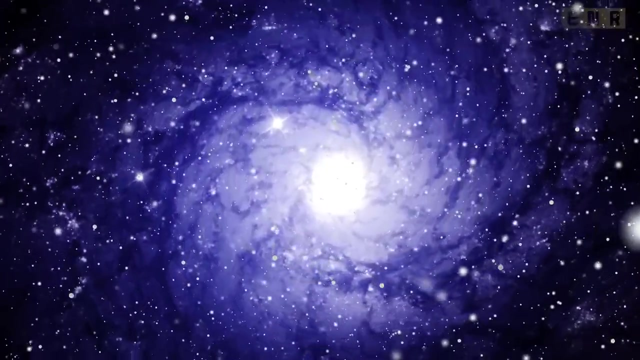 And this is the Sombrero galaxy. Its massive bright core is surrounded by a cloud of gas and dust. All galaxies are very beautiful. They stand in for the fundamental building block of the cosmos. As they spin across space, they resemble enormous pinwheels. 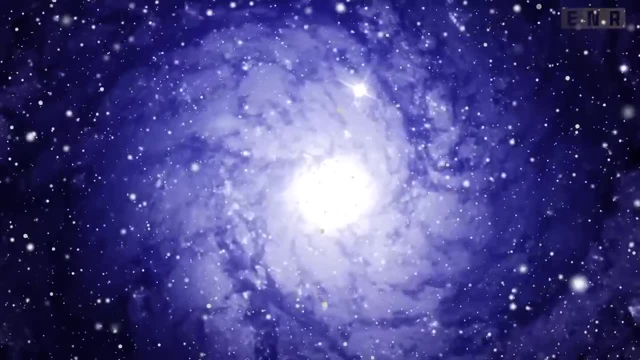 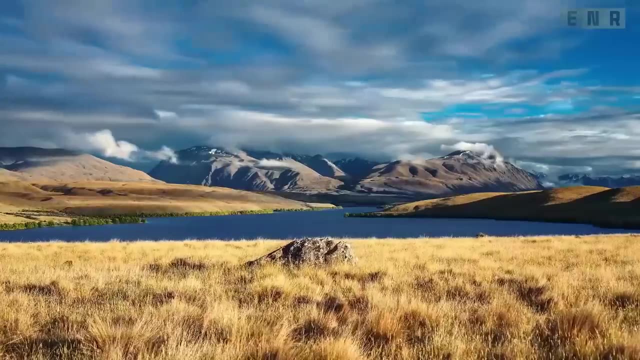 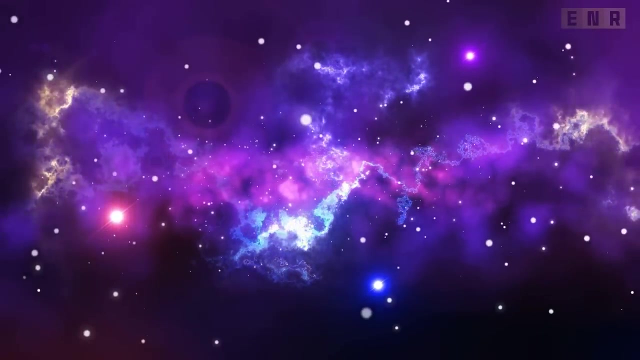 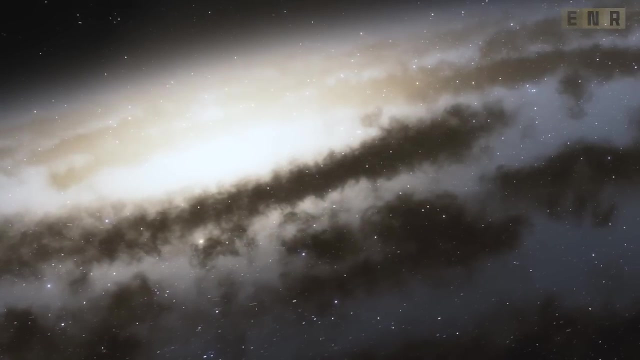 Galaxies are enormous on a grand scale. On Earth, we measure distance in miles. In space, astronomers use light years. This is how far light can travel in a year. Our galaxy's diameter is over 100,000 light years and we're now located at a distance of 25,000 from its center. 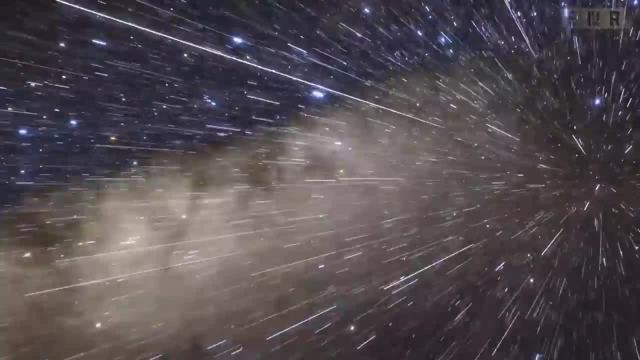 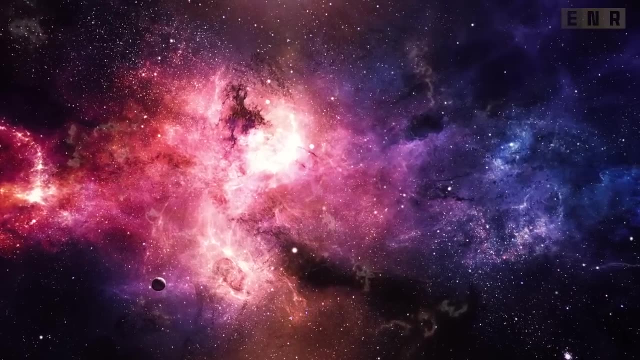 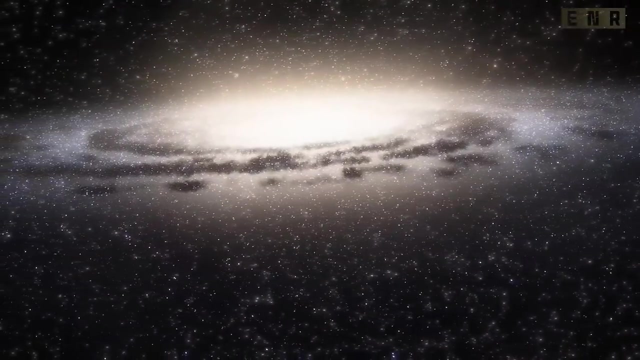 However, in the grand scheme of things, even it seems like a tiny dot. While the Milky Way seems enormous from Earth, when compared to other galaxies it is really rather little. Andromeda, the galaxy closest to us, is about 200,000 light years wide. 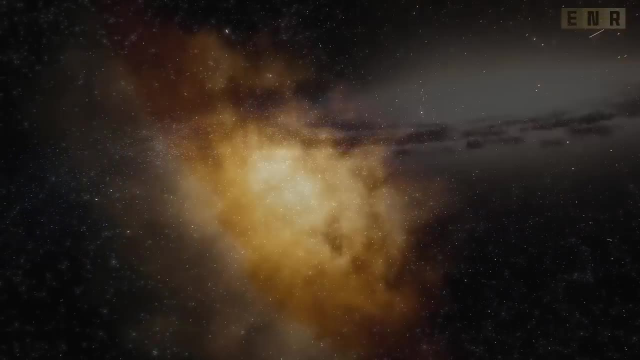 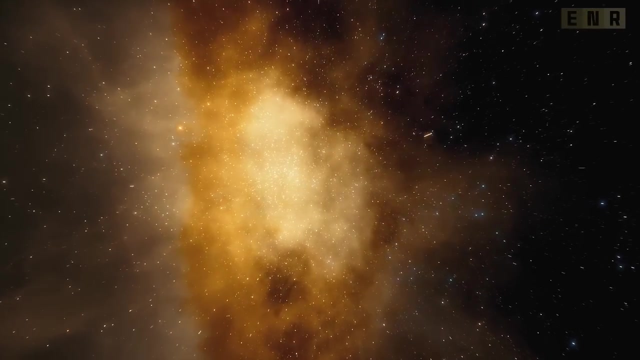 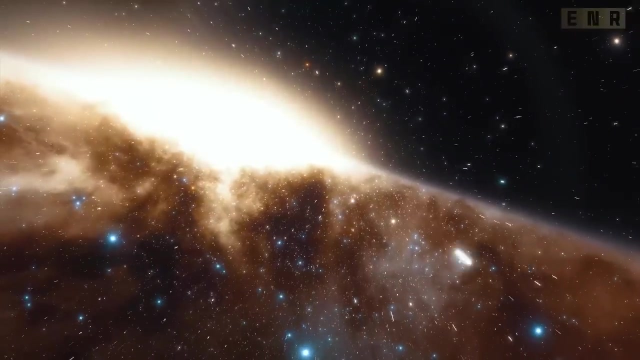 making it twice as large as the Milky Way. M87 is the largest elliptical galaxy in our own cosmic backyard and much bigger than Andromeda, But M87 is tiny compared to this giant Six million light years across. IC 1011 is the biggest galaxy ever found. 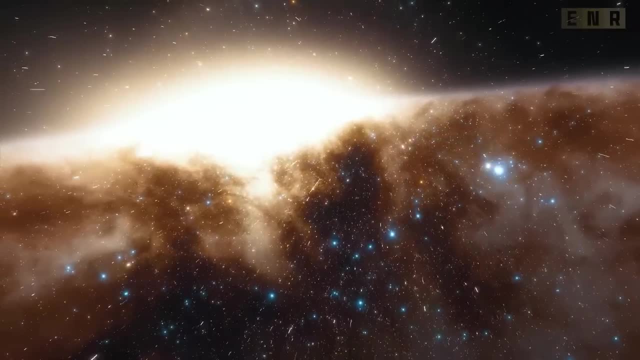 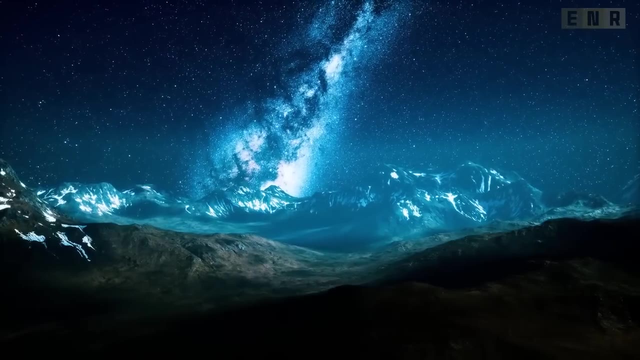 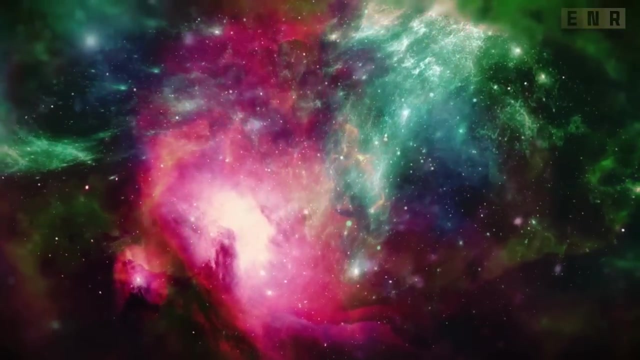 It's 60 times the size of our own Milky Way. It's common knowledge that galaxies are enormous and ubiquitous, But why is this the case? The origin of galaxies is a key mystery in astrophysics. Approximately 13.7 billion years ago, 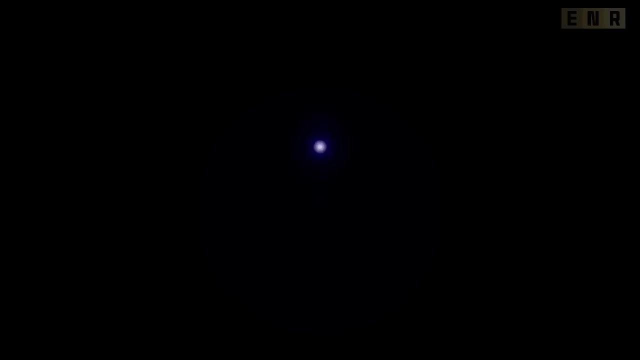 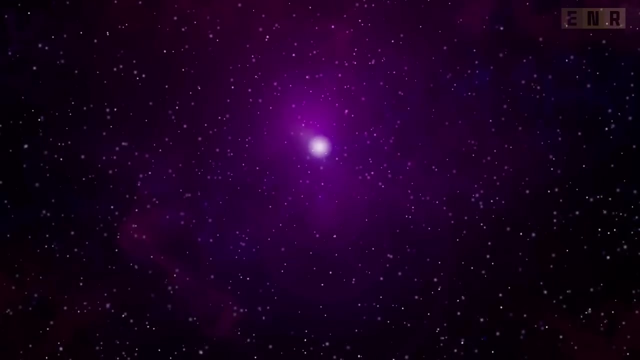 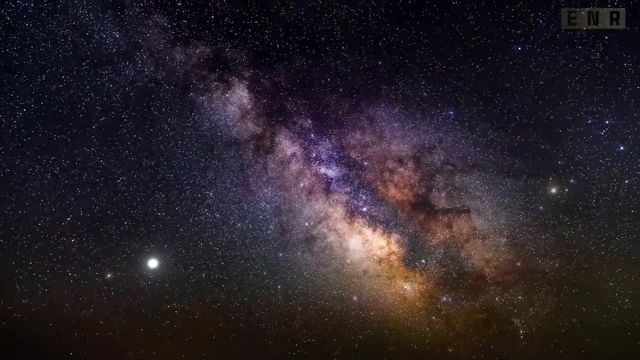 the universe began with what we refer to as the Big Bang, a period of intense heat and density. We know that there could not have been anything like a galaxy at that time, So galaxies must have come from that very early universe and formed from it. 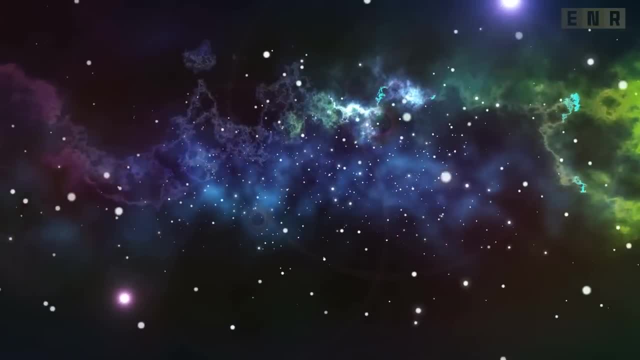 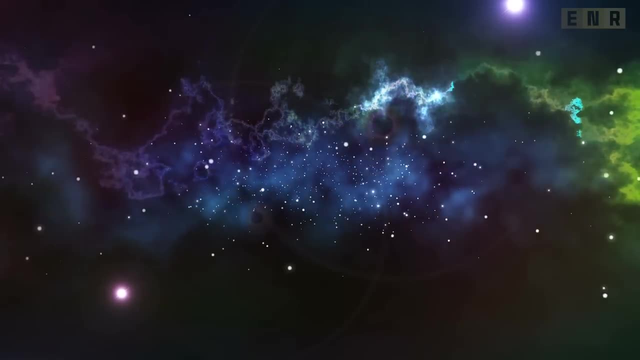 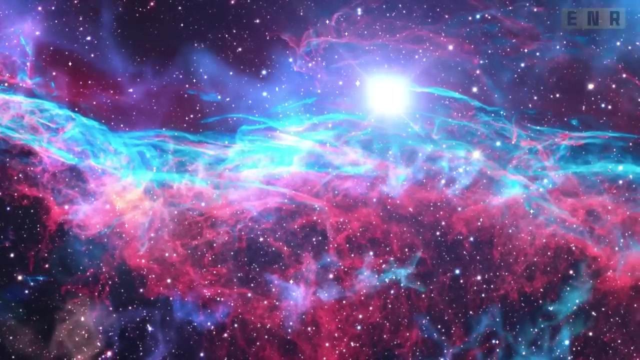 For stars to form and for galaxies to form from those stars, gravity is essential. After the Big Bang, the first stars began to emerge only 200 million years later. The earliest galaxies formed as their masses began to clump together because to gravity. 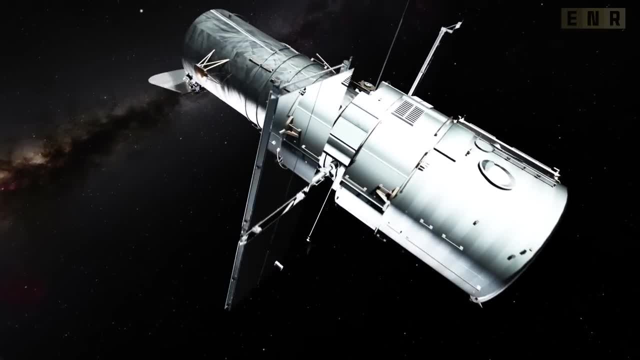 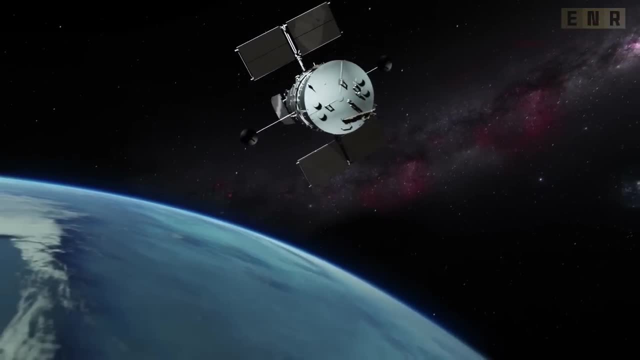 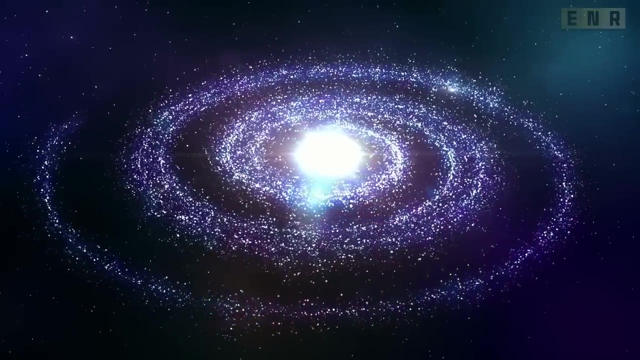 Thanks to the Hubble Space Telescope, we can now see the early universe, when galaxies were just beginning to form. Numerous galaxies are visible to the Hubble. the light we see from distant galaxies now, However, really departed those objects many millions or perhaps billions of years ago. 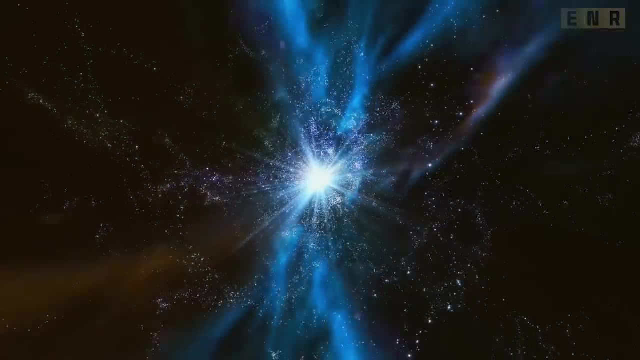 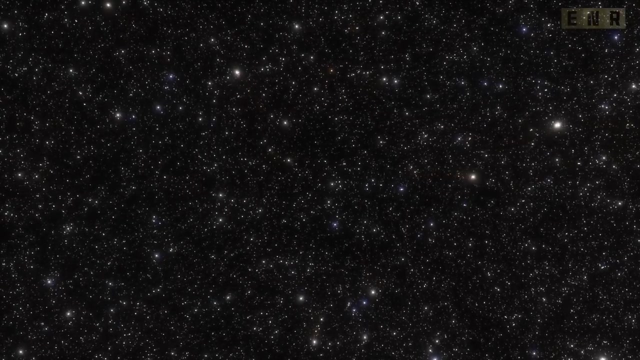 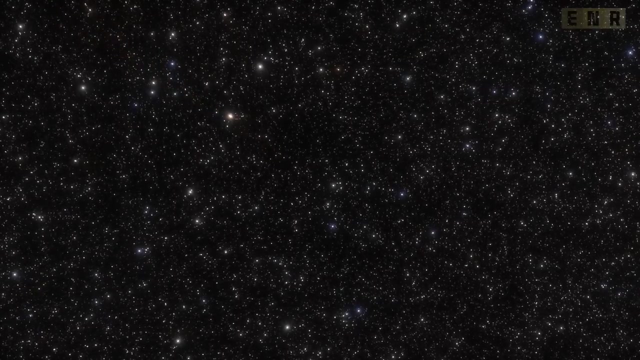 What we see now is the distant past of those galaxies, since it took so long for their light to get to us. The Hubble Deep Field reveals a collection of fuzzy dots. They are quite different from the galaxies we see now. We can hardly make out these little specks of light. 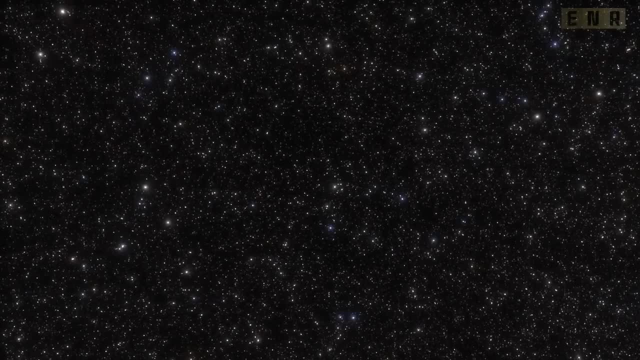 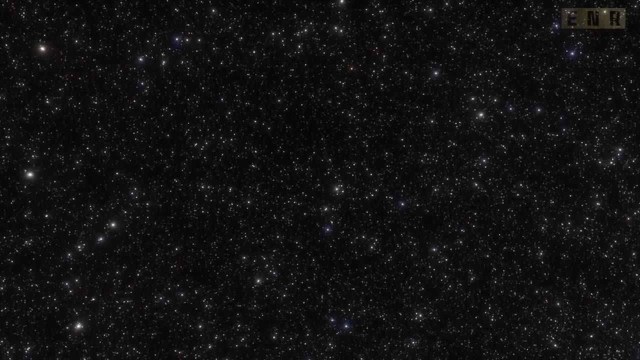 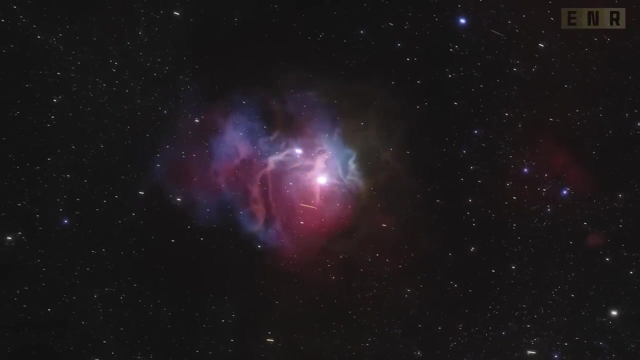 Those fuzzy patches of light are really millions or billions of stars beginning to combine. The oldest galaxies are represented by these barely visible blotches. They began to take shape around a billion years after the Big Bang. However, Hubble's range of visibility ends there. 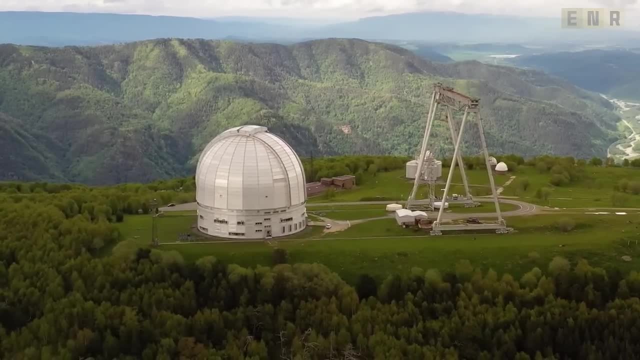 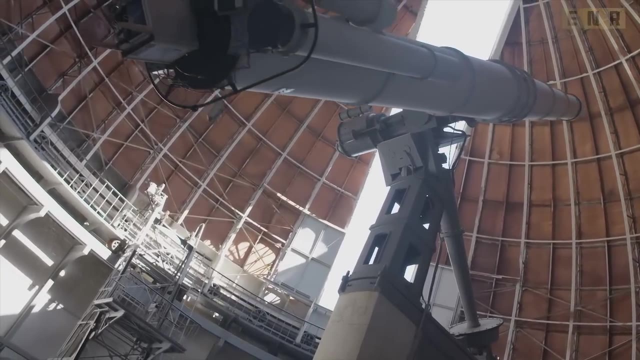 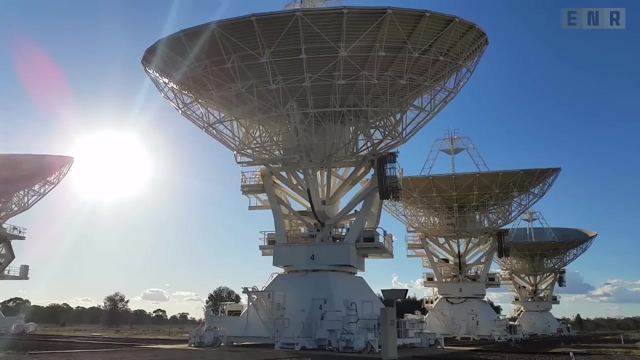 A second sort of telescope, one too large to send into space, is required if we are to travel much farther back in time. Not only can the telescope identify primordial galaxies, but it can also trace their evolution. The evolution of galaxy and galaxy cluster formation may be followed. 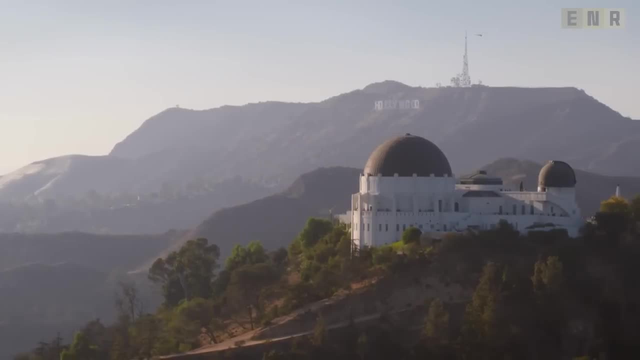 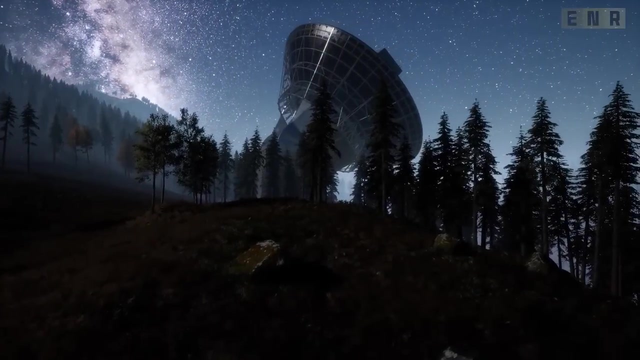 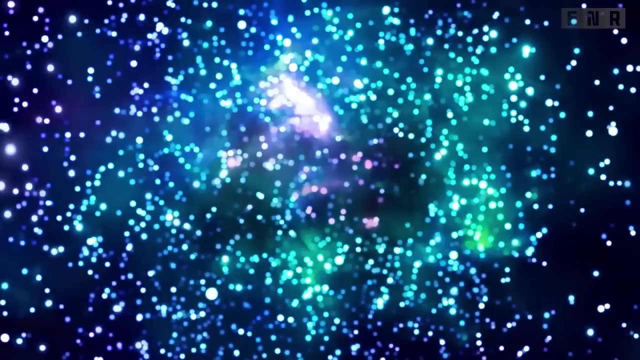 All the galaxies that have developed since the cosmos was just a few hundred thousand years old are leaving their imprints for us to observe. Finally, scientists can begin to answer the question: what did young galaxies look like? Galaxies have evolved from clusters of stars to the complex web of systems we see today. 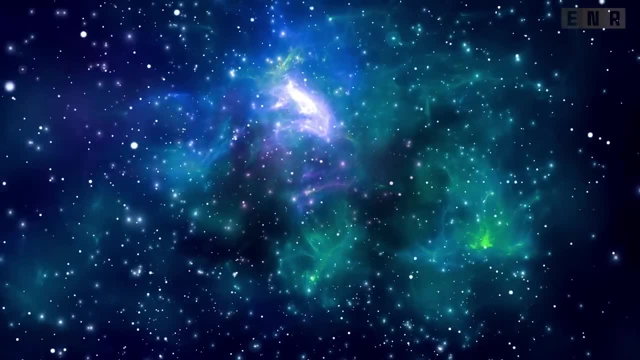 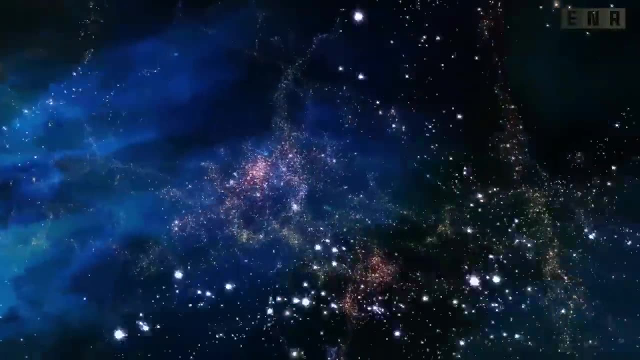 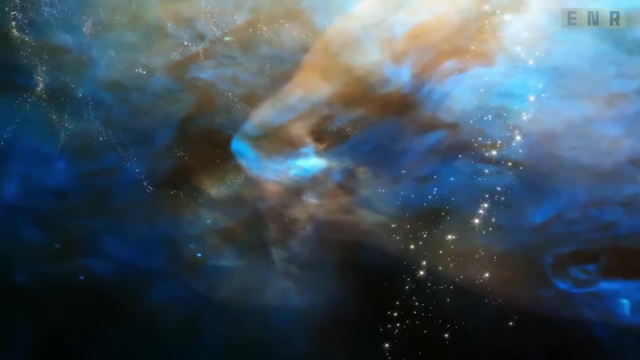 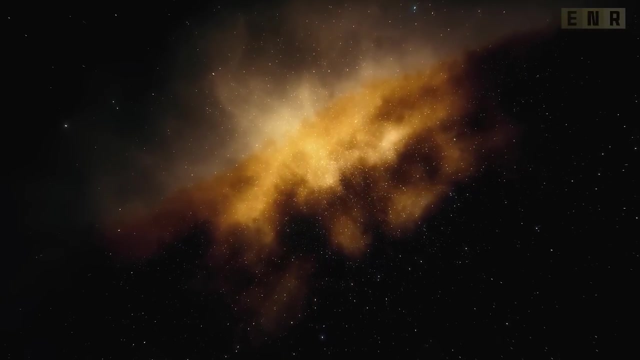 and this process is being seen by astronomers. As far as we can tell, the greatest structures in the universe today originated as star clusters evolved into galaxies, formed clusters of galaxies and ultimately coalesced into superclusters of galaxies. There was a lot of stardust gas and clumpy structures in the early galaxies. 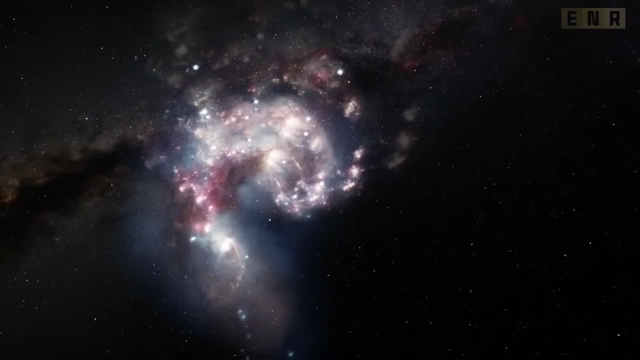 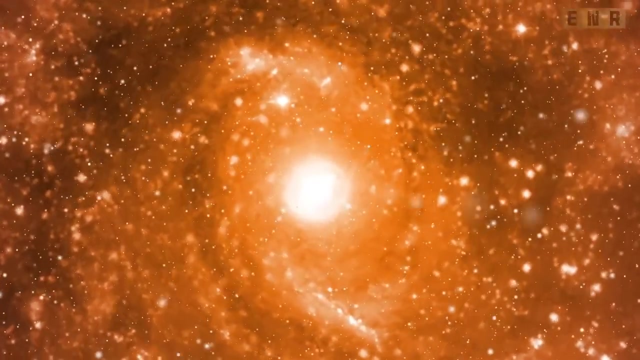 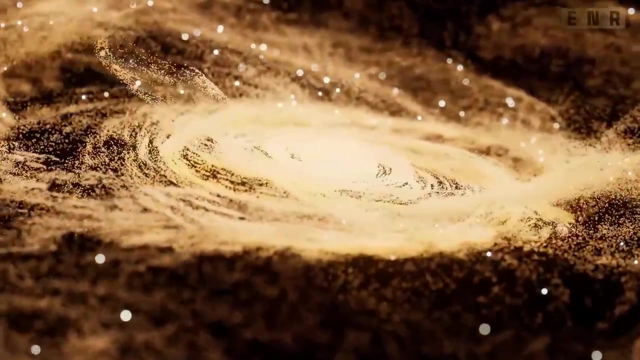 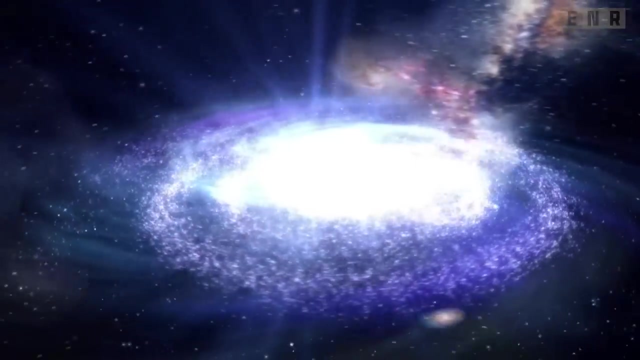 However, modern galaxies seem organized and tidy. When and how can tangled clusters of galaxies become neatly organized spirals and pinwheels? Gravity is the explanation. Galaxies are molded by gravity and its effects determine their fate. At the center of most galaxies lies an unfathomably strong and destructive gravity source. 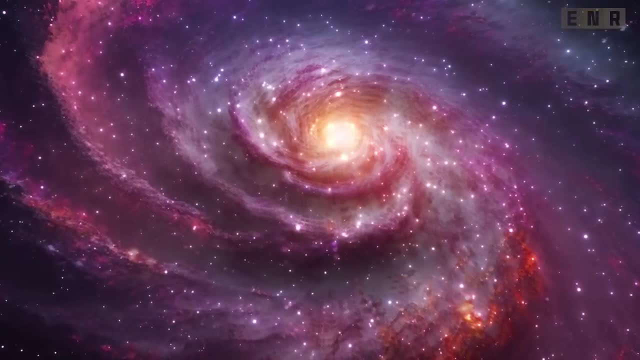 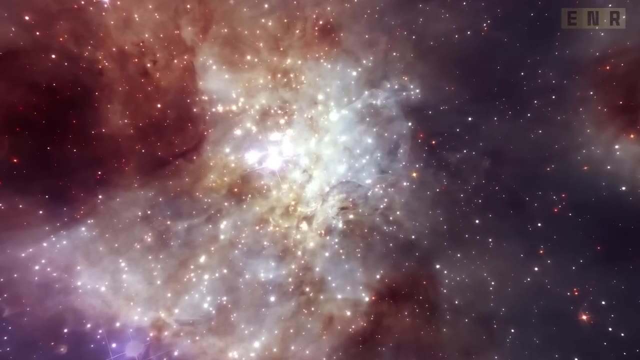 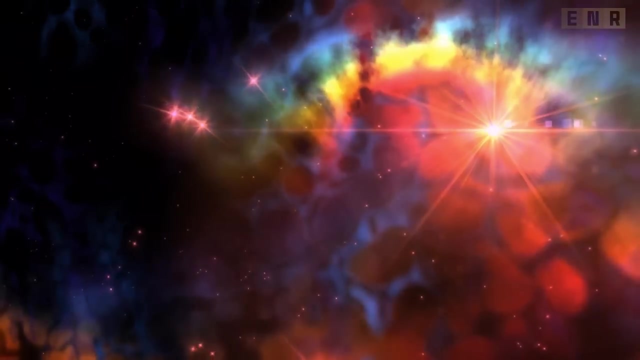 And our own Milky Way has one hidden at its core. Over 12 billion years have passed since galaxies first appeared. These stellar conglomerations may take many forms, from spirals to giant spheres of stars. as far as we can tell, However, there is still a great deal we don't understand about galaxies. 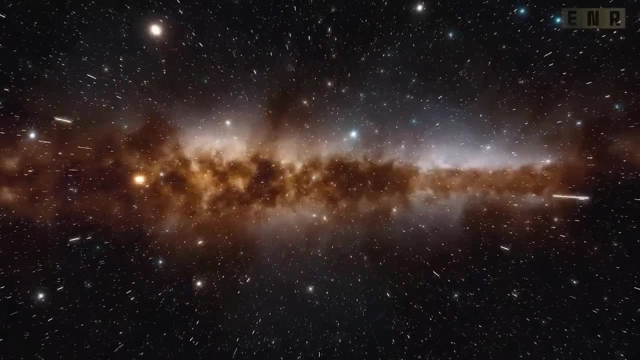 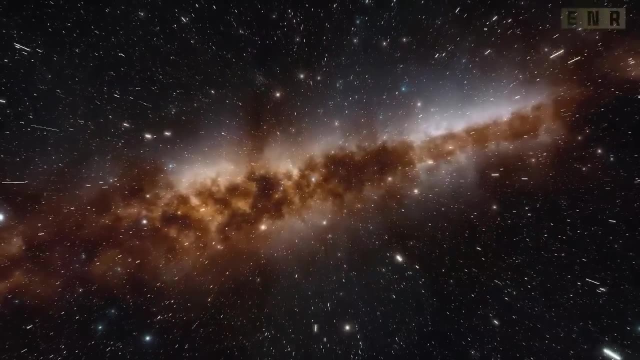 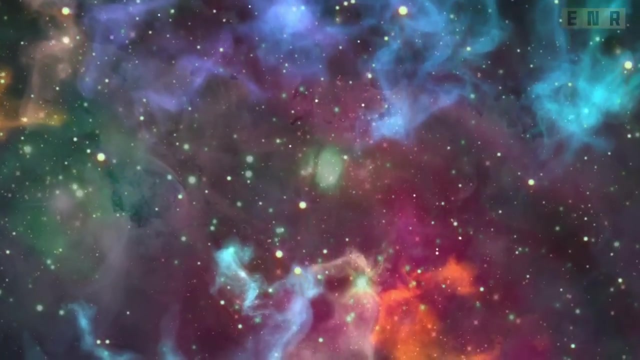 How did galaxies evolve into their present forms? Did spiral galaxies always have to be spirals? The answer is almost certainly no. Young galaxies are a mix of stars, gas and dust. They are untidy and chaotic. They begin as chaotic formations like the Whirlpool Galaxy. then, over billions of years, develop into more orderly forms. The Milky Way wasn't born from a single galaxy, but from a cluster of several. Our Milky Way originated as a collection of disparate formations, objects of varying sizes and shapes that gradually merged to become the galaxy we see today. 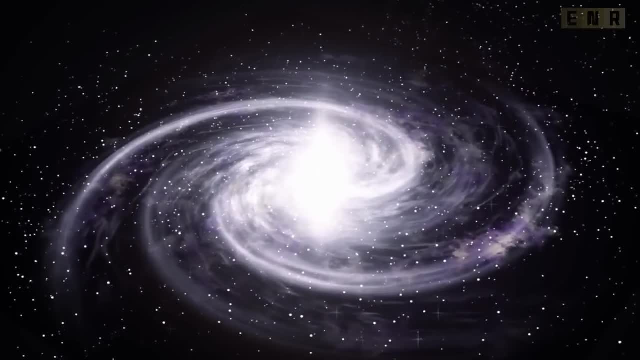 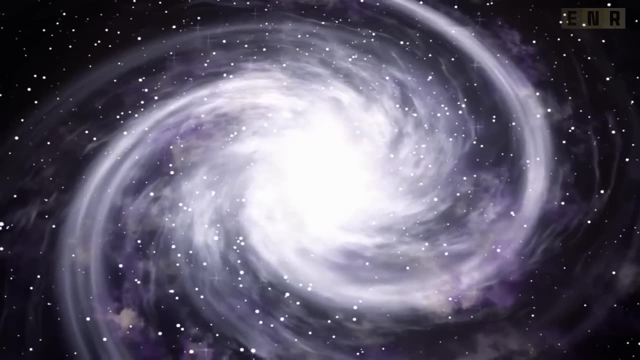 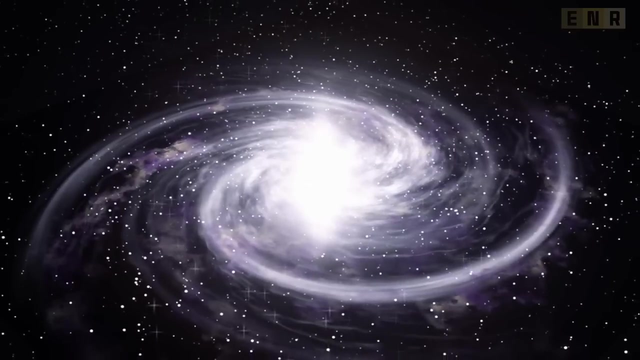 Gravity is what binds the various components together. Over time, it gradually draws stars closer. They pick up speed and flatten out into a disk shape. Massive spiral arms gather stardust and gas. This process was carried out countless times during the course of the cosmos. 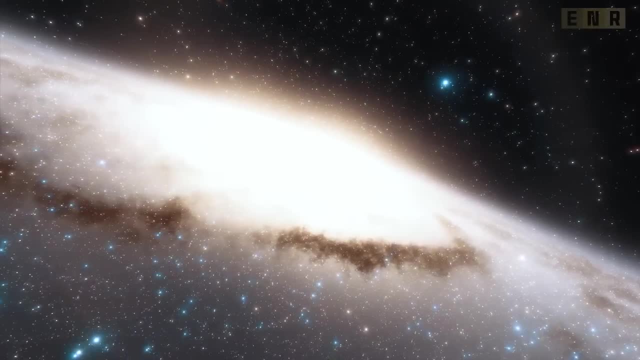 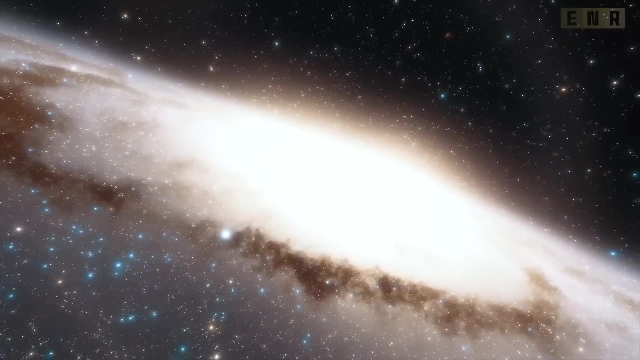 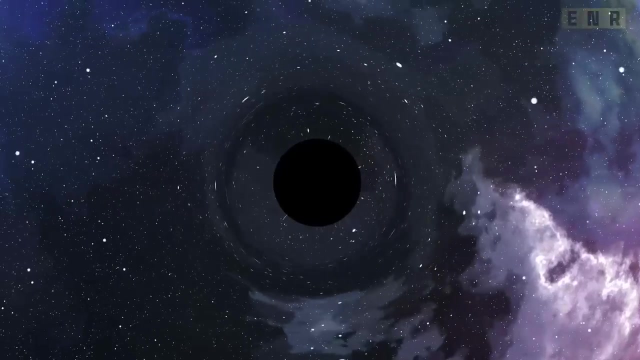 While visually distinct, these galaxies share the fact that they all seem to circle the same central object. For a long time, researchers pondered what might possibly alter a galaxy's behavior, And they found out a black hole, And not just any kind of black hole. 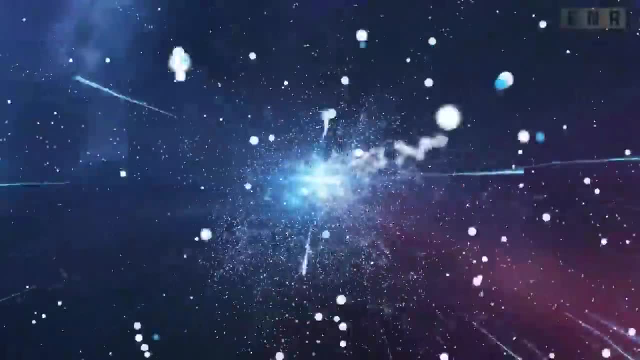 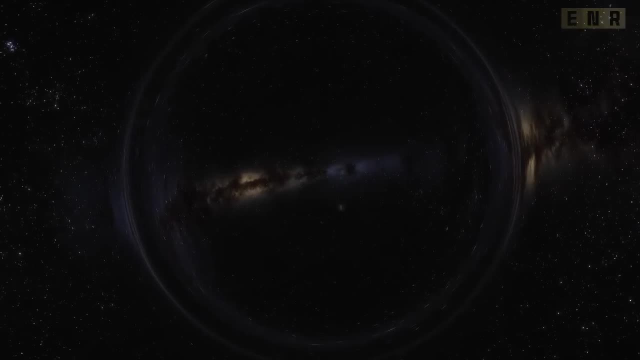 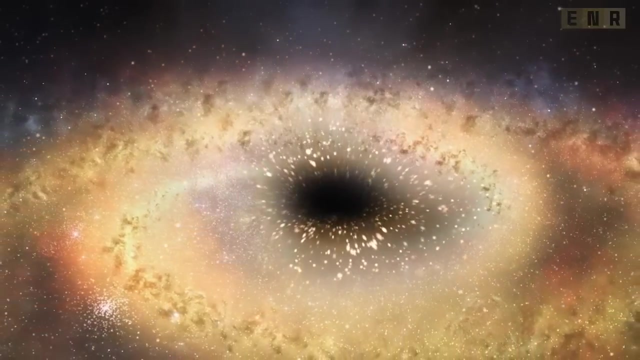 but it's a supermassive black hole. The discovery of extreme amounts of radiation coming from the centers of certain galaxies was the first indication of supermassive black holes. Black holes in these galaxies are eating their surroundings, much like a giant Thanksgiving feast. 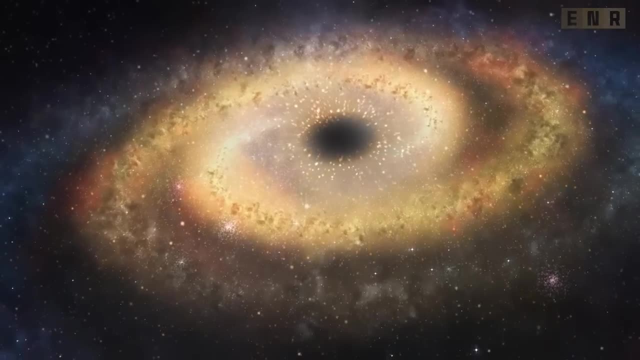 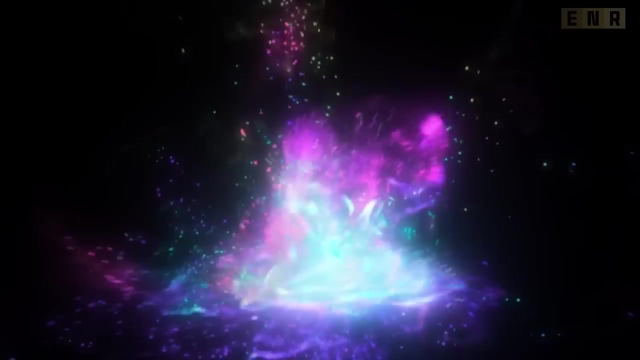 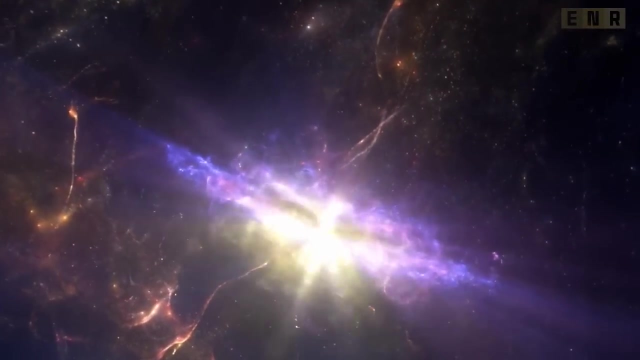 The gas and stars are the supermassive black holes' dinner. Sometimes black holes consume their food so rapidly that they spew it out into space as beams of pure energy. They refer to it as a quasar. The presence of a quasar indicates the presence of a supermassive black hole at the center of the galaxy. 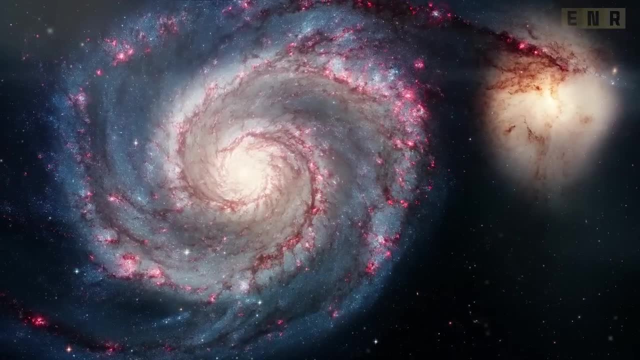 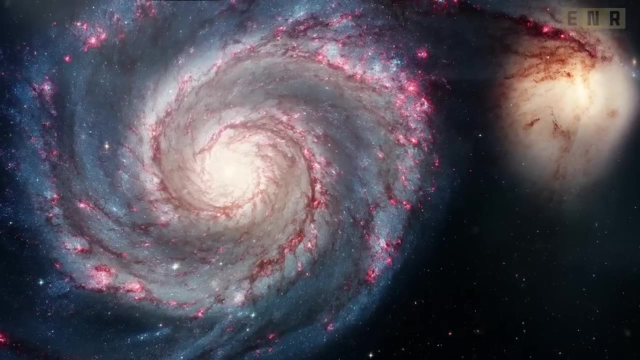 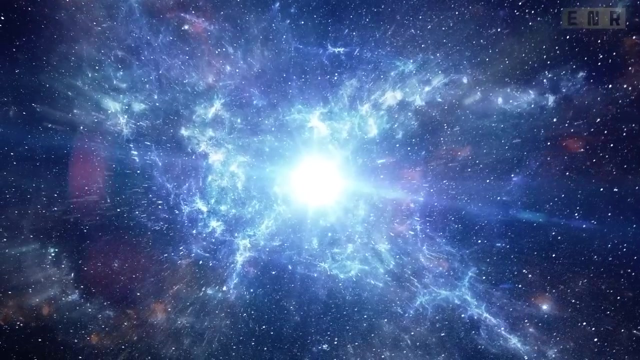 However, what about the Milky Way? There's no quasar here. Does it rule out the existence of a supermassive black hole? Observing the motion of the stars is the key to finding the supermassive black hole in the heart of our Milky Way. 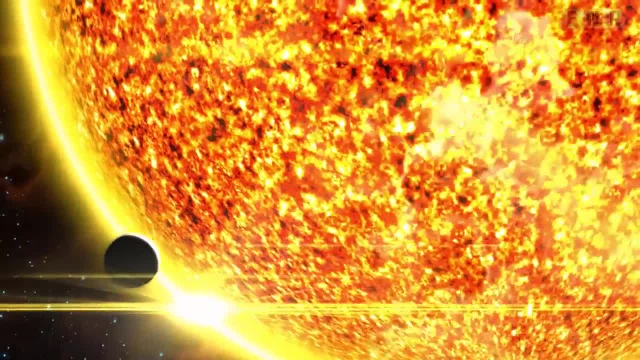 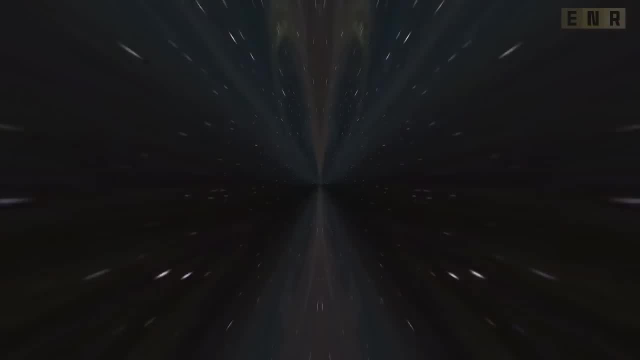 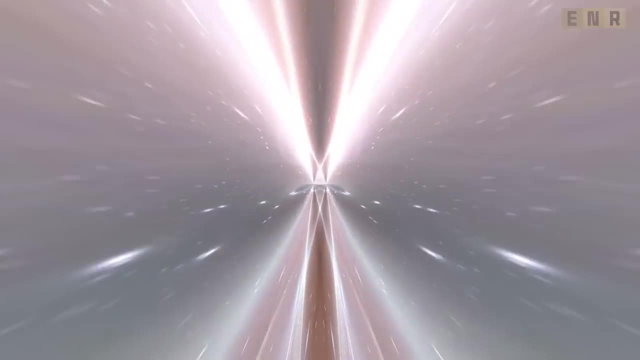 Like the planets that circle the Sun, the stars also move due of gravity. What we discovered was a bizarre and violent environment At the center of our galaxy. everything is more extreme. Things move very quickly. The stars will be passing one another at high speeds. 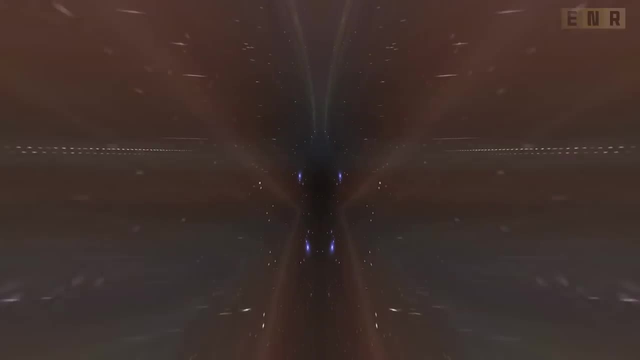 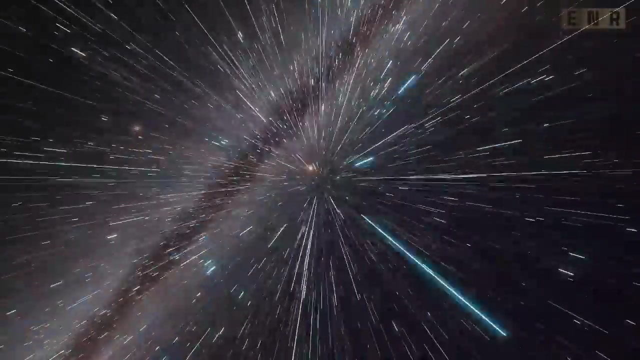 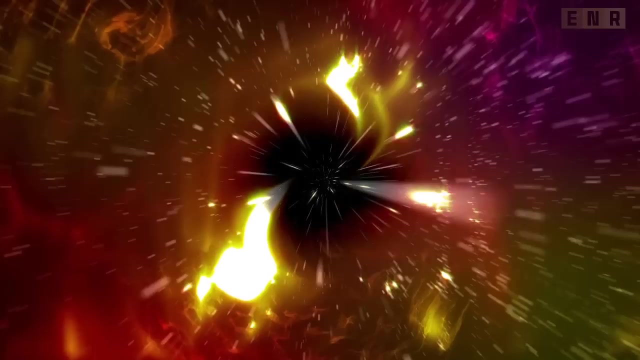 It is unlike any other place in the universe. The photographs of the stars in orbit showed a remarkable phenomenon. They had to have been traveling at a million miles per hour or more. Only a gigantic black hole has the energy to toss large stars around like that. 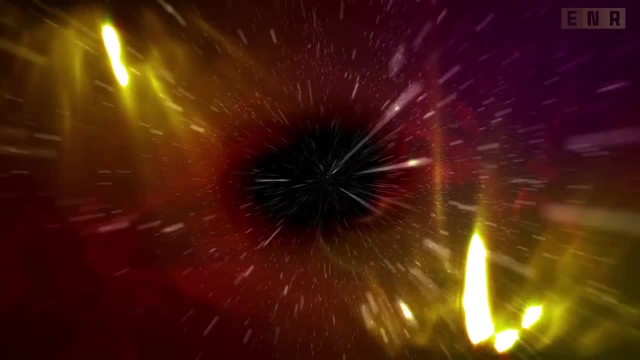 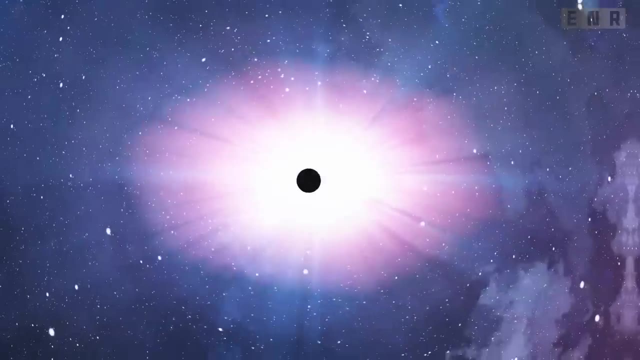 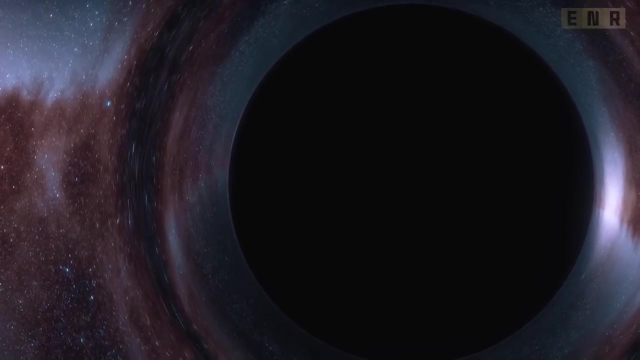 This curvature was the conclusive evidence for a supermassive black hole at the heart of our galaxy. As it is the black hole's gravity that drives the orbits of these stars, A massive black hole measuring 15 million miles wide sits at the heart of our Milky Way galaxy. 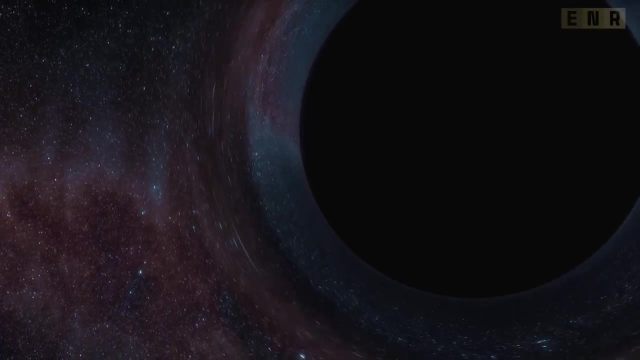 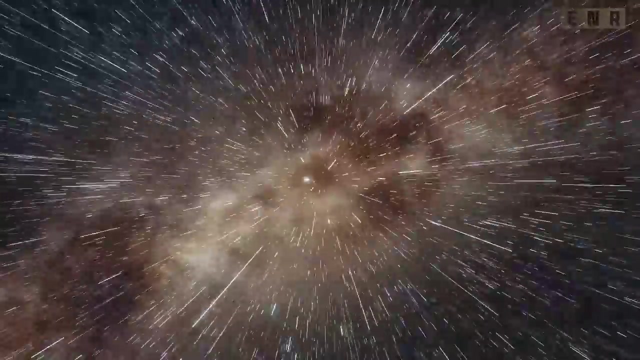 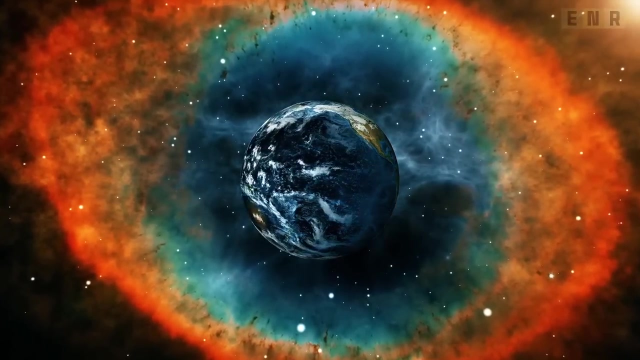 So is there any danger to Earth? We are in absolutely no danger of being sucked into our supermassive black hole. It's simply too far away. In reality, the distance between Earth and the supermassive black hole in the heart of the Milky Way galaxy is 25,000 light-years. 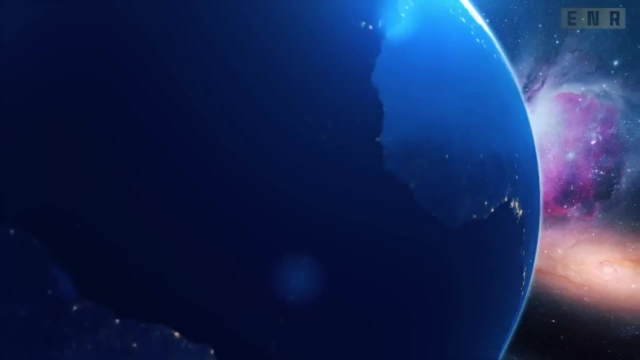 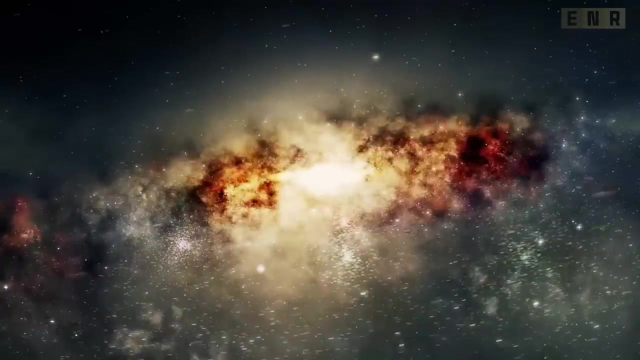 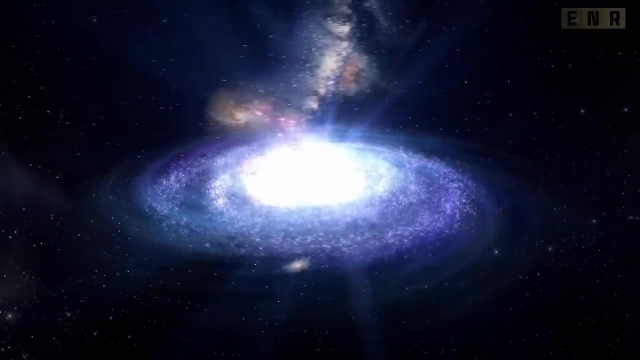 That's many trillions of miles. For the time being, Earth is secure. Although supermassive black holes are the source of enormous quantities of gravity, they are not strong enough to bind galaxies together. In reality, the rules of physics dictate that galaxies should accelerate away from one another. 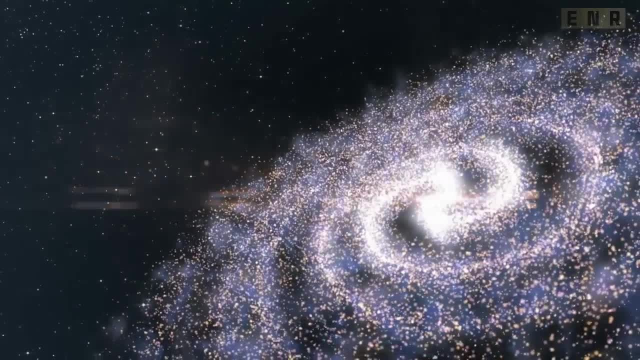 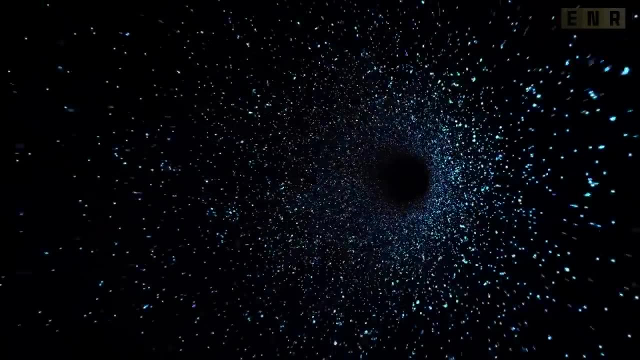 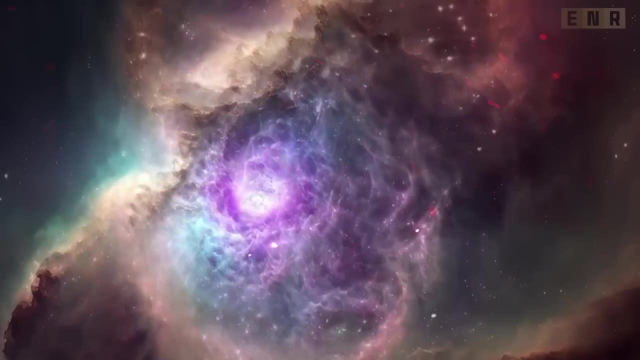 So what's stopping them? Because there's something stronger than a gigantic black hole waiting to be discovered. It is invisible and very difficult to detect. It's called dark matter and it's everywhere. Supermassive black holes discovered by astronomers are found in the centers of galaxies. 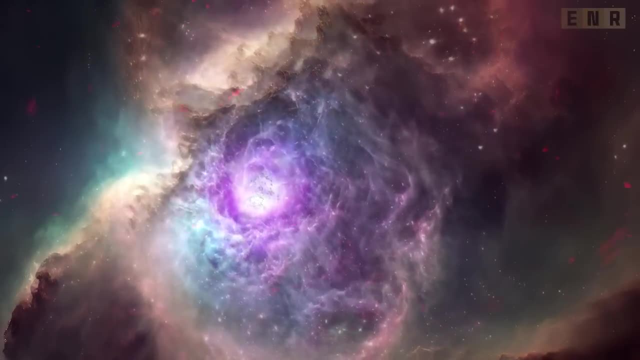 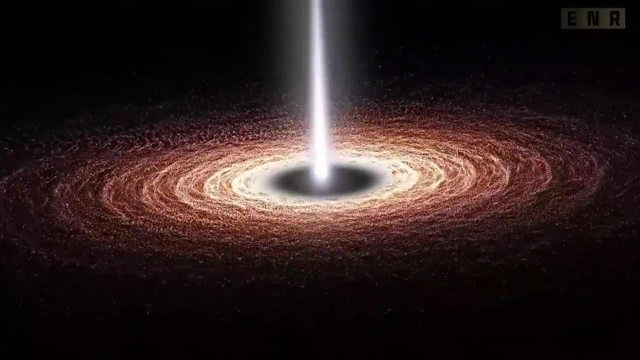 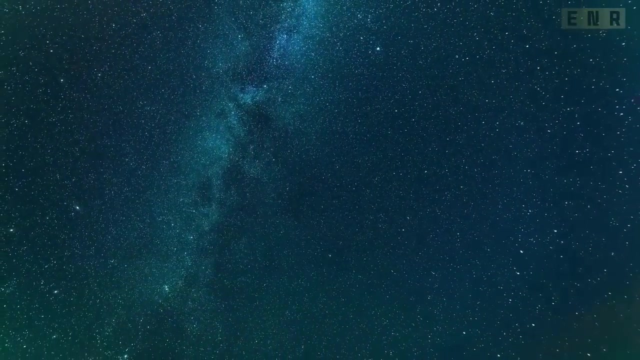 and are responsible for the rapid movement of stars in their vicinity. However, they are insufficient to hold together all of the stars in a vast galaxy. So what does hold them together? It was a mystery until a maverick scientist proposed that something unknown was in action. 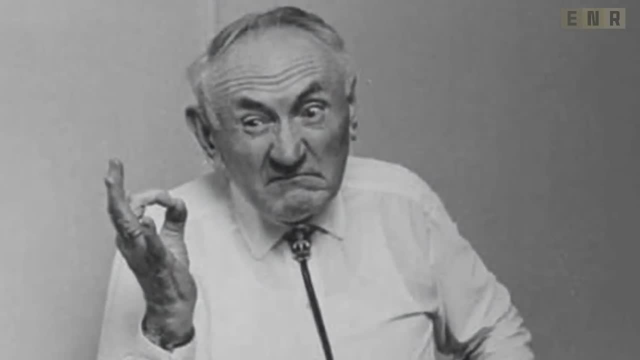 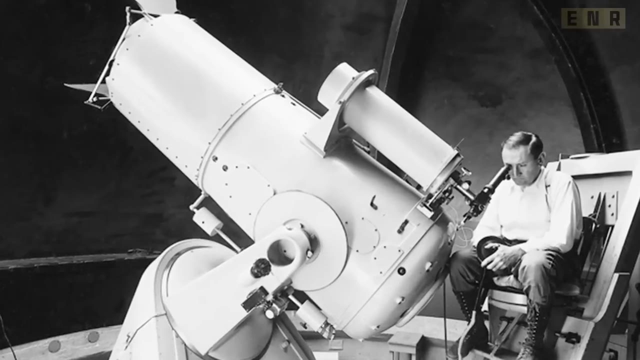 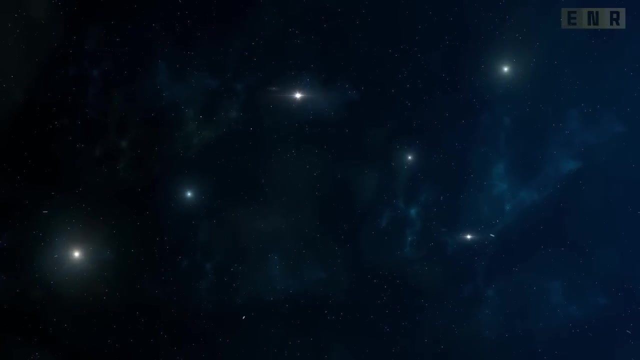 Fritz Zwicky, a Swiss astronomer, pondered in the 1930s why galaxies clustered together. He reasoned that because they weren't producing enough gravity, they should be flying apart. However, the force of our own gravity was insufficient. Therefore, he deduced that it must be something that had never been discovered before. 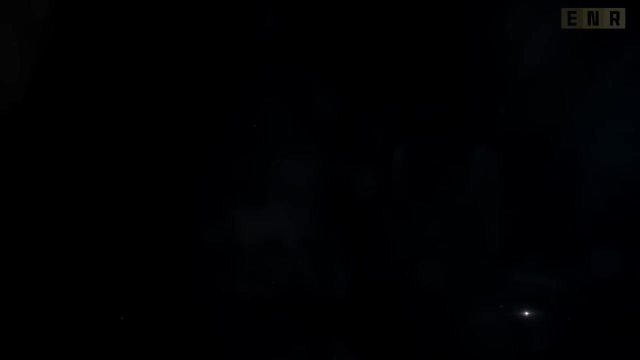 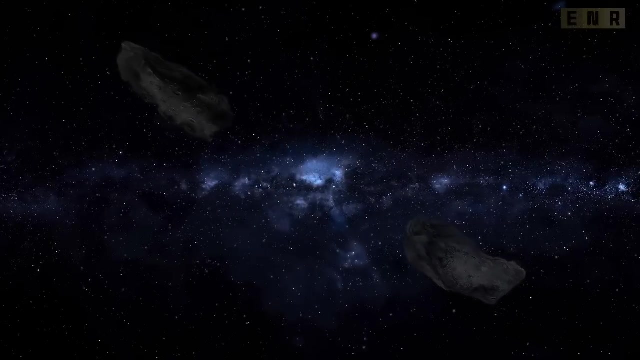 something that had never even been considered, and he called it dark matter. Fritz Zwicky was decades ahead of his time and that's why he graded on the astronomical community, And this is a brilliant idea. But he was correct, you know. 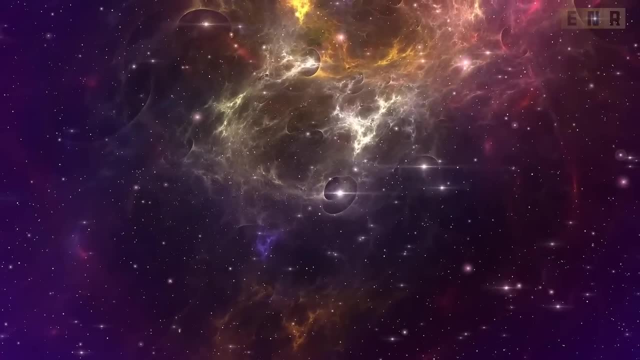 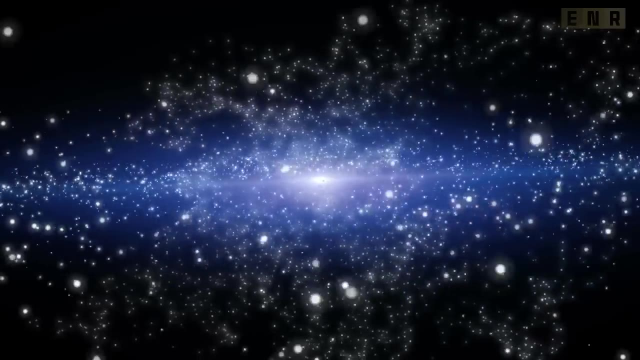 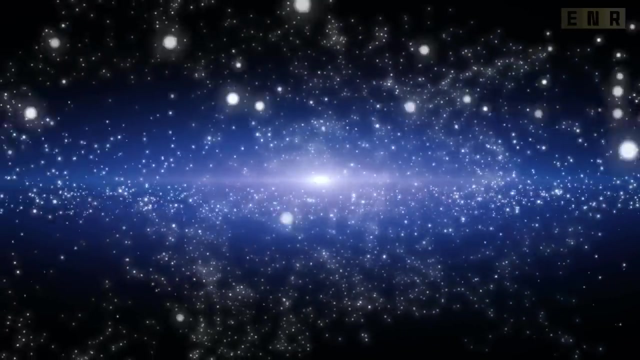 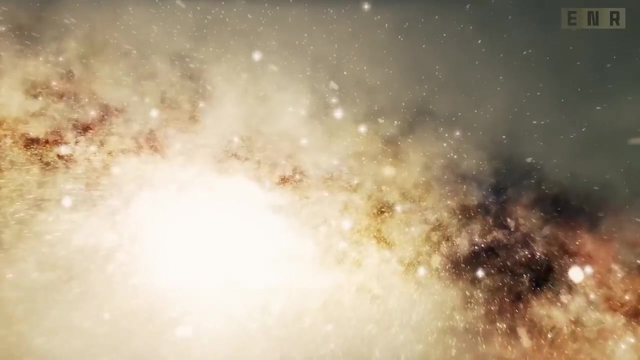 It's possible that individual galaxies are also held together by the mysterious substance that Zwicky dubbed dark matter. Galaxies rely on dark matter as a kind of protective framework that keeps them from collapsing and moving about. Now scientists have discovered that dark matter does more than just bind galaxies together. 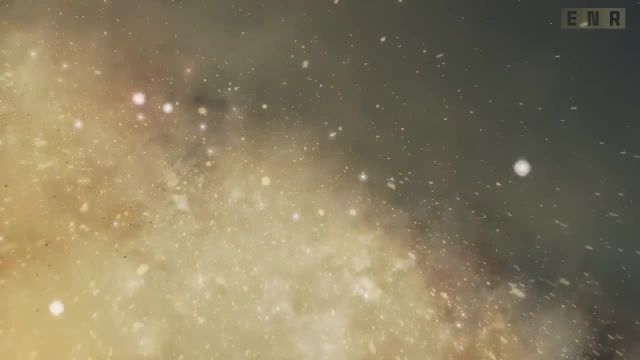 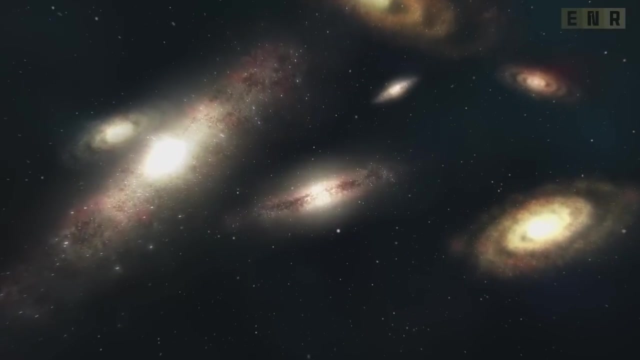 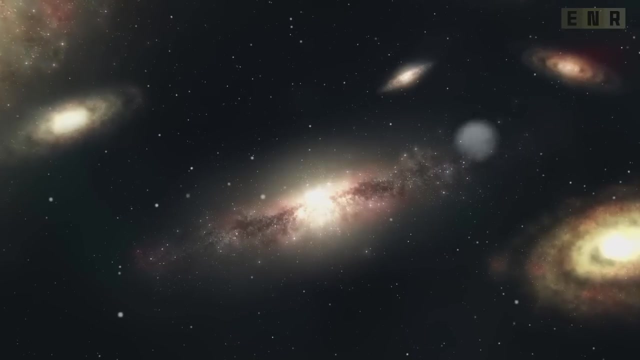 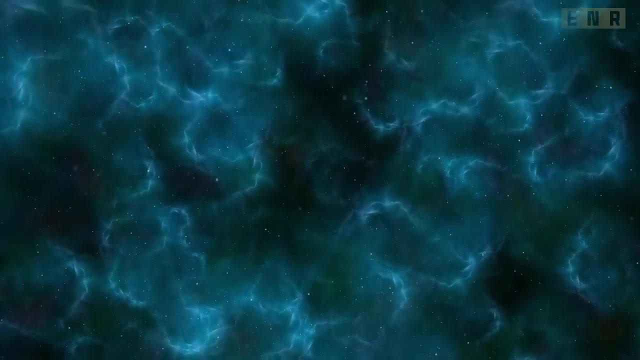 It may have also triggered their evolution. Scientists believe that after the Big Bang, dark matter started to cluster and these dark matter clumps evolved into the galaxy's nucleus. However, the nature of dark matter is still a mystery to physicists. Weird things happen with dark matter. since we don't know what it is. 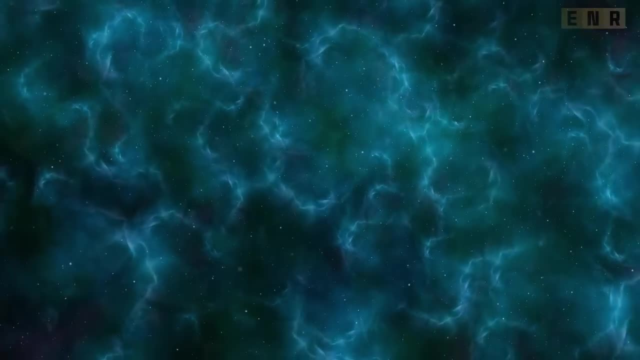 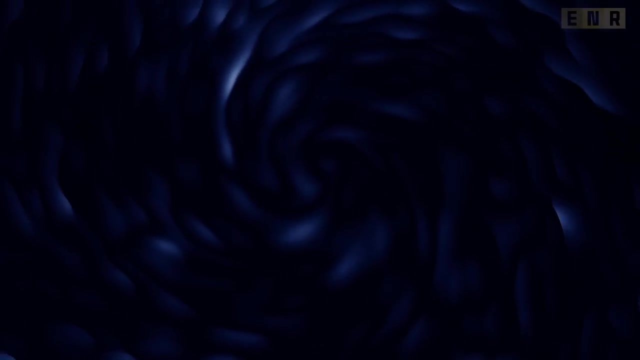 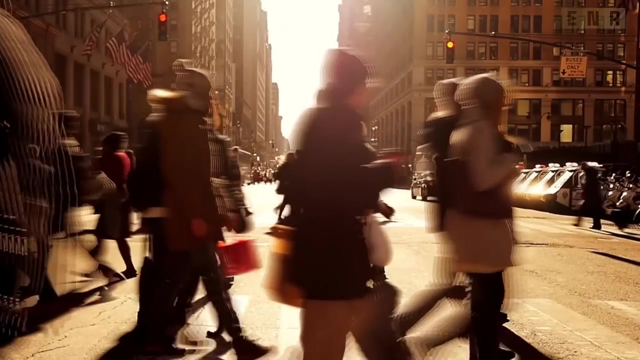 Obviously, it's not constructed from the same substance that humans are. You can't push against it, You can't feel it. However, it is likely everywhere. It's a ghost-like material that will pass right through you as if you didn't exist at all. 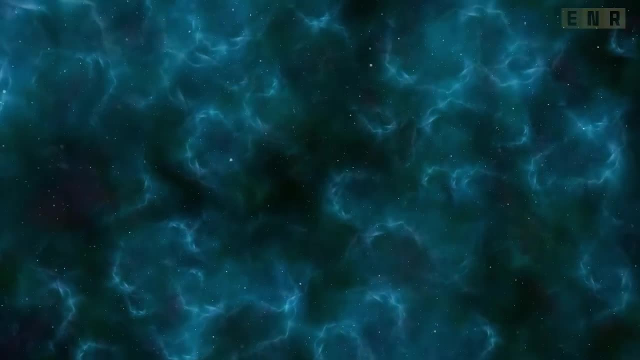 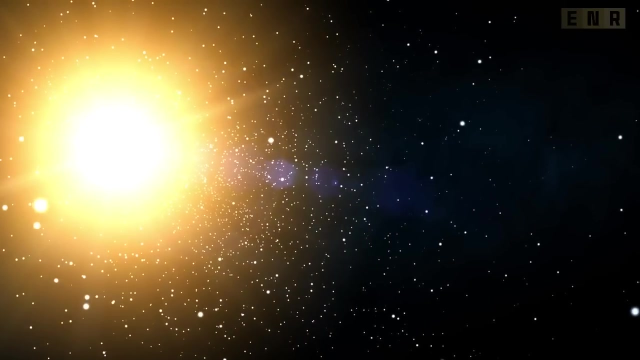 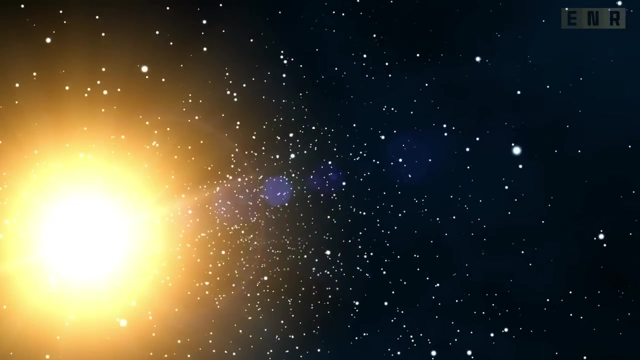 Although our understanding of dark matter is limited, it seems to be abundant across the cosmos. That means there must be at least six times as much dark matter as regular matter what humans are comprised of in the cosmos, And the way the cosmos seems to function depends on it. 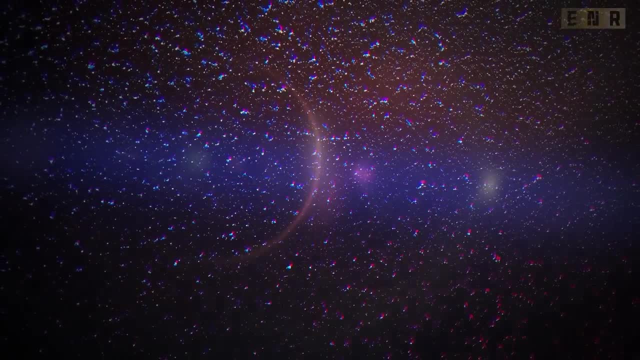 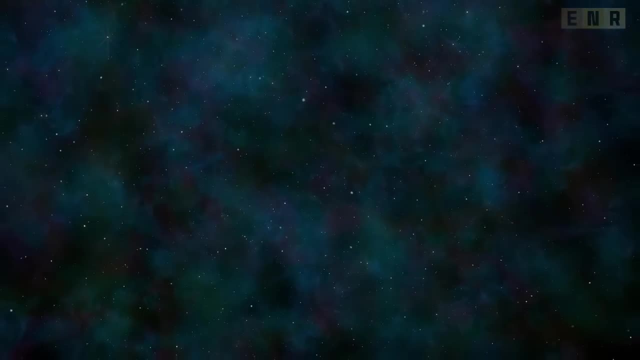 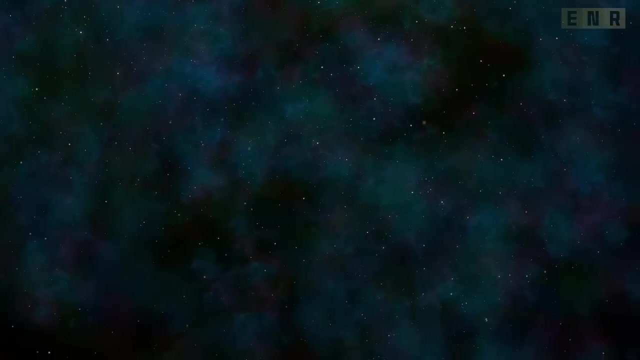 Observations of its effects on light have led to its recent indirect detection in deep space. Through a process known as gravitational lensing, it warps the light. The existence of dark matter may be tested using gravitational lensing, As a ray of light from a distant galaxy travels towards us. 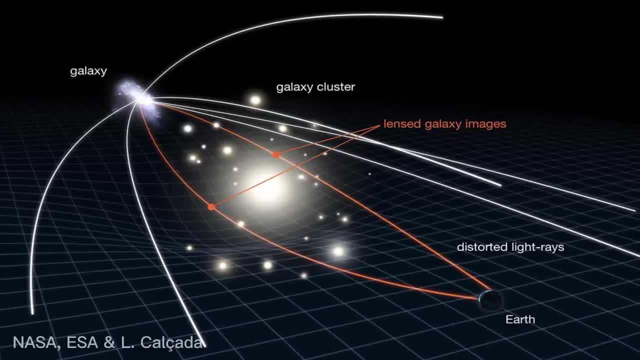 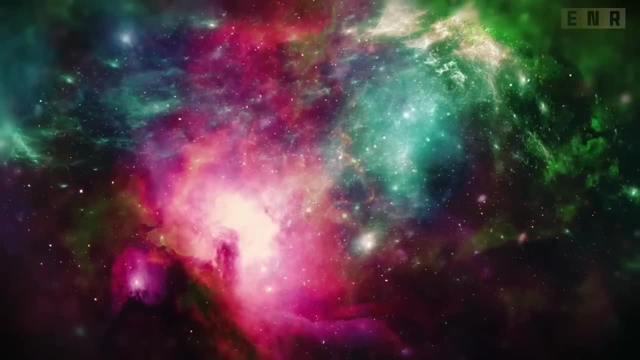 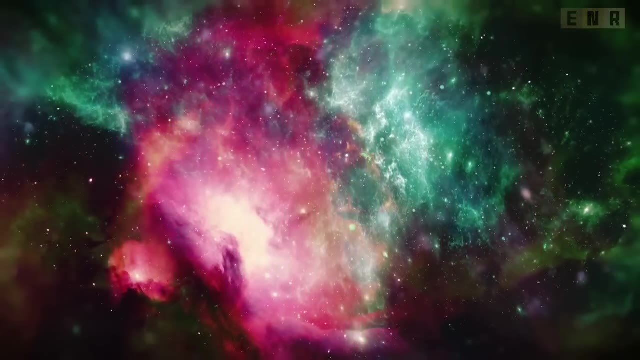 its course will be bent around a huge collection of dark matter. due to the latter's greater gravitational attraction, Some distant galaxies indeed seem stretched and warped when seen via the Hubble telescope. The picture distortion is due to the presence of dark matter. We can determine the density of dark matter. 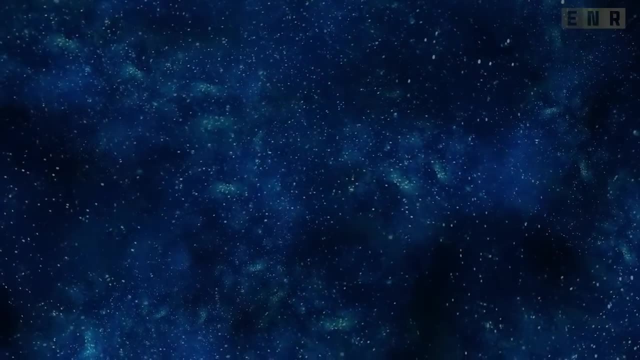 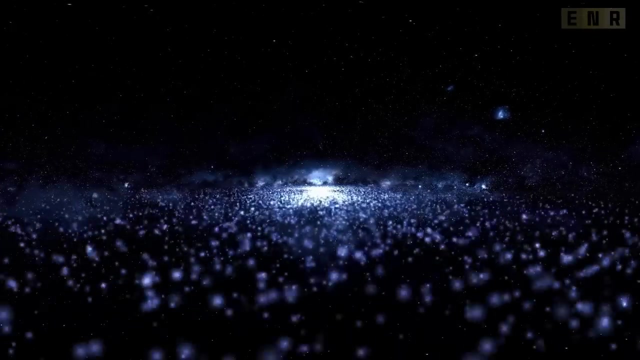 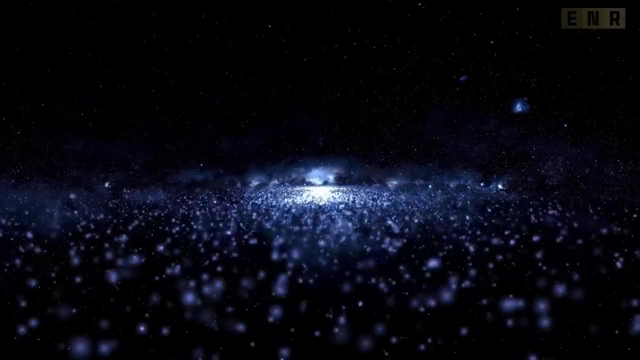 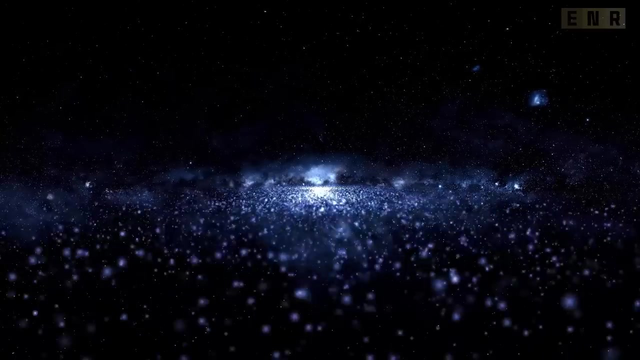 by carefully examining the forms and degrees of distortion of these galaxies. Now more than ever, the importance of dark matter to the cosmos is undeniable. It's what makes galaxies form and stops them from collapsing. Even though it's invisible and undetectable, dark matter rules the cosmos. 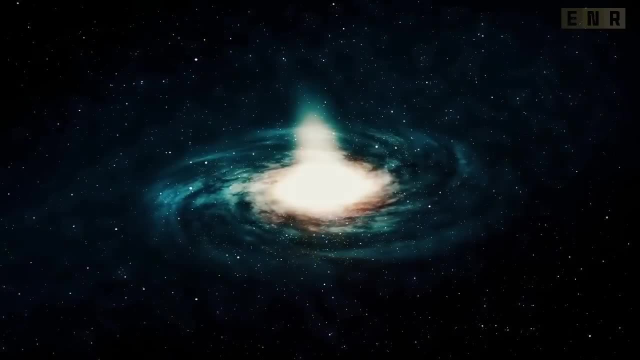 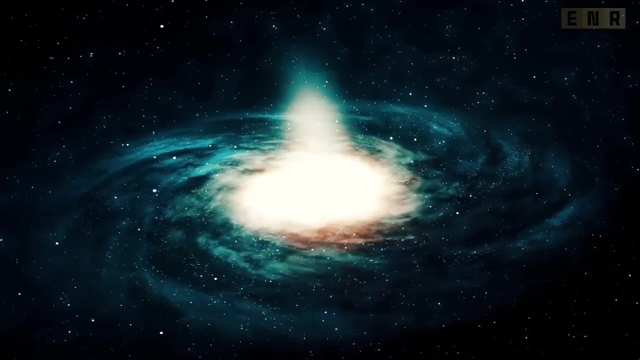 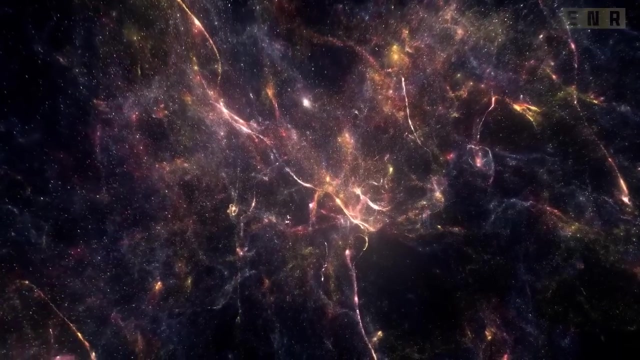 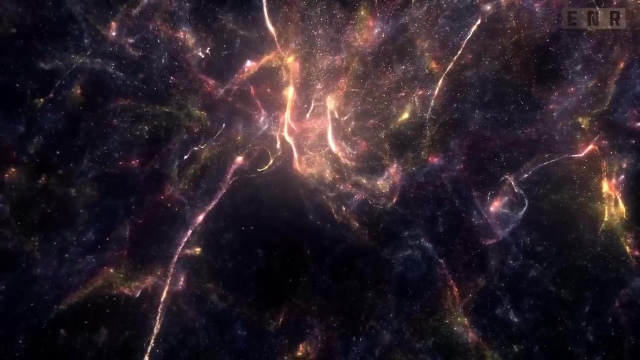 These galaxies seem to be completely alone. It's true, they are trillions of miles apart, But actually they live in groups called clusters, And these clusters of galaxies are linked together in superclusters containing tens of thousands of galaxies. The Milky Way's place in the cosmos remains a mystery. 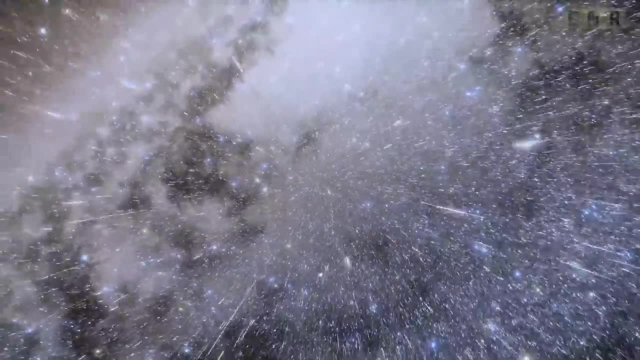 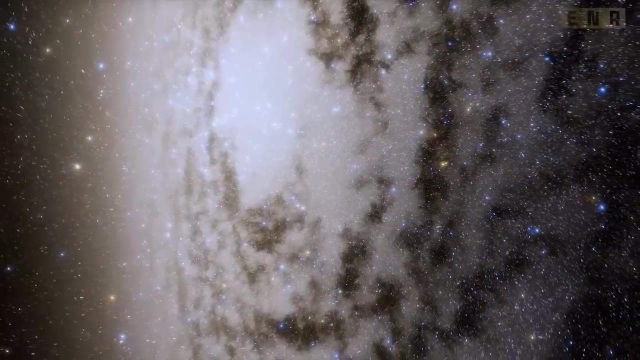 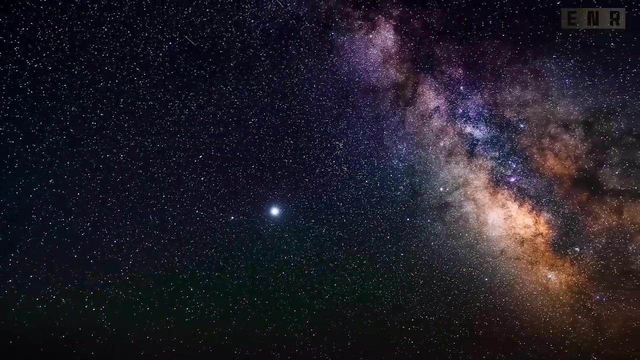 If you look at the overall image, you'll see that our galaxy is associated with a smaller group of galaxies, including about 30 members in total, and that our galaxy and Andromeda are the two largest members of this group. Further observation reveals, however. 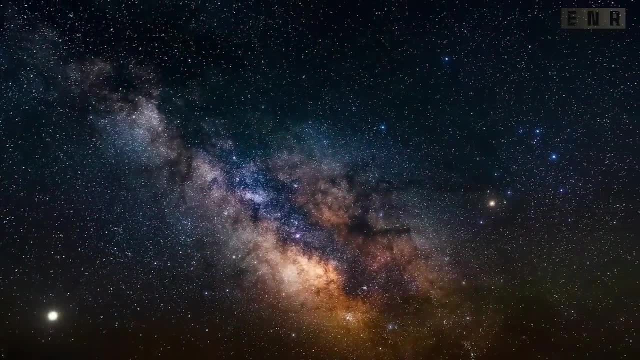 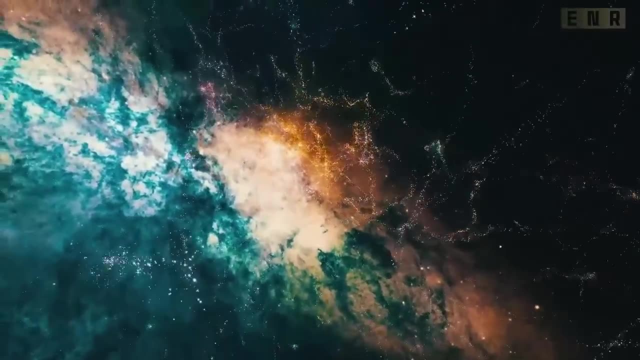 that our galaxy is embedded inside the Virgo supercluster. Researchers are now making maps of galaxy clusters and superclusters to better understand the causes. This is the first time we've seen a galaxy cluster in the cosmos. Galaxies are the immense star empires. 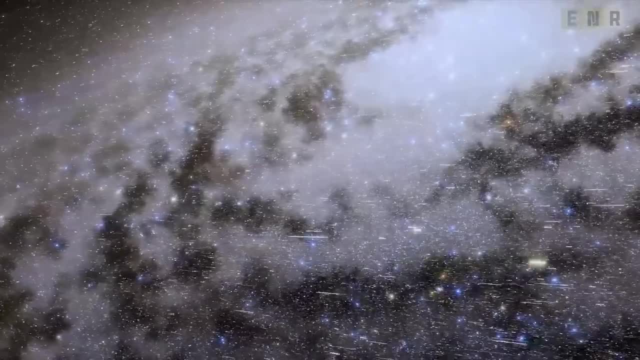 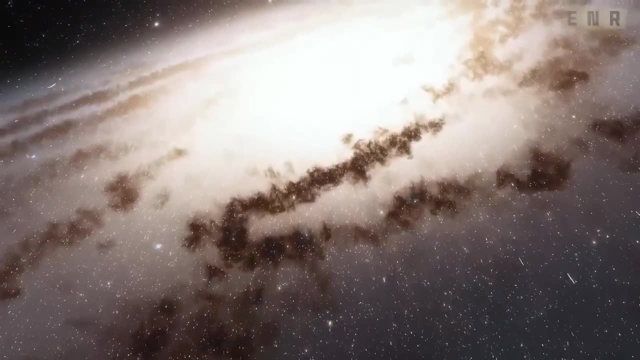 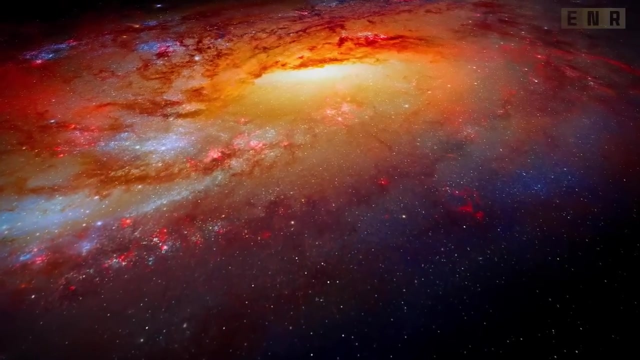 The shapes range from enormous balls to intricate spirals. The problem is that they are always evolving. When we stare out into the cosmos, it's easy to assume that our galaxy hasn't changed in eons. It's not. The Milky Way is a dynamic galaxy. 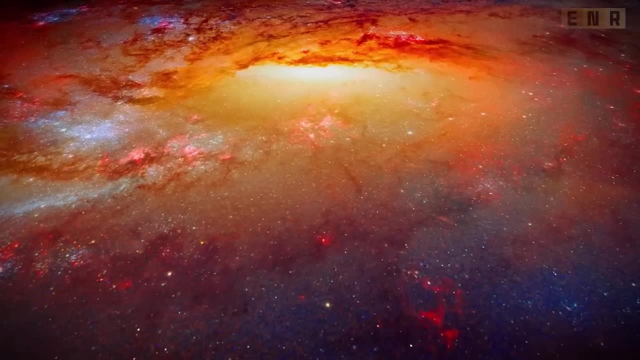 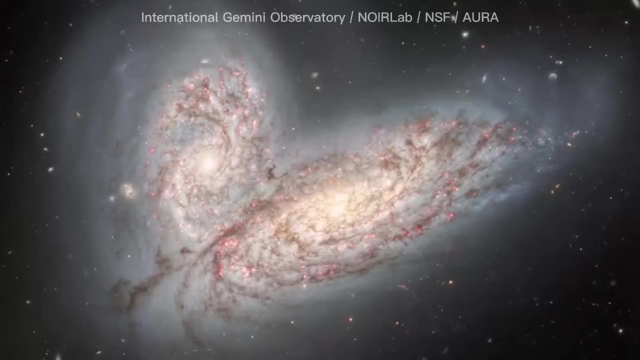 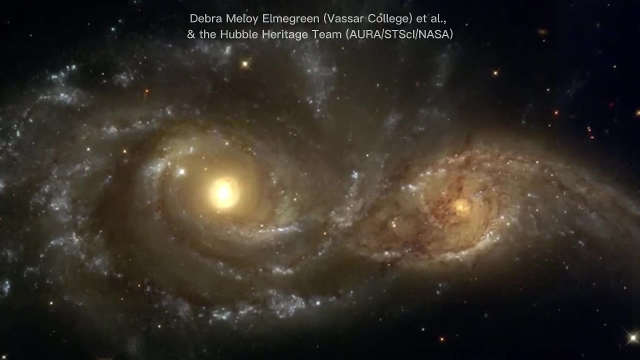 Over cosmic eons, its basic nature has been changing. Galaxies don't only evolve, they move as well, And sometimes they run into each other. The two galaxies will merge over millions of years when they collide. This kind of collision occurs all the time in the cosmos. 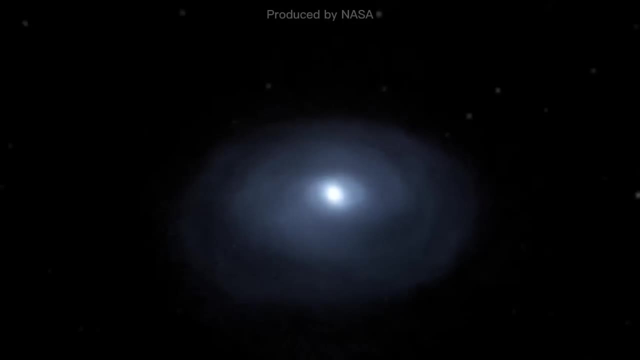 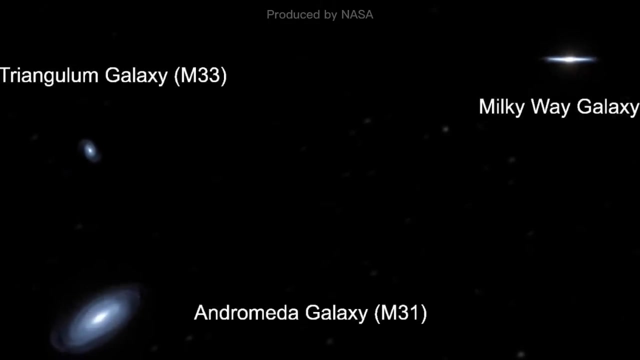 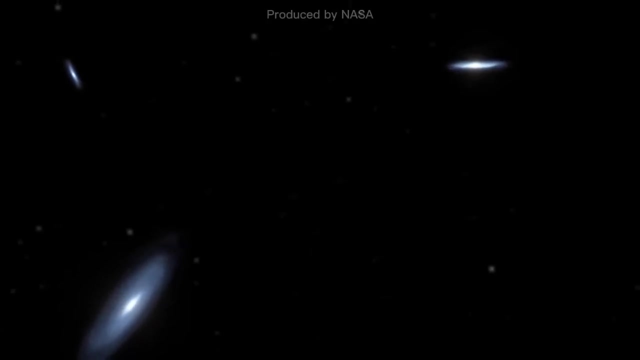 Our own Milky Way is no exception. We are on a collision course with the galaxy Andromeda, And that's terrible news for the Milky Way. At a speed of around a quarter of a million miles per hour, our Milky Way galaxy will collide with Andromeda in about 5 billion to 6 billion years. 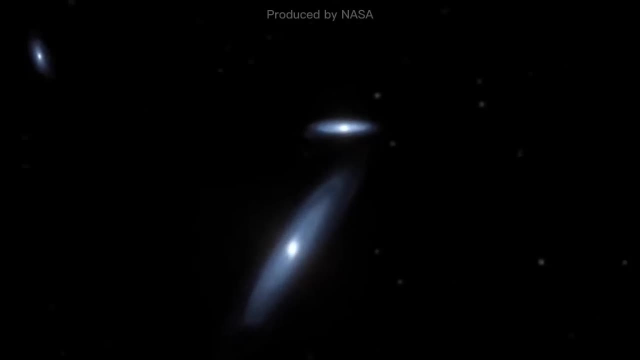 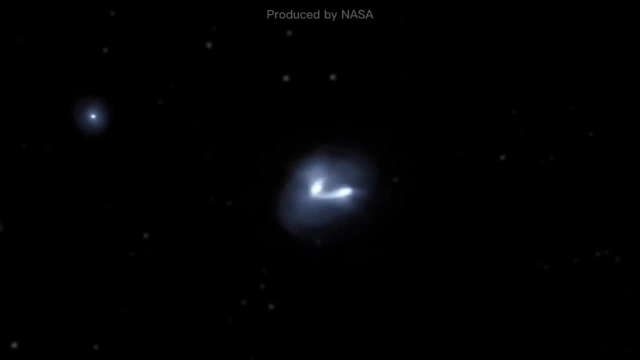 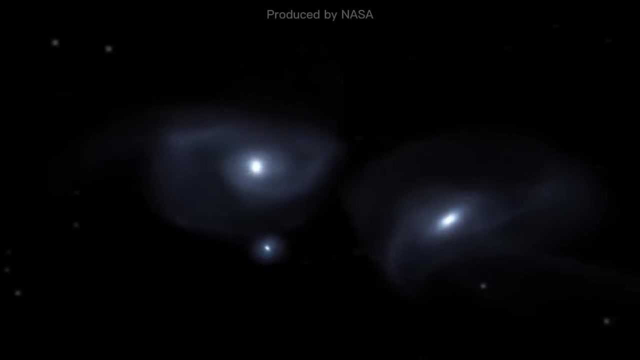 It's all over for the Milky Way galaxy. If you could look out into space, you'd see the whole Andromeda galaxy hurtling toward us at a tremendous rate of speed. As the two galaxies interact, they both become more and more disturbed and closer and closer together. 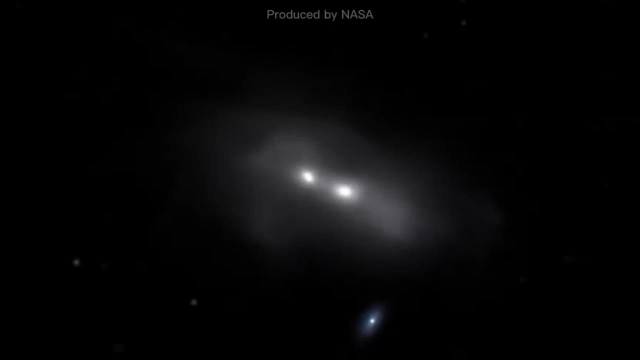 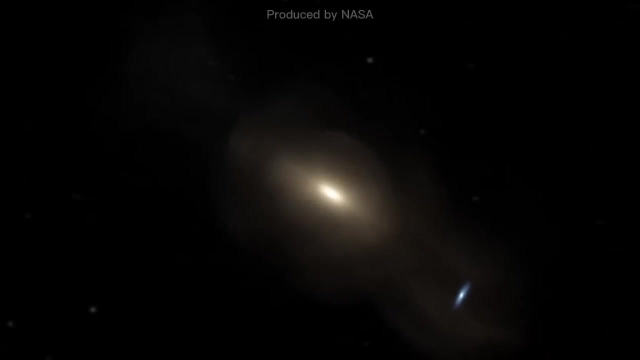 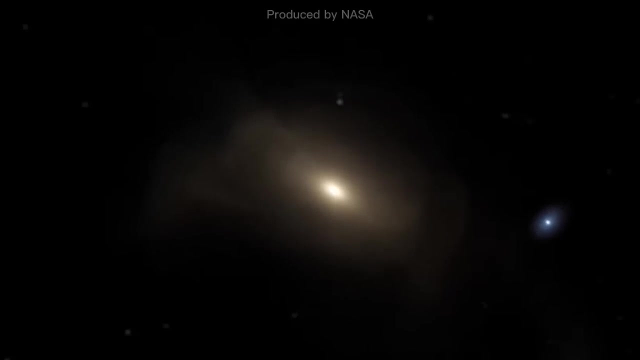 There will be a dance of death between the two galaxies. Whenever galaxies collide, they release clouds of gas and dust in all directions. As galaxies collide, their combined gravity rips stars from their orbits and launches them into the void. As we approach doomsday for the Milky Way galaxy, it would be spectacular. 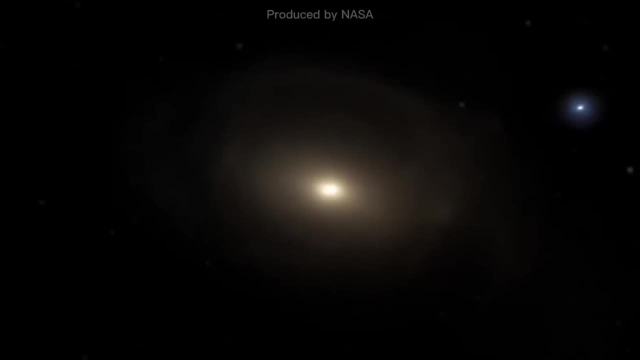 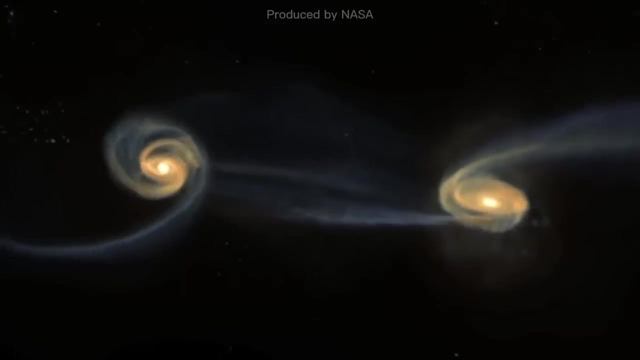 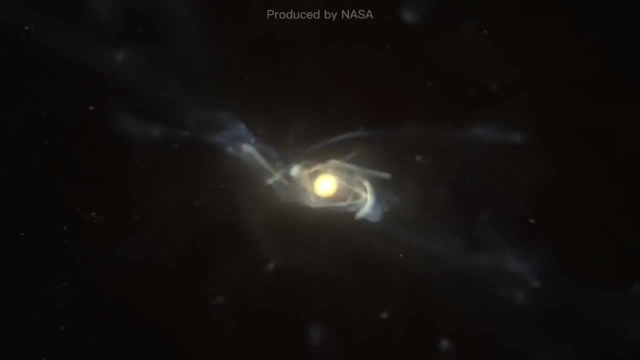 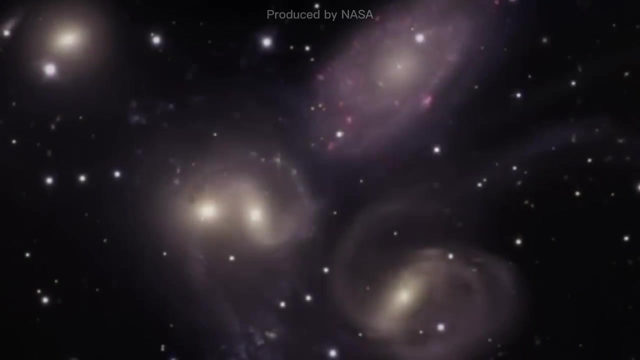 The two galaxies will ultimately pass through one another and merge into a single one: The Milky Way and Andromeda. as we know it will cease to exist and Milkomeda will be born, and it will look like a whole new galaxy. There's no escaping what's going to happen. 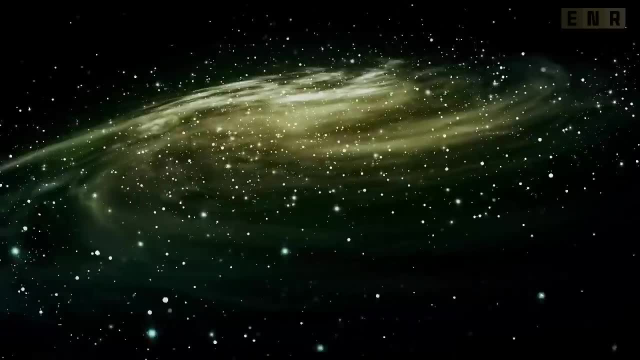 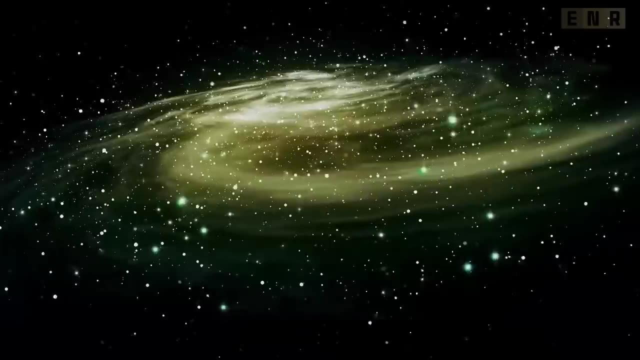 The question is: what's it mean for planet Earth? We may either be thrown out into outer space when the arms of the Milky Way galaxy are ripped apart, or we could wind up in the stomach of this new galaxy. Stars and planets will be pushed all over the place. 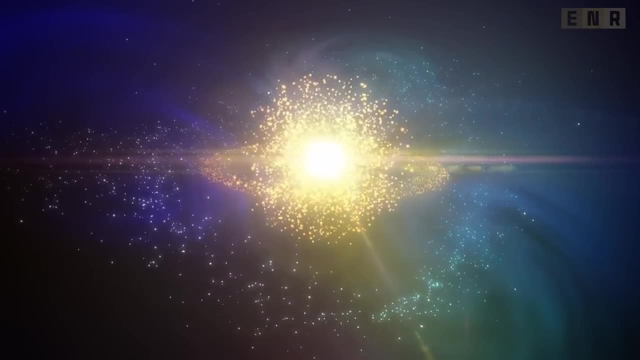 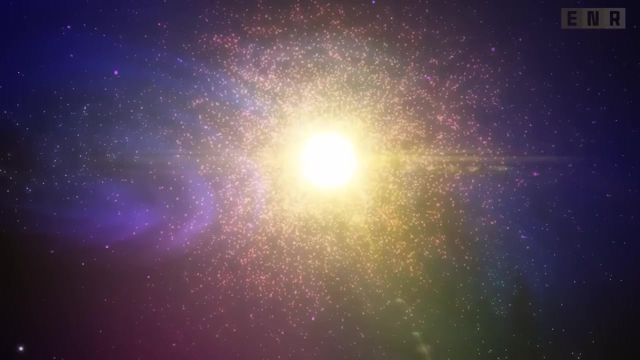 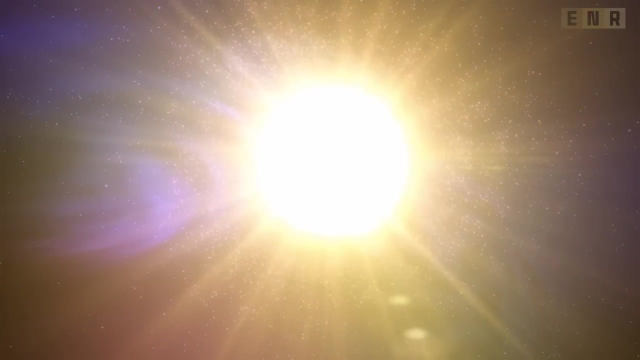 so this may well be the end of planet Earth. Galaxies all over the universe will continue to collide, But this age of galactic cannibalism will eventually pass, Because there is an even more destructive force in the universe, a force that nothing can stop. 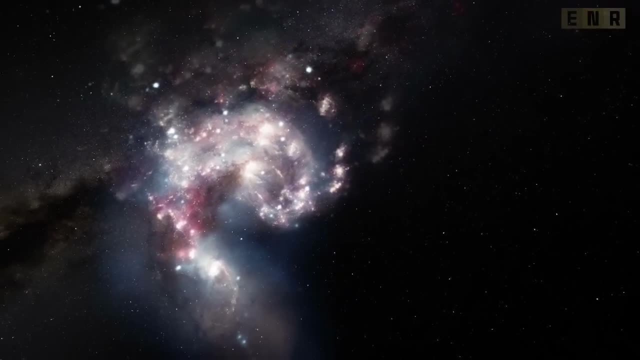 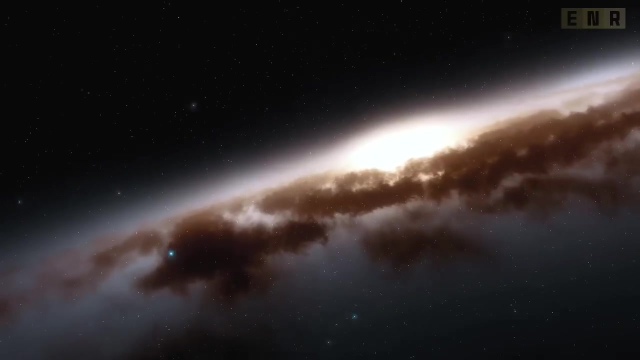 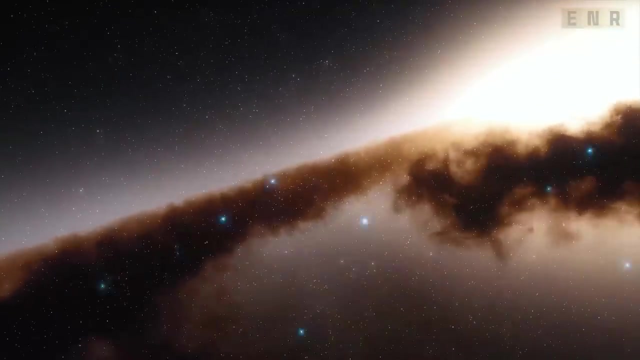 It will eventually tear the cosmos apart by stretching everything to the point that galaxies are pushed apart from one another. Researchers have identified a new cosmic power. It's called dark energy. Unlike dark matter, dark energy has the opposite effect: It pushes galaxies apart rather than bringing them together. 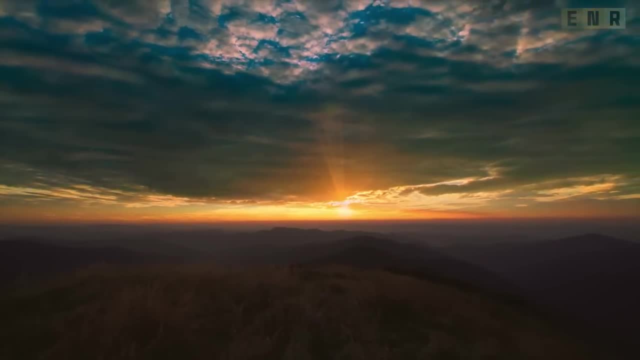 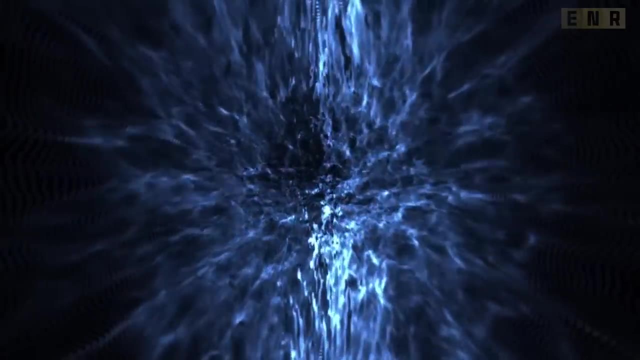 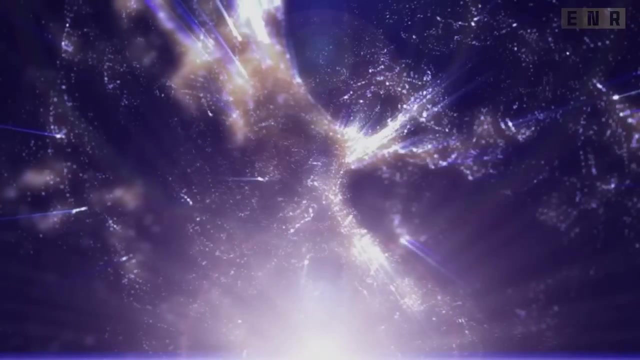 Dark energy, which we've only discovered in the last decade and which dominates the universe, is significantly more enigmatic. We don't have the slightest idea why it's there. What it's made from, we don't really know. We are aware of its presence, but beyond that, 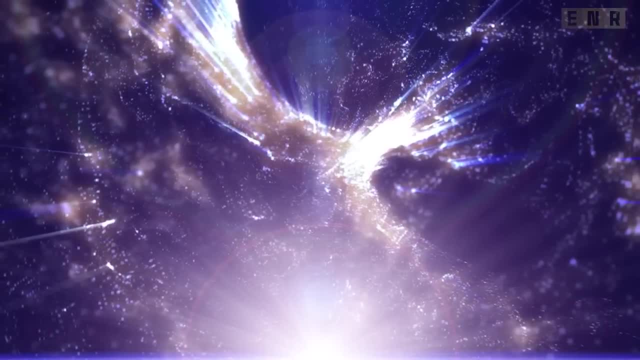 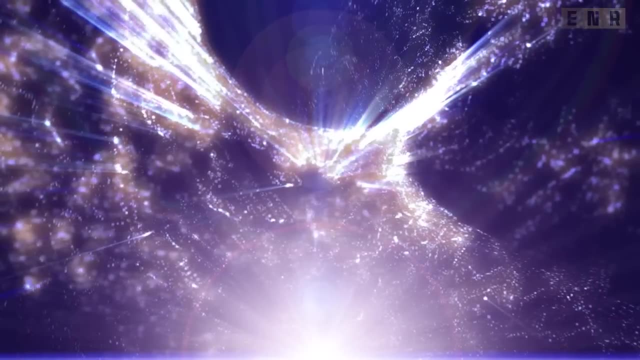 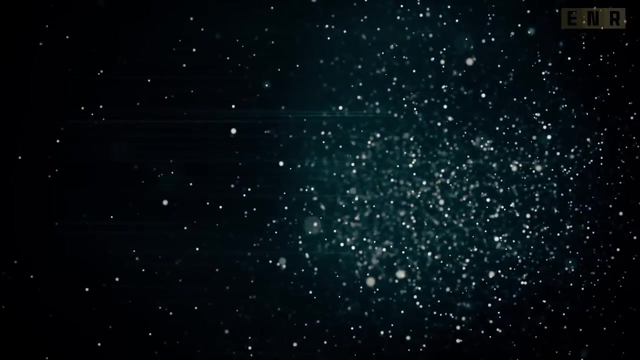 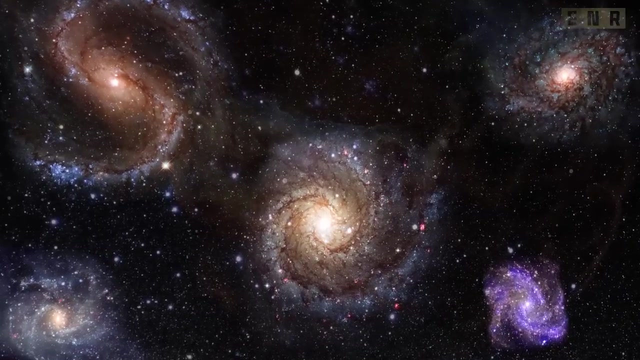 our understanding of it is limited. Dark energy is really weird. Things resist and are pushed away from one another, as if space itself contained tiny springs. In the far future, scientists predict that dark energy will triumph over dark matter in the cosmos And with that triumph, galaxies will finally begin to drift apart. 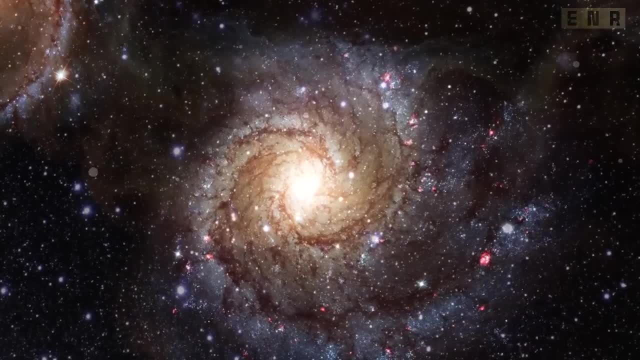 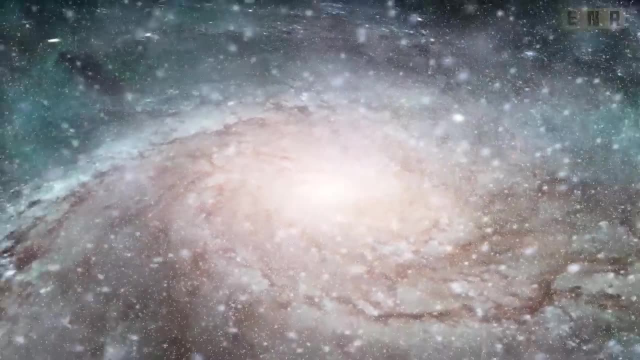 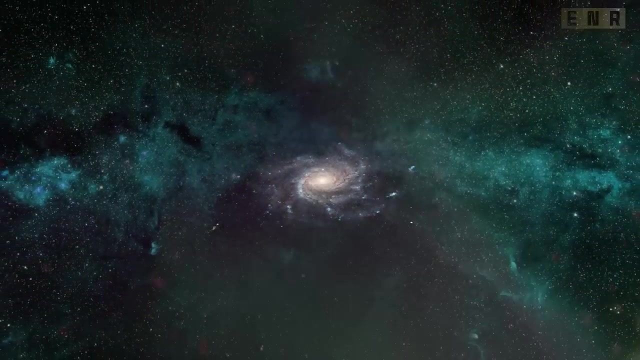 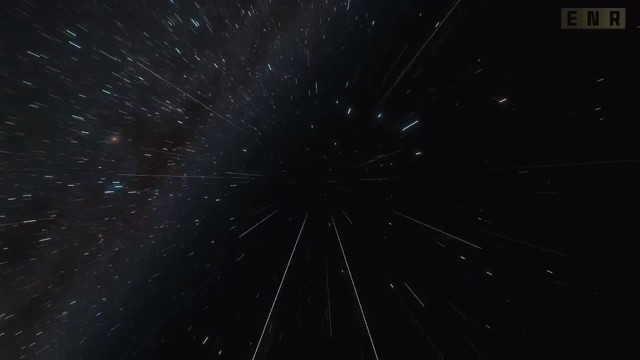 Galaxies will eventually die off due to dark energy. It will do this by accelerating the expansion of the universe, forcing all galaxies to recede farther and further away from us, until they become invisible and travel faster than the speed of light. Therefore, everything else in the cosmos will vanish before our own eyes. 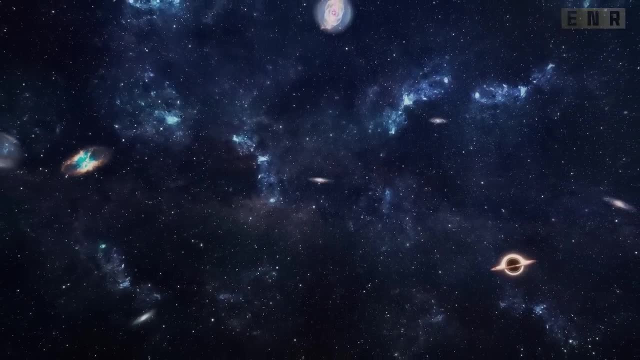 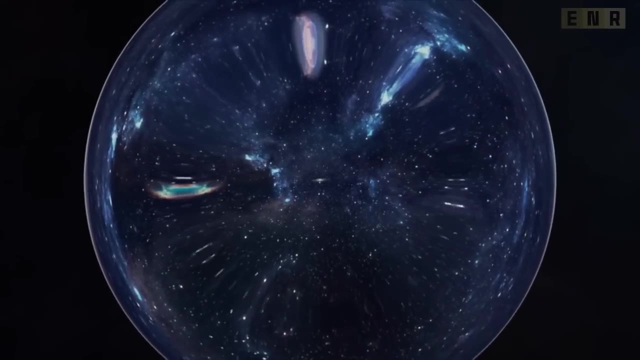 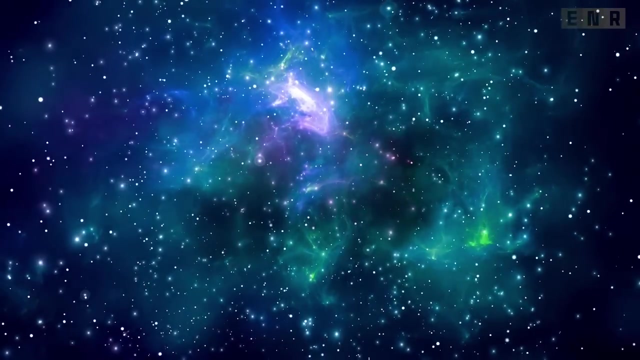 The remainder of the cosmos won't vanish today or tomorrow, but it may after a trillion years. Galaxies will be left alone in the void. However, this will not occur for an extremely lengthy period. The cosmos is doing well right now and galaxies are creating favorable circumstances for life to exist. 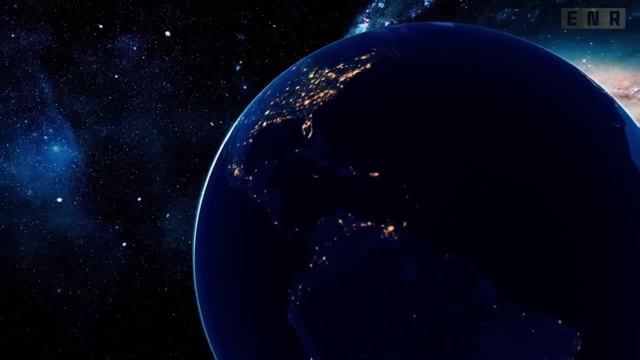 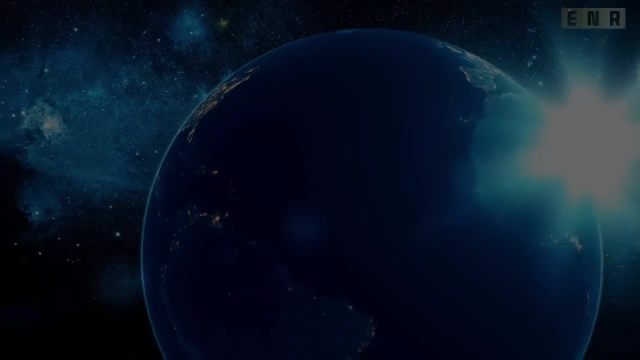 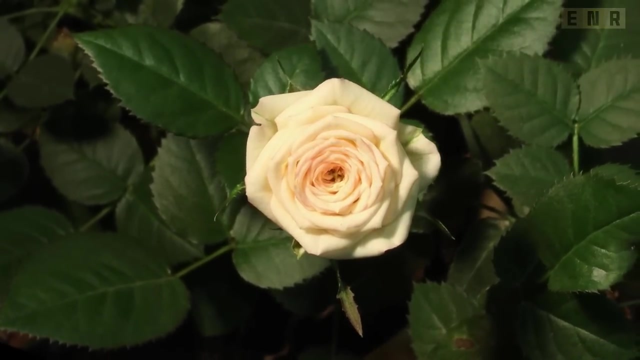 Without galaxies, I wouldn't be here, You wouldn't be here. Maybe not even life itself would exist. This is unfortunate for us. The only reason why life has evolved on Earth is because our minuscule solar system was formed in the correct region of the galaxy. 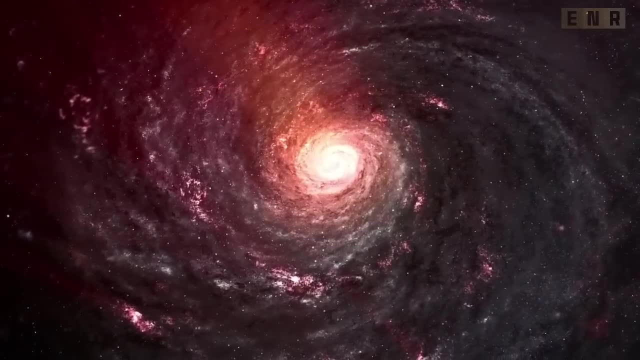 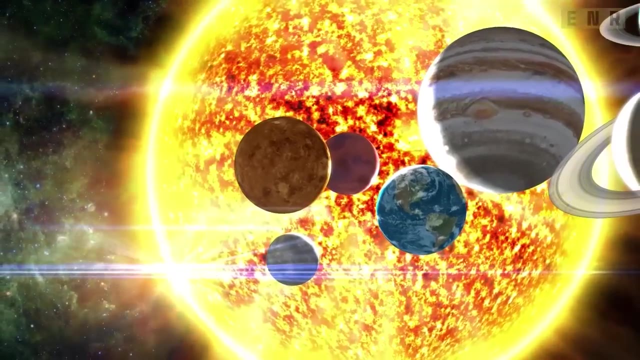 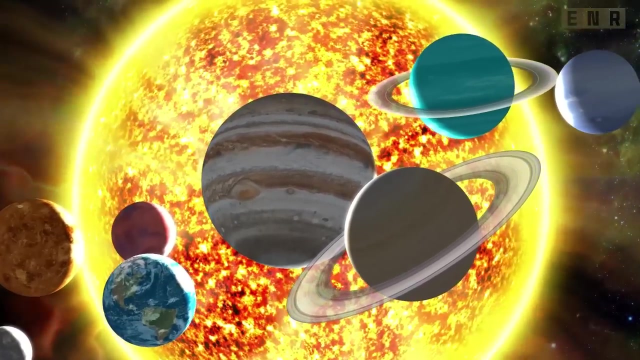 If we were any closer to the center, we wouldn't be here. Life in the center of a galaxy may be extremely hazardous. In point of fact, the proximity of our solar system to the core of our galaxy would render it so radioactive that it would be impossible for life to continue in any form. 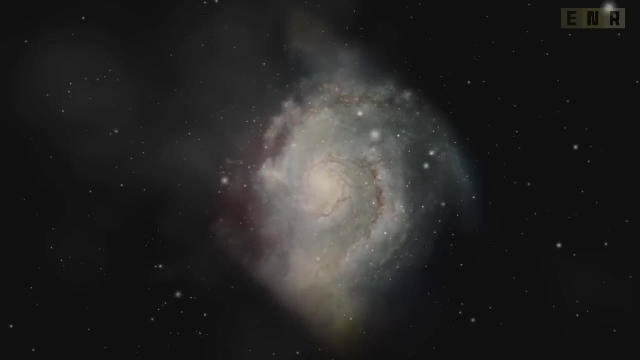 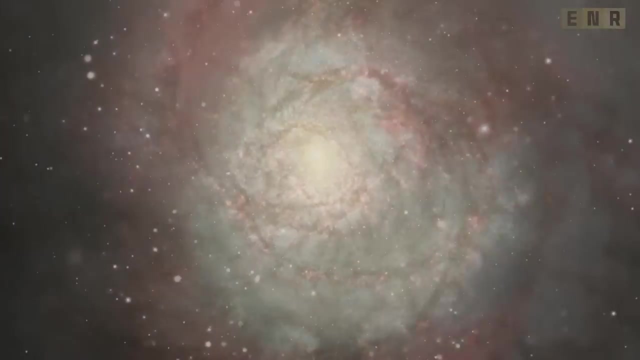 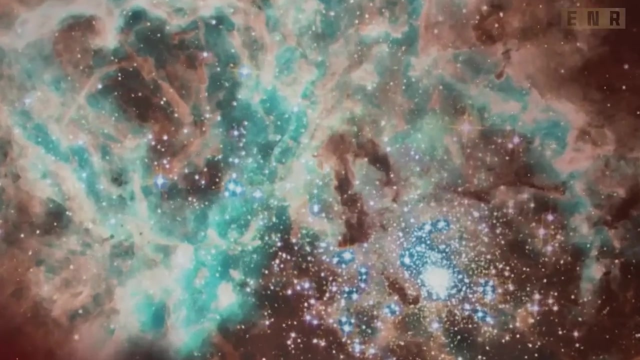 Too far away from the center would be just as bad. Out there there aren't as many stars, We might not exist at all. We are therefore, in a sense, in the Goldilocks zone of the galaxy: Neither too close nor too far away, but just right. 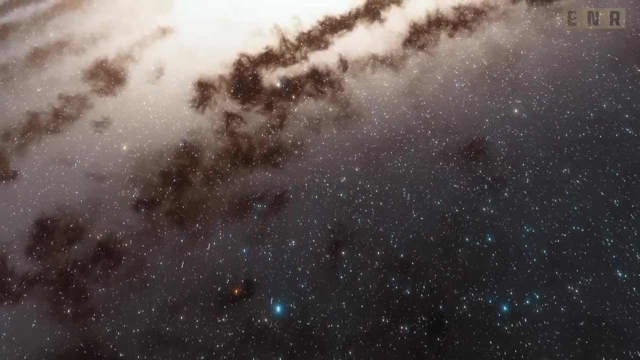 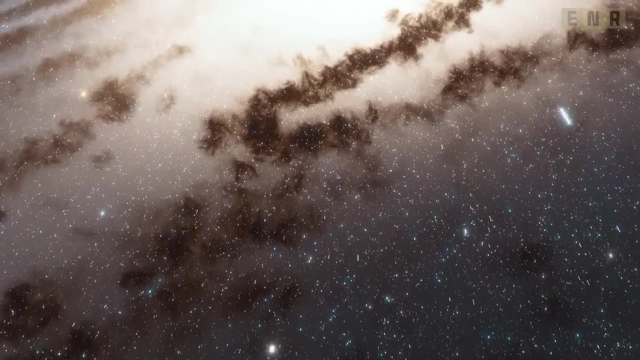 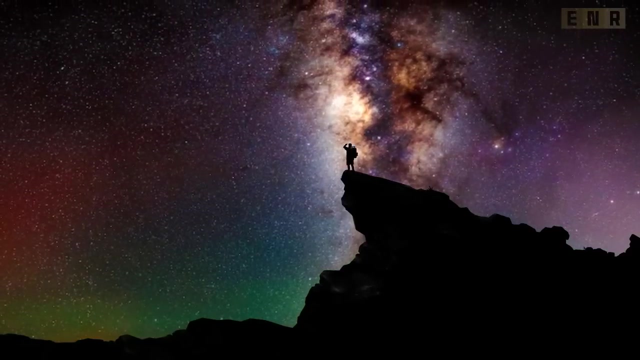 There may be millions of stars in the cosmic Goldilocks zone, where conditions are just suitable for life. Furthermore, if our galaxy can support life, then other galaxies should be able to as well. The cosmos is very large, and the really incredible part is that we continue to learn new things about it. 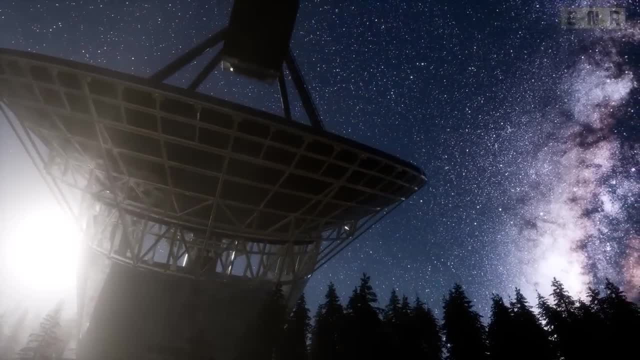 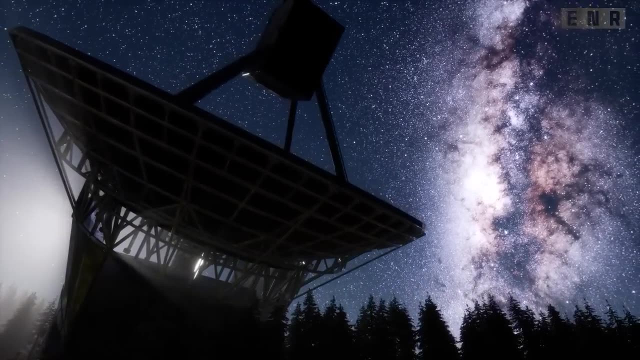 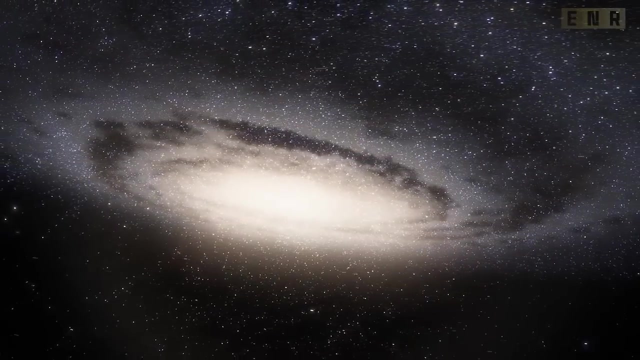 Every time we believe we've figured out a solution to an issue, we uncover that it's really part of an even greater one. That's awesome. Our Milky Way galaxy and the galaxies beyond it are rife with mysteries and unanswered questions. Who would have guessed 20 years ago? 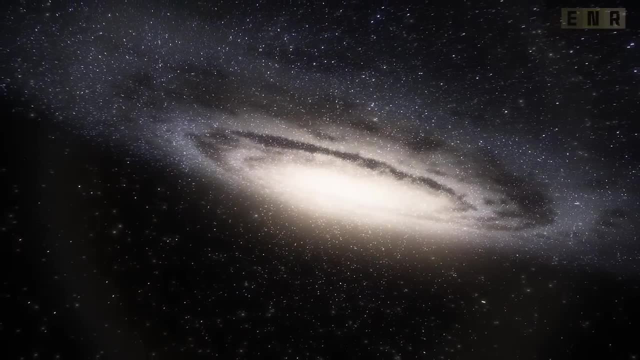 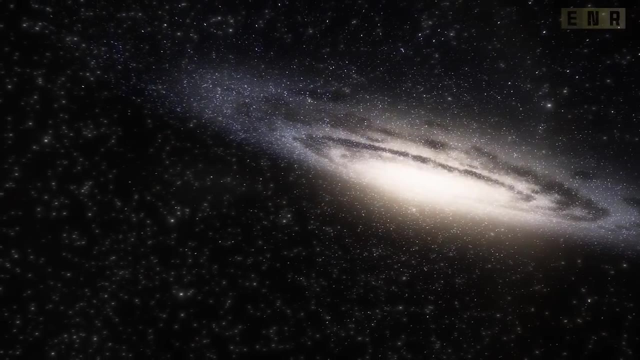 that we would be able to identify the black hole at the center of the galaxy. Who would have predicted 20 years ago that the astronomical community would accept the existence of dark matter and dark energy? We should be astonished to be alive at this particular moment in cosmic history. 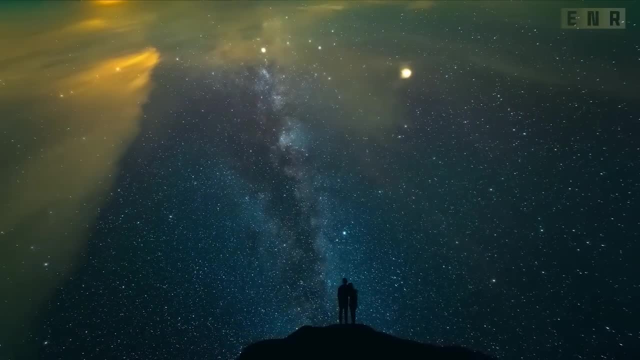 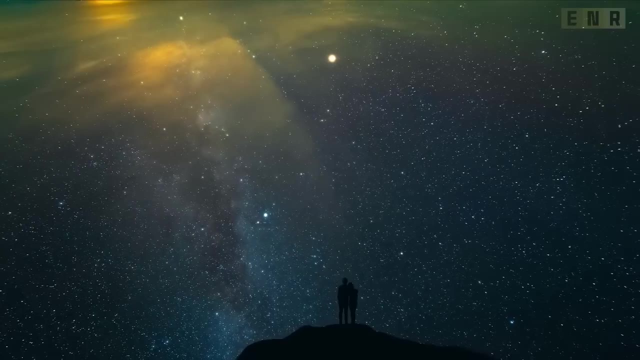 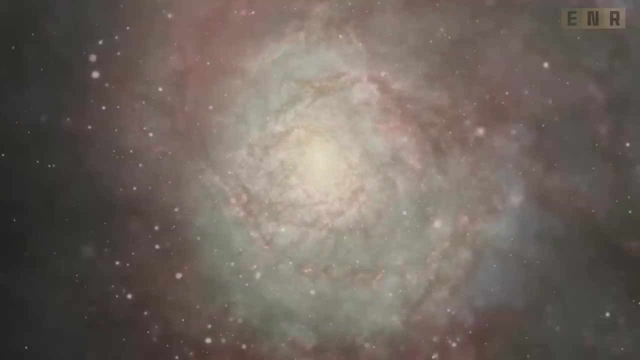 on this particular planet, on the fringes of this particular galaxy, with the ability to ponder questions and seek answers. across the whole cosmos, Galaxies are born, they evolve, they collide and they die. The Milky Way is a fortunate home for intelligent life. 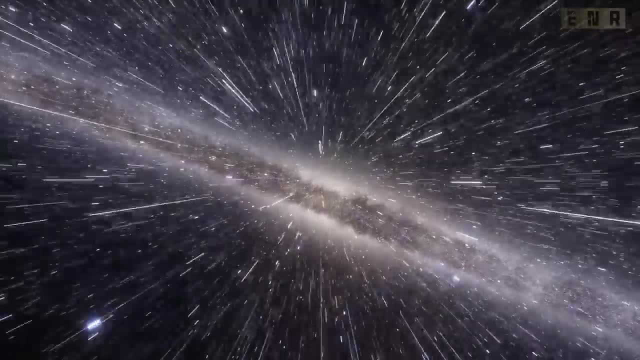 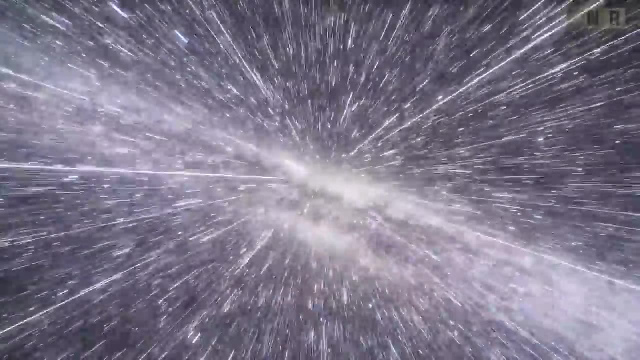 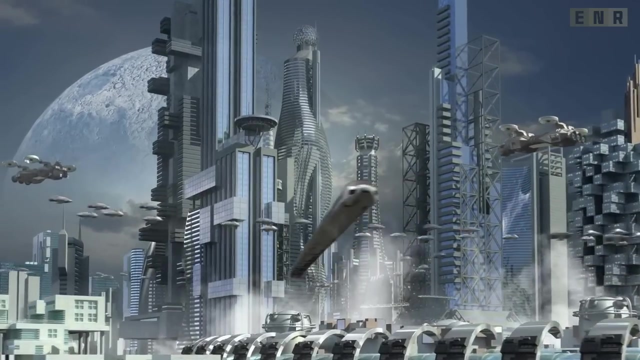 Our fate is intertwined with that of every galaxy. Ultimately, our fate rests in their hands, since they are the ones who created us and are shaping our identities. Ladies and gentlemen, welcome to today's topic: aliens. Are they real? Do they exist? 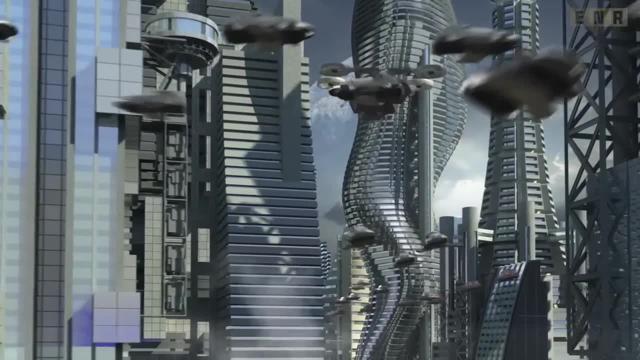 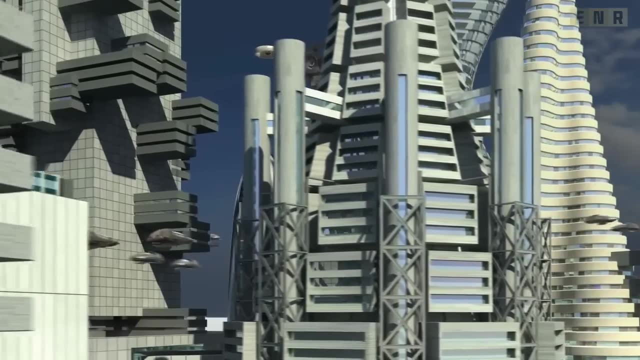 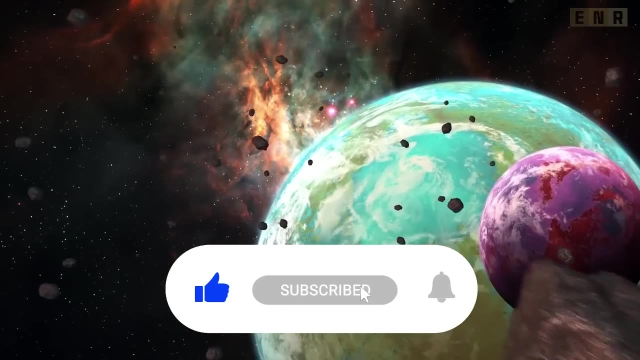 And if so, what do they look like? Today, we will dive deep into the topic of aliens, exploring various theories and facts about these mysterious creatures. If you are interested in amazing videos about the universe, be sure to subscribe to our channel to stay updated. 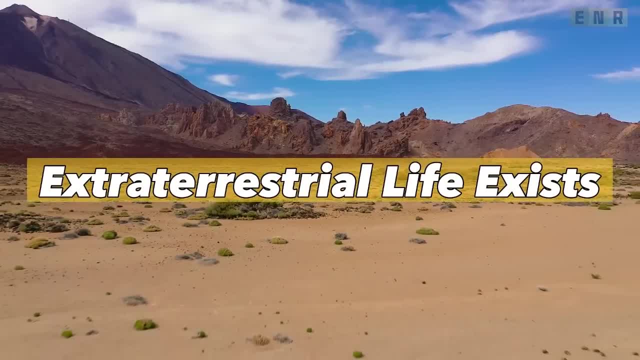 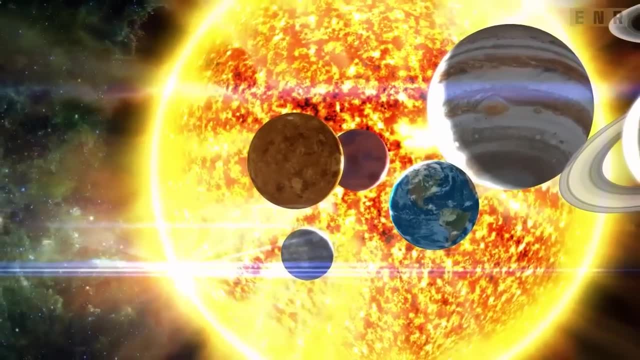 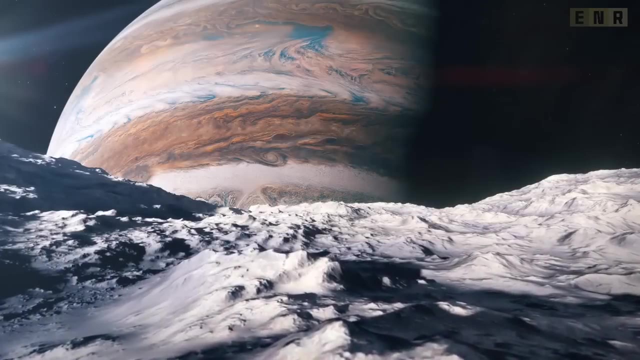 Here are a few theories about aliens. Extraterrestrial life exists. This is the theory that life exists elsewhere in the universe, perhaps even within our own solar system. Microbial life could potentially exist on Mars or some of the moons of Jupiter and Saturn, for example. 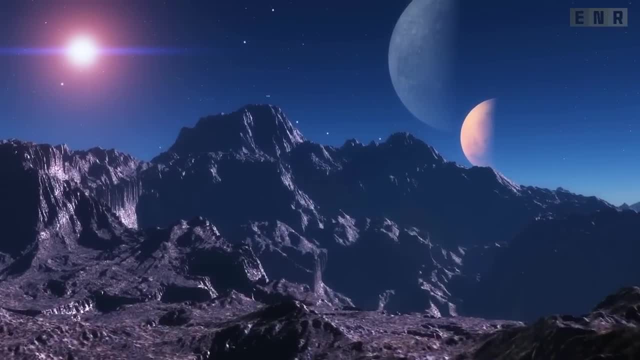 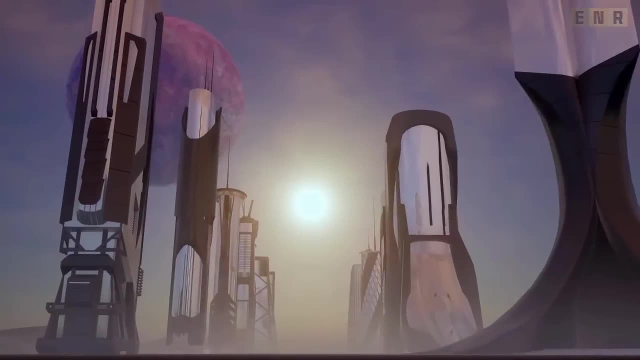 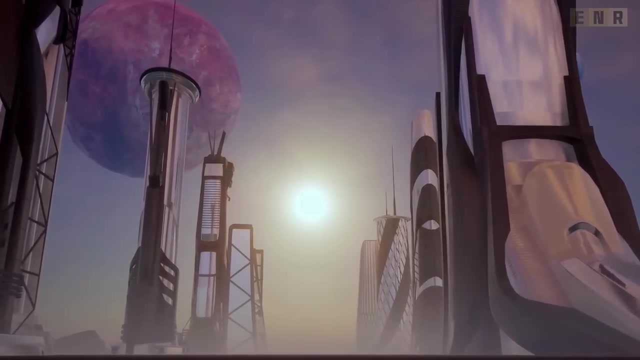 More complex life forms, such as intelligent civilizations, could also exist on planets orbiting other stars. The Fermi Paradox. The Fermi Paradox suggests that if intelligent life is common in the universe, why haven't we detected any evidence of it? 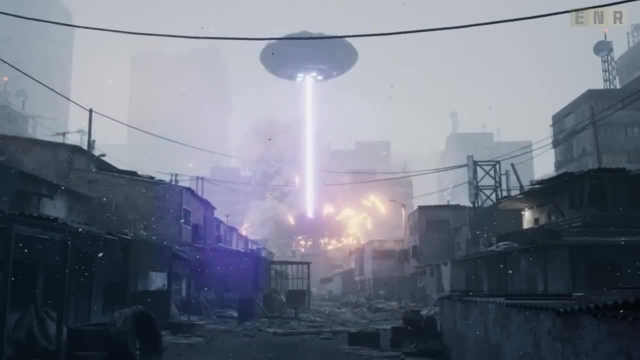 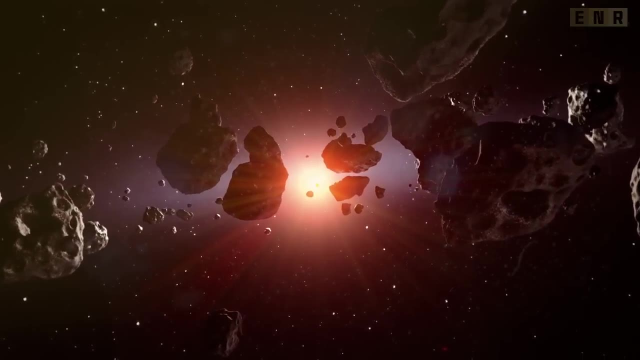 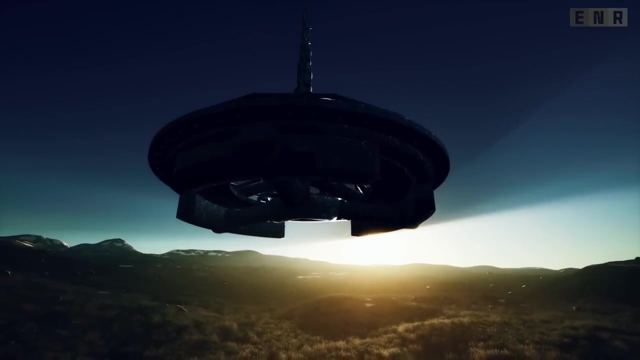 Some theories suggest that intelligent civilizations tend to self-destruct, while others propose that they are too far away or have no desire to communicate with us Ancient aliens. This theory suggests that aliens have visited Earth in the past and have influenced human history and culture. 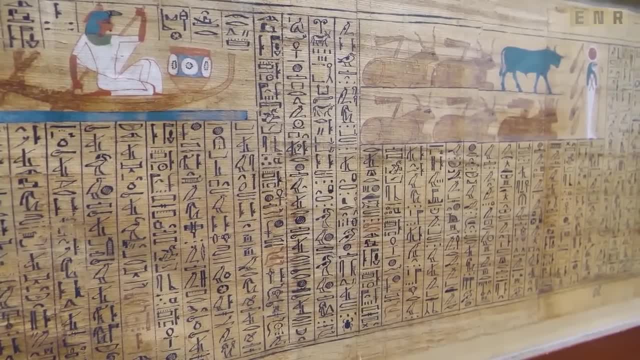 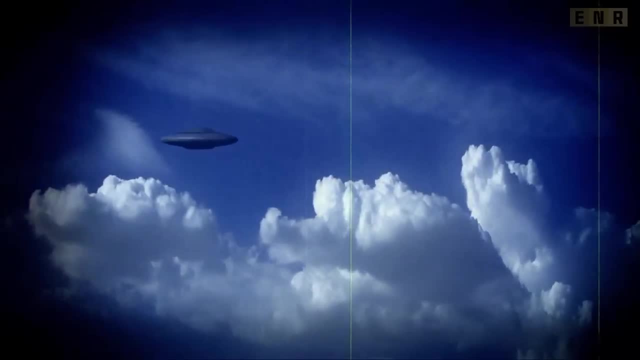 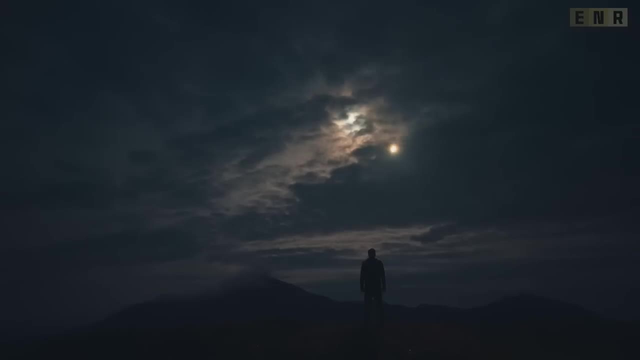 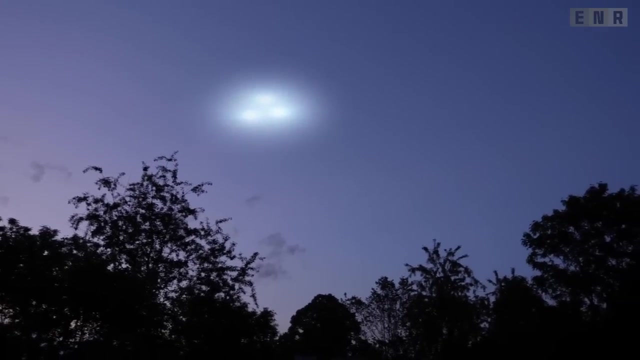 Proponents of this theory point to ancient artwork and texts as evidence of alien visitation. UFO sightings- Unidentified flying objects are often cited as evidence of alien visitation. While many sightings can be explained by natural phenomena or human-made objects, some remain unexplained and could potentially be evidence of extraterrestrial visitation. 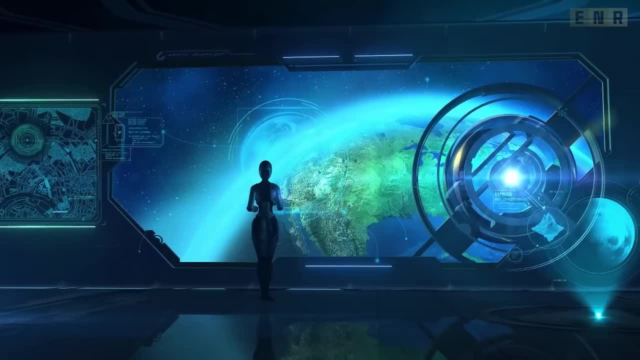 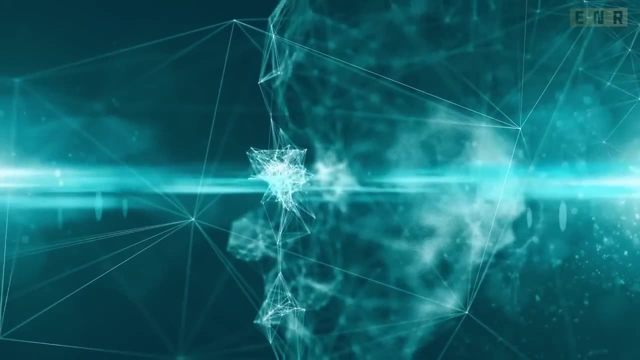 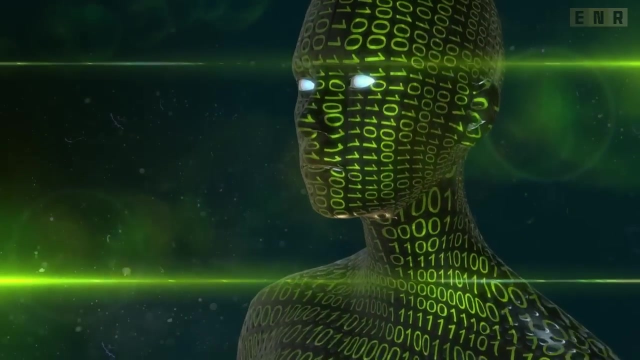 The Simulation Theory. This theory proposes that our entire reality is a computer simulation created by an advanced civilization. While not specifically about aliens, this theory suggests that the creators of the simulation could potentially be an extraterrestrial civilization. To start with, let's address the most basic question. 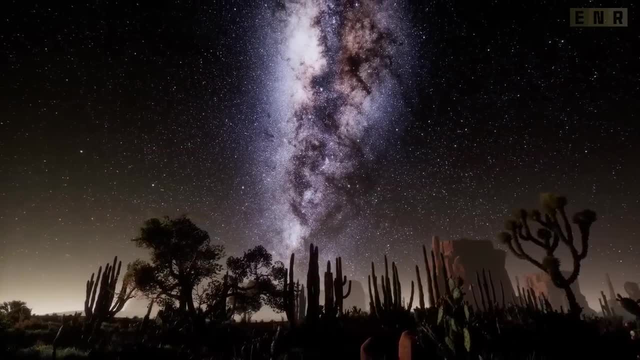 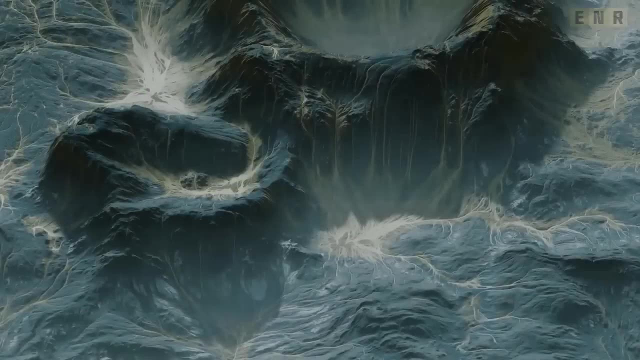 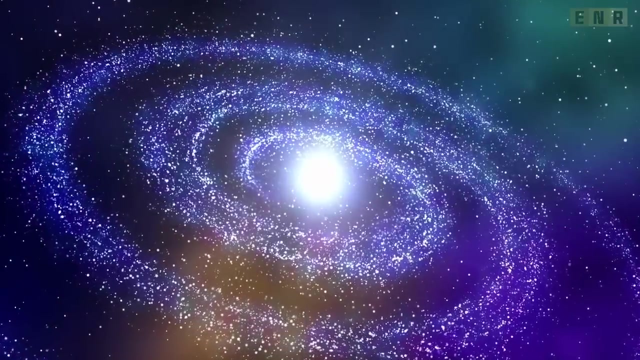 do aliens exist? Well, according to the Drake Equation, which was developed in 1961 by astronomer Frank Drake, the probability of intelligent life existing elsewhere in the universe is high. The equation takes into account factors such as the number of stars in our galaxy. 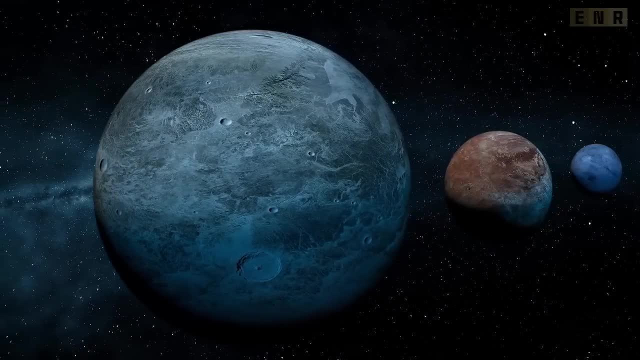 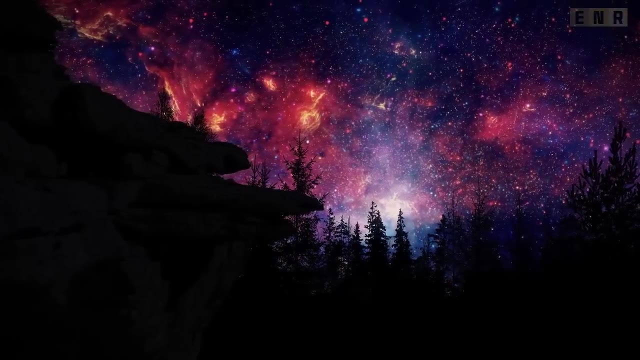 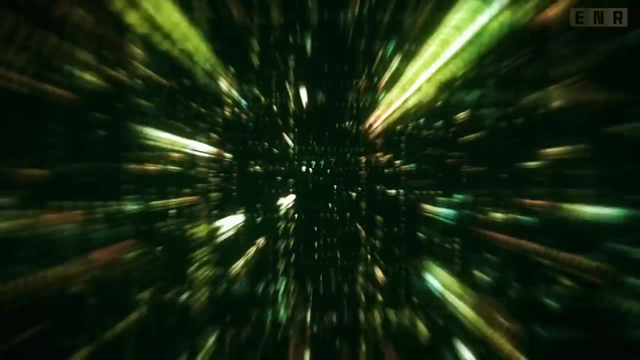 the number of planets that could potentially support life and the probability of life forming on those planets. Using these factors, the Drake Equation estimates that there could be millions of intelligent civilizations in our galaxy alone, But the question remains: have we ever encountered these civilizations? 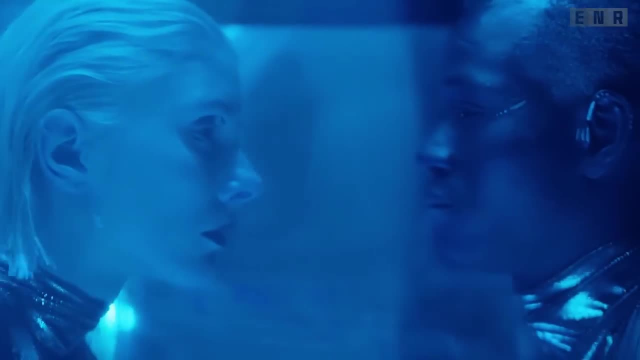 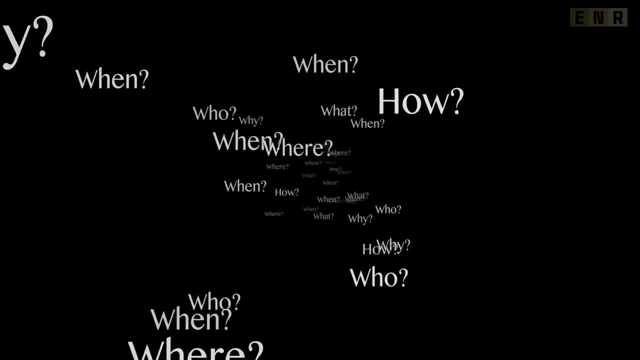 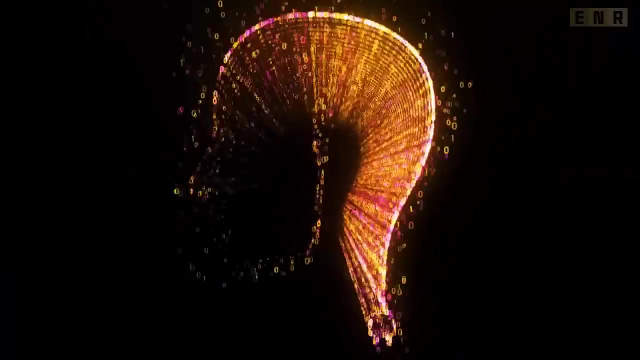 Many people believe that we have, and there are countless stories of alien sightings, abductions and encounters. However, there is little concrete evidence to support these claims, So let's explore some of the most popular theories about what aliens might look like. 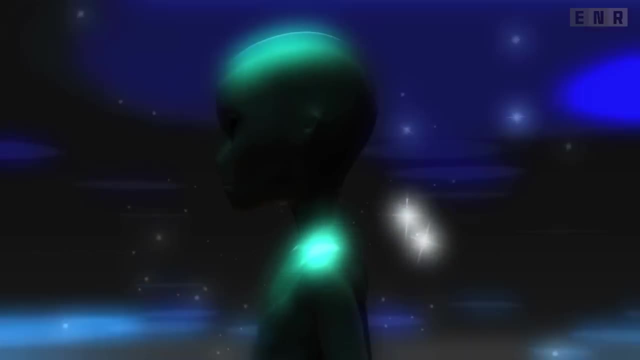 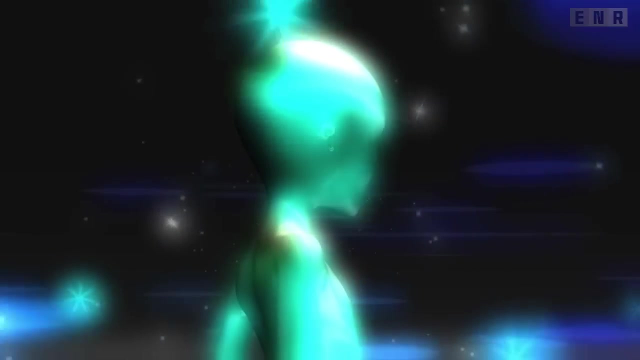 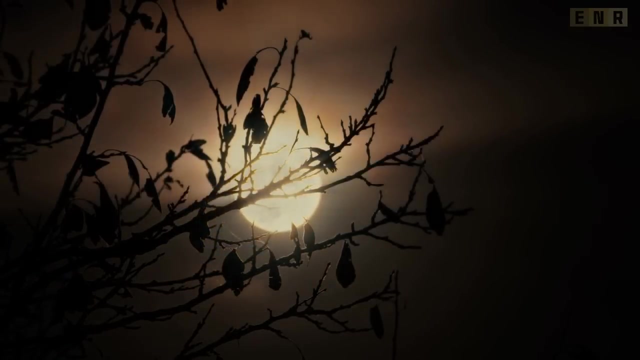 The traditional image of aliens as small, green, big-eyed beings is a product of popular culture. However, it is unlikely that aliens would look anything like this. In fact, it is impossible to predict what aliens might look like, as their appearance would depend on the conditions of the planet they evolved on. For example, if an alien species evolved on a planet with high gravity, they might have shorter, stockier bodies. If they evolved on a planet with a harsh, radiation-filled environment, they might have evolved to be more resilient to radiation. It's also possible that some alien species might not even have bodies as we know them. 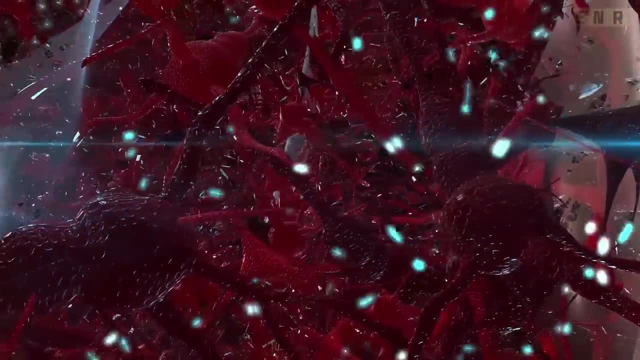 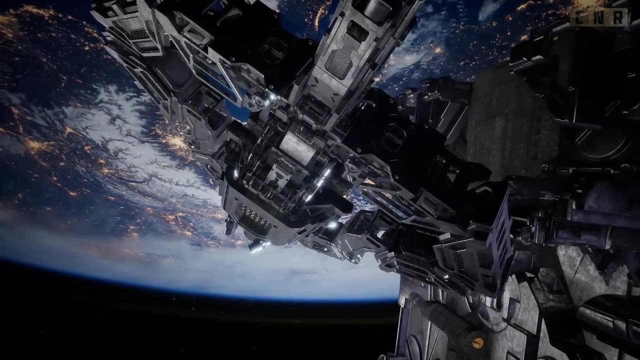 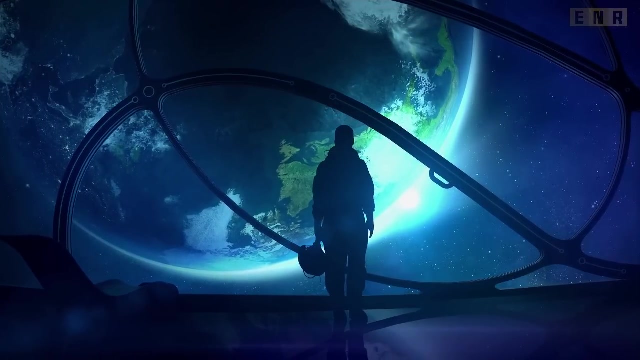 They might exist as pure energy or as a hive mind collective. But why would aliens visit Earth? There are a few possible reasons. Some scientists speculate that aliens might be interested in our planet. because of its unique location in the universe, Earth is in a Goldilocks zone. 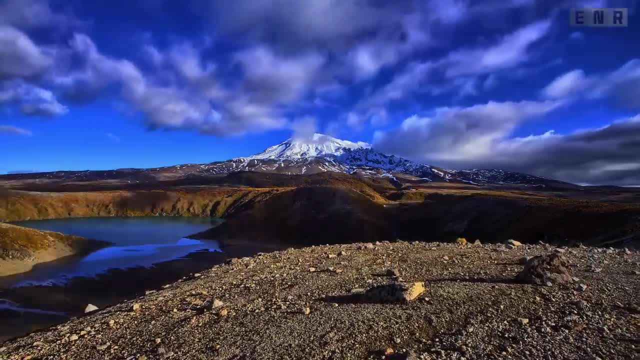 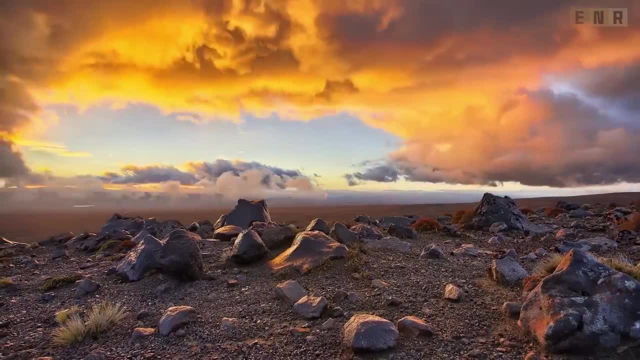 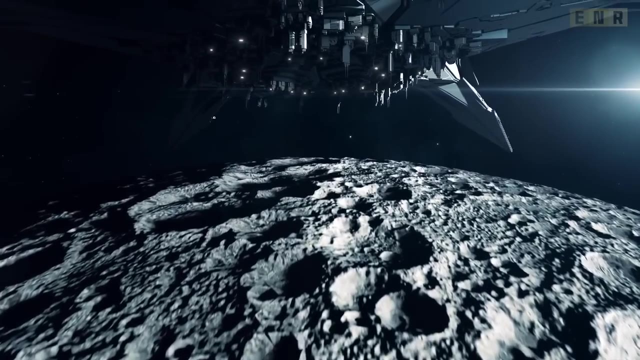 It's not too hot, not too cold and has the right conditions for life to thrive. Aliens might be interested in studying our planet to learn more about how life can survive in these conditions. Another reason aliens might visit Earth is to make contact with us. 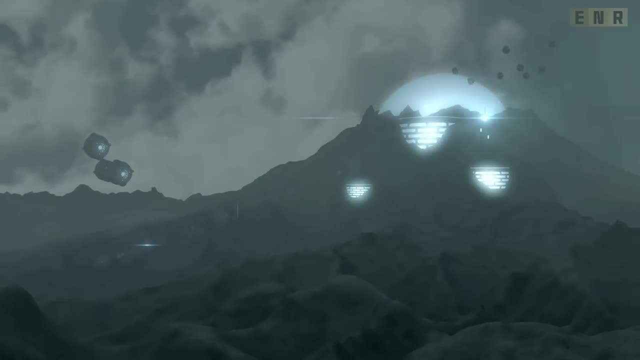 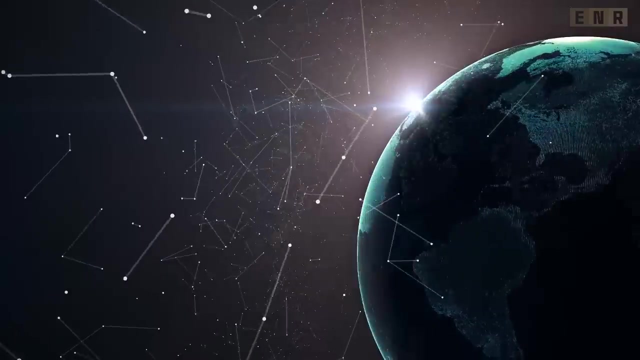 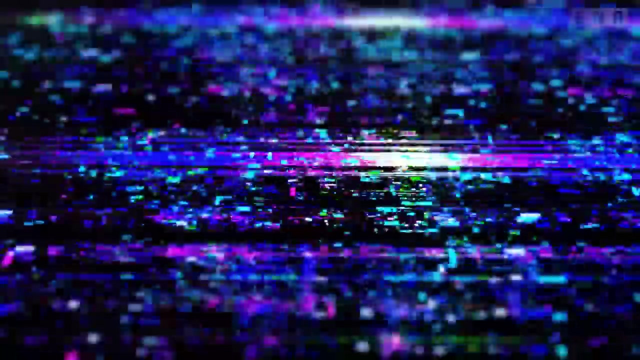 If there are millions of intelligent civilizations in the galaxy, it's possible that some of them are trying to communicate with us. However, if this is the case, they might be communicating in ways that we can't even comprehend. Their methods of communication might be vastly different from ours. 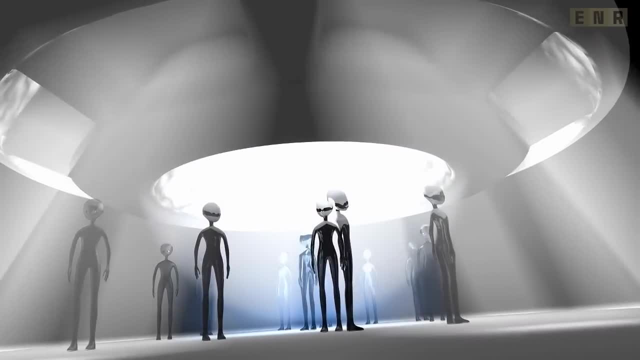 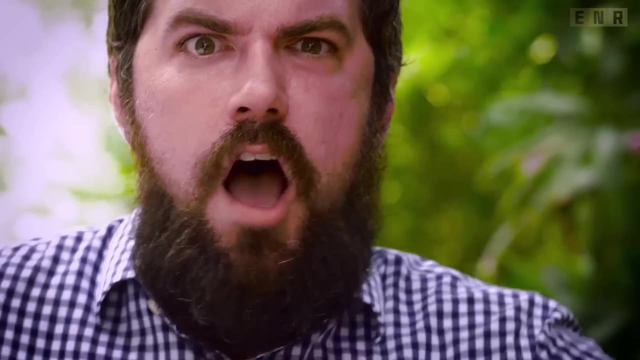 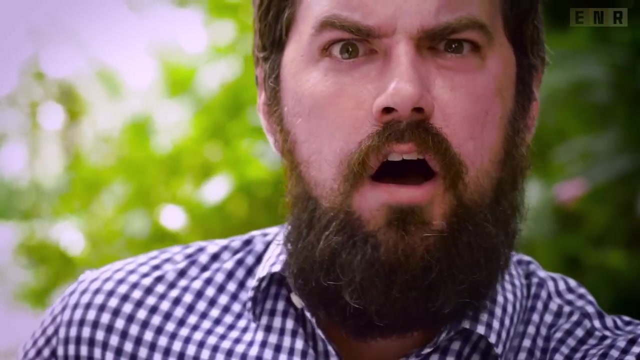 So what should we do if we ever do encounter aliens? Many scientists believe that we should approach any encounter with caution. We should avoid making any sudden movements or aggressive actions, as these might be misinterpreted by the aliens. Instead, we should attempt to communicate in a peaceful and non-threatening manner. 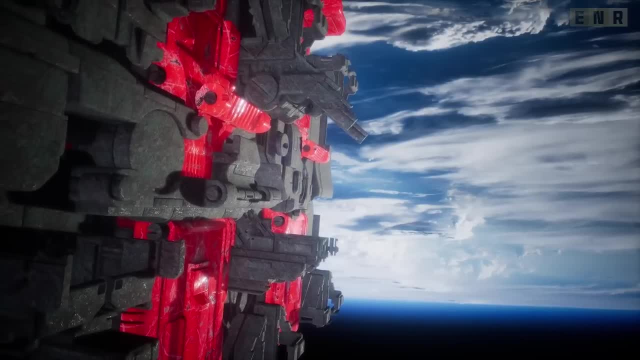 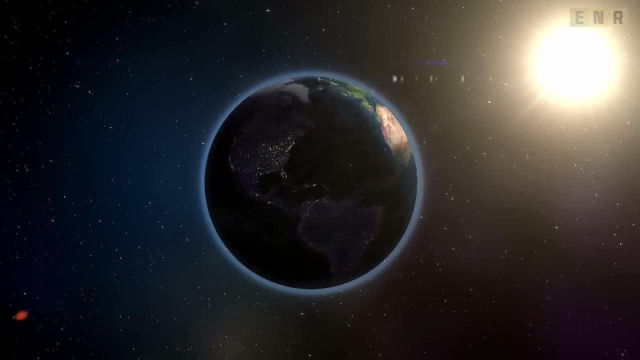 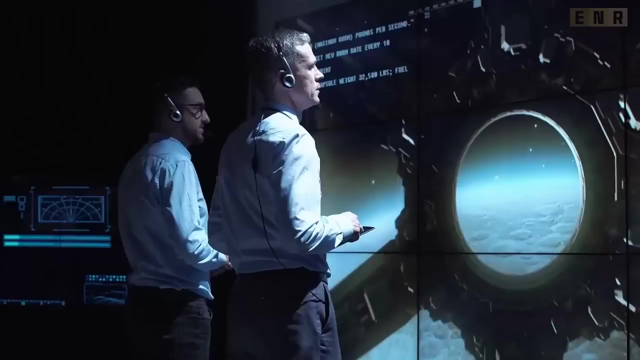 If we do make contact with aliens, it could have profound implications for our understanding of the universe. It could challenge our beliefs about our place in the cosmos and force us to confront some of the big questions about life, the universe and everything. Now that we've explored some of the theories and possibilities of alien life, 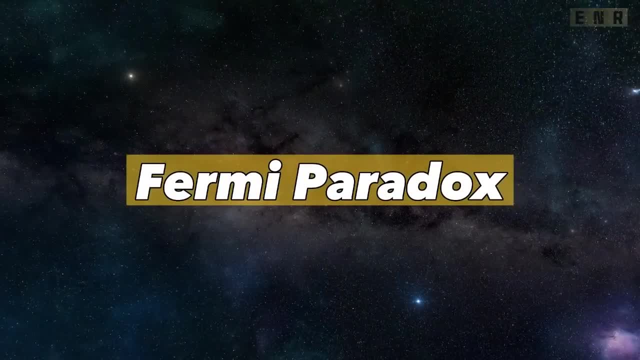 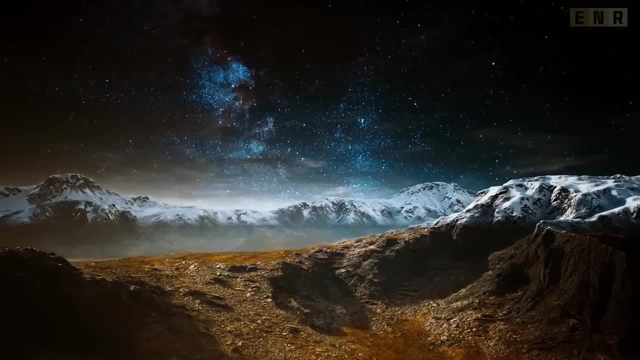 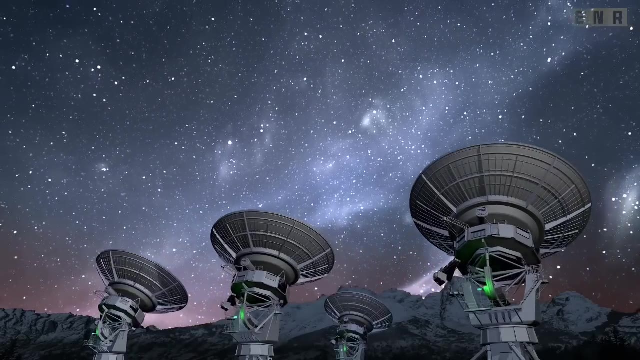 let's consider the idea of the Fermi Paradox. This paradox asks the question: if there are so many intelligent civilizations out there, why haven't we seen any evidence of them? Why haven't we detected any signals or observed any spacecraft from other worlds? 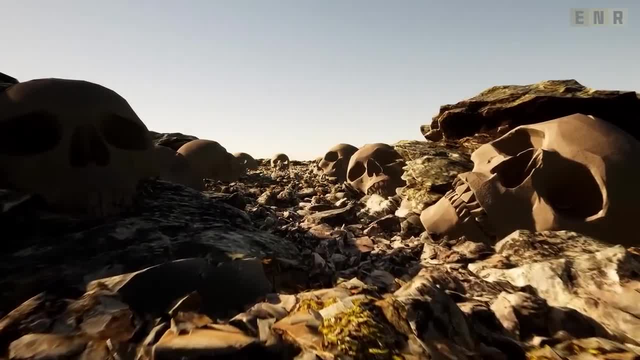 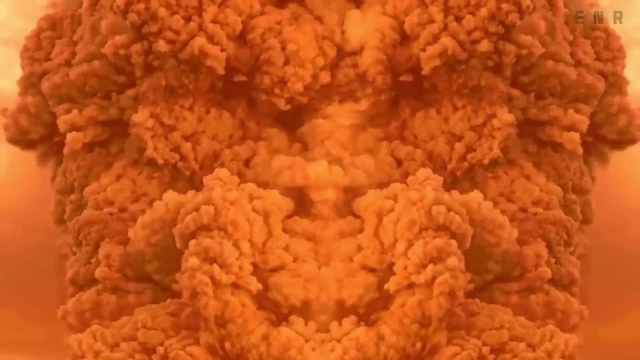 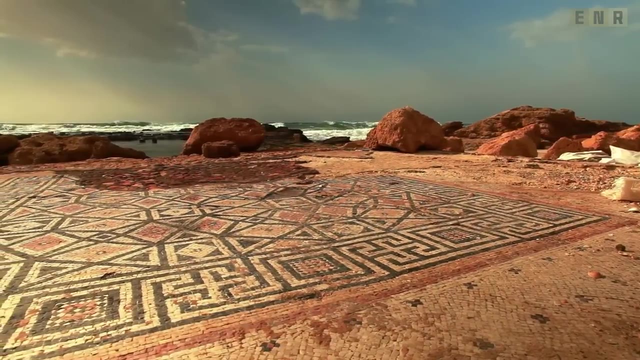 One possibility is that advanced civilizations tend to self-destruct. With technology comes the potential for destruction, whether through environmental damage, war or some other catastrophe. It's possible that many intelligent civilizations reach a point where they are unable to sustain themselves and ultimately fail. 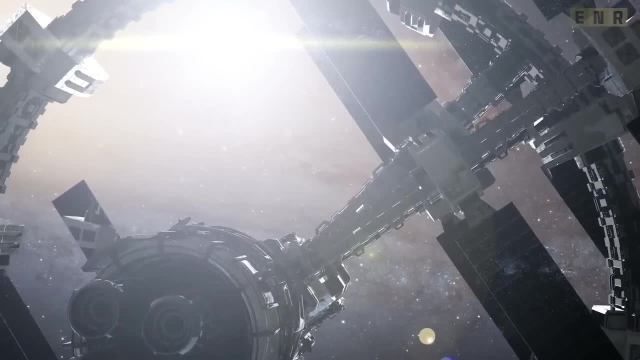 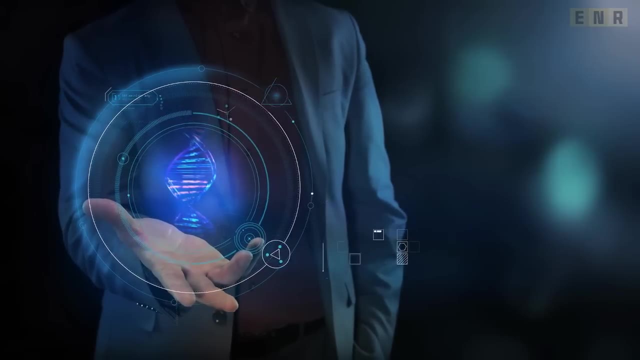 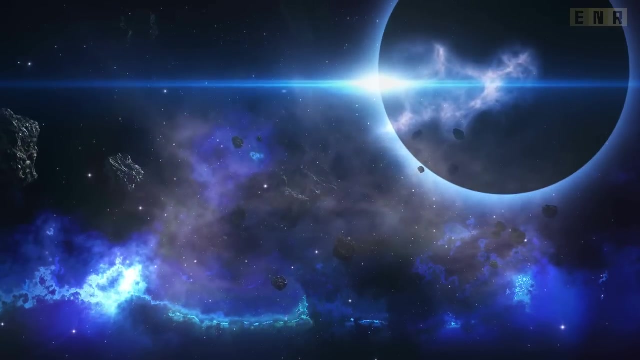 Another possibility is that intelligent civilizations have no desire to make contact with us. Perhaps they are simply not interested in Earth or in communicating with other species, Or perhaps they are too far away to detect our signals and we are too primitive to detect theirs. Regardless of the reasons, 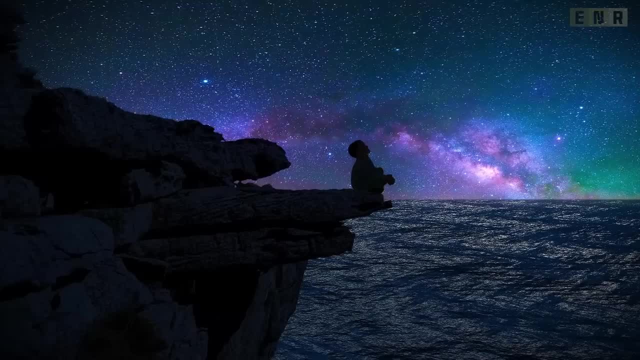 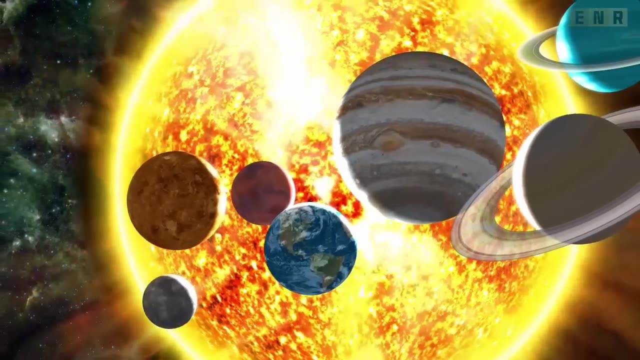 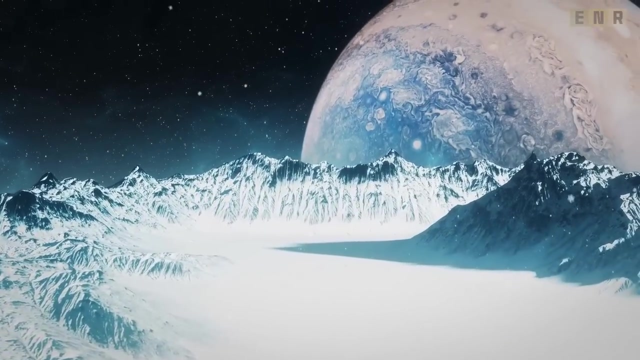 the Fermi Paradox remains a mystery and a subject of much speculation, But let's turn our attention to the possibility of life in our own solar system. While we haven't found any evidence of intelligent life, there are some promising signs that microbial life 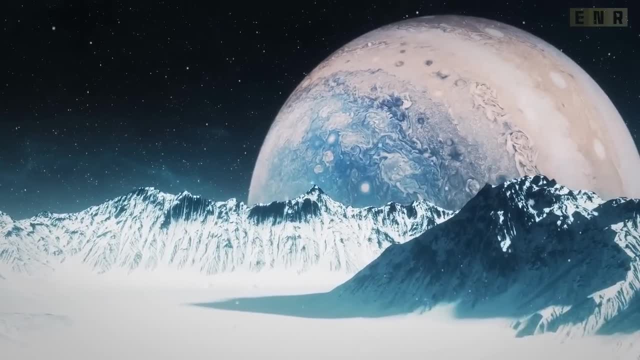 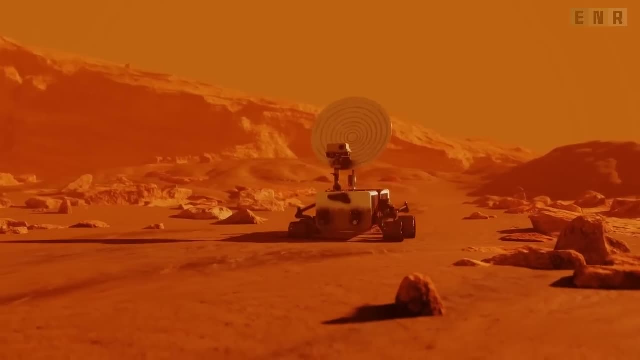 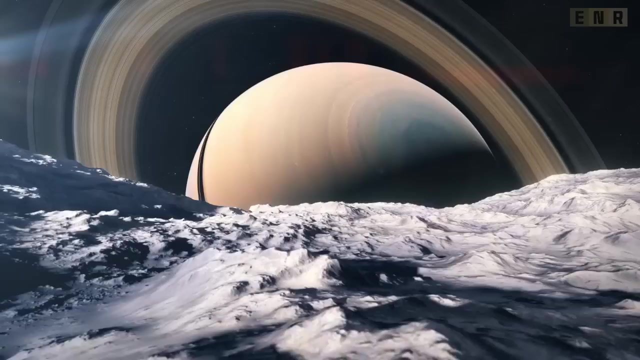 might exist on other planets or moons. For example, NASA's Mars rover has detected methane on the planet's surface, which could be a sign of microbial life, And scientists have found evidence of subsurface oceans on some of Jupiter and Saturn's moons. 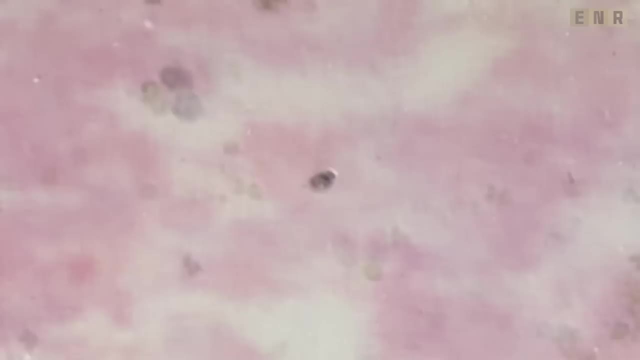 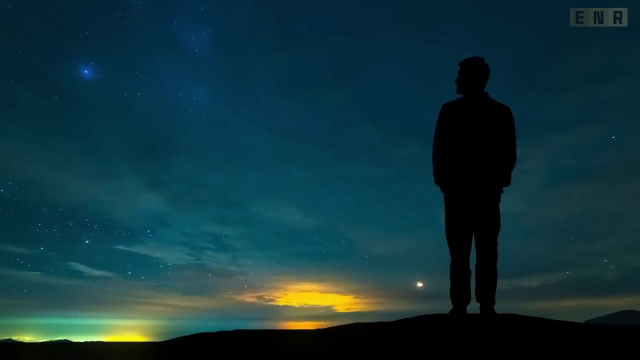 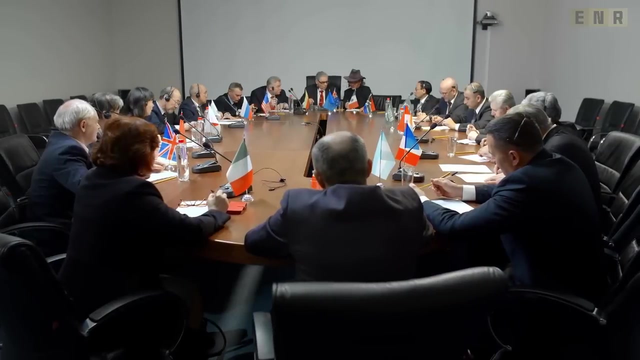 which could potentially support life. If we do find evidence of microbial life in our own solar system, it would be a major discovery and could have significant implications for our understanding of life in the universe. Let's consider the potential implications of discovering intelligent life. 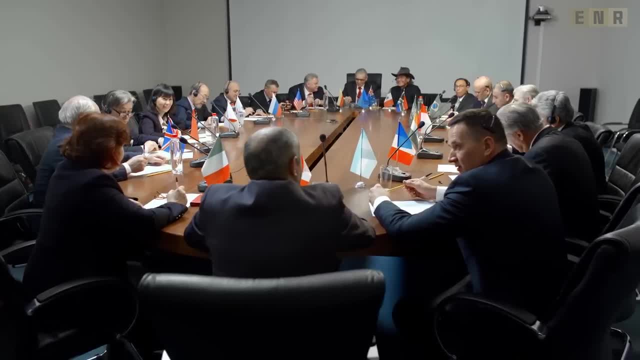 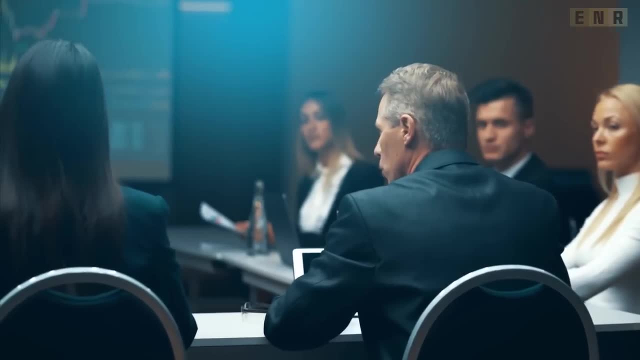 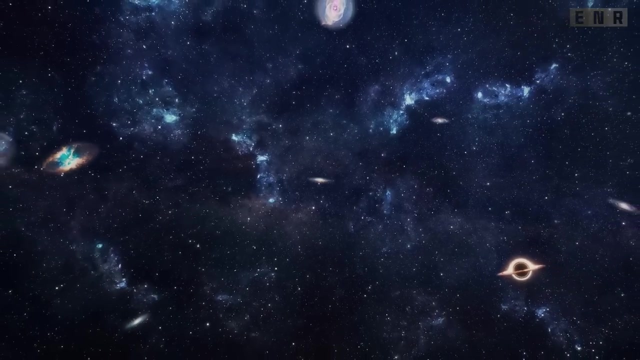 If we were to make contact with an alien civilization, it could have profound impacts on our society and our understanding of the universe For one. it could challenge our existing beliefs and worldviews. We might need to re-evaluate our ideas about our place in the cosmos. 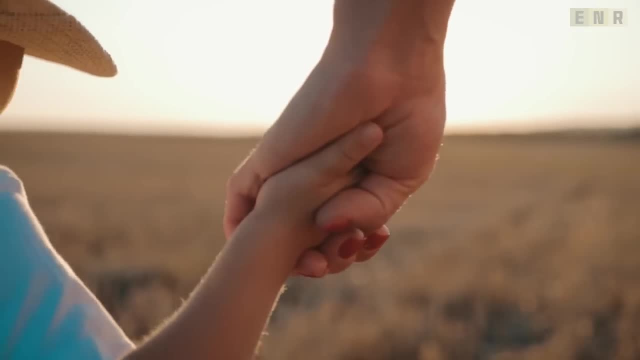 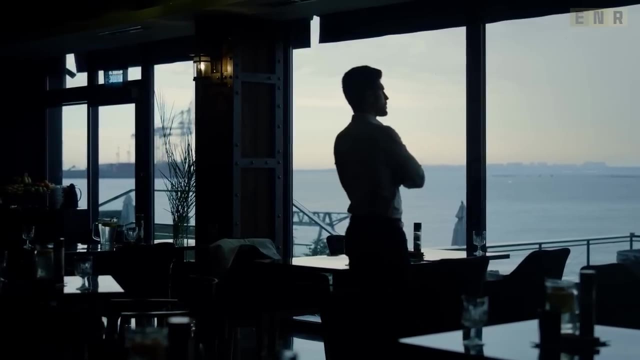 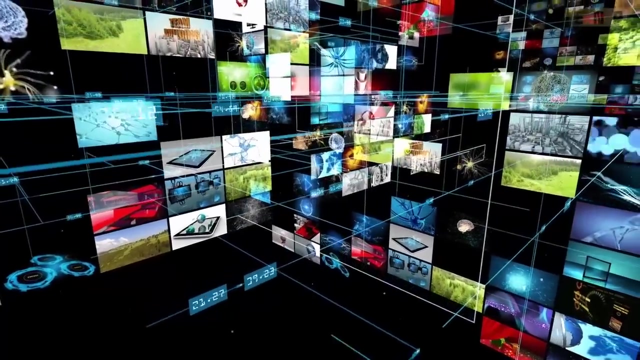 our religious and philosophical beliefs and our understanding of the origins of life. It could also raise questions about the ethics of interacting with other intelligent species and the responsibilities that come with such interactions. Another potential impact is on our technology and scientific progress, If we were to encounter 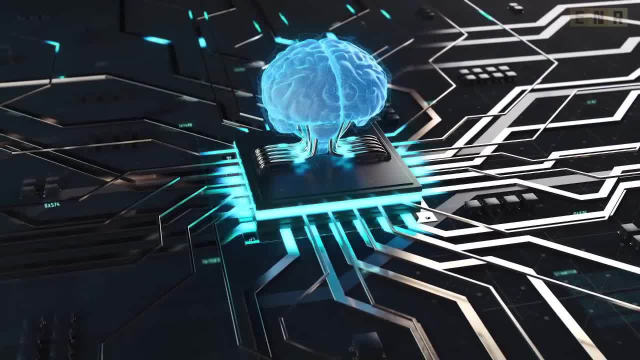 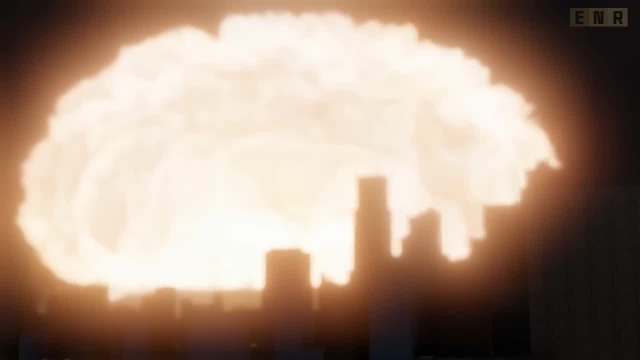 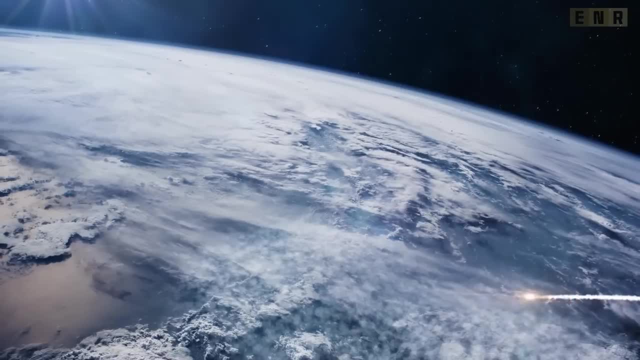 a more advanced civilization. we could learn from their technology and knowledge, potentially accelerating our own progress. On the other hand, it could also pose a threat if the aliens have hostile intentions towards us. It's difficult to say for certain whether aliens, if they exist. 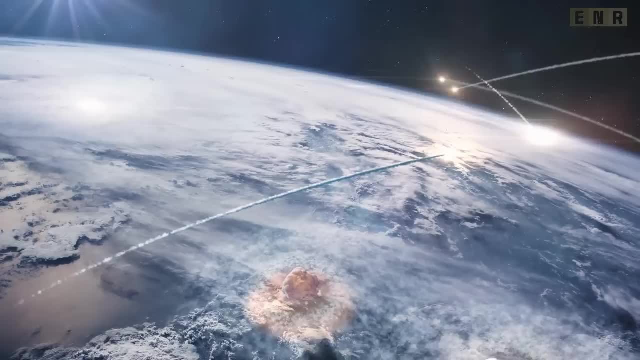 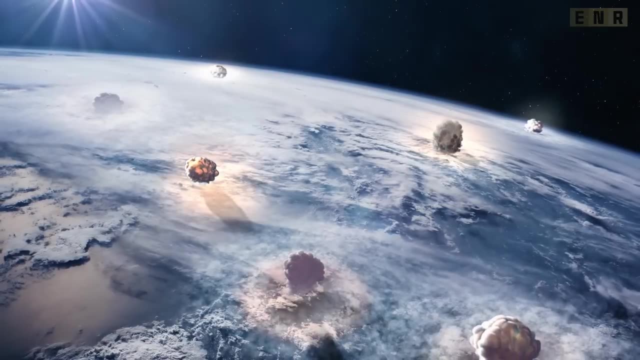 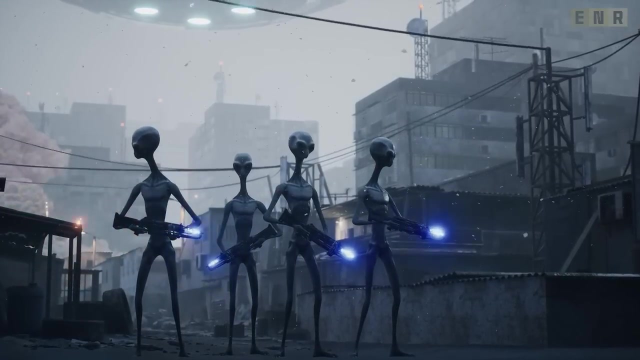 would be dangerous to us. We have no concrete evidence of intelligent extraterrestrial life, and so any speculation about their intentions or behaviors is purely hypothetical. Some people argue that aliens could be dangerous if they are more technologically advanced than us and have the ability to conquer or destroy us. 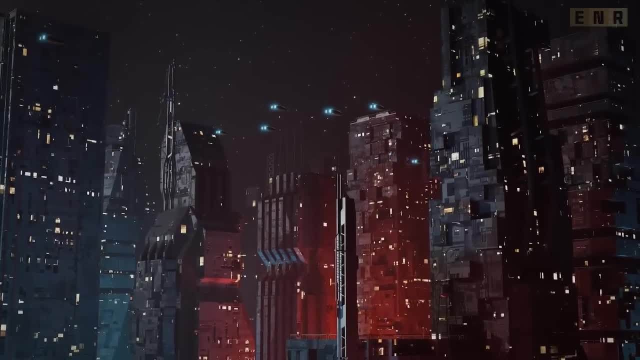 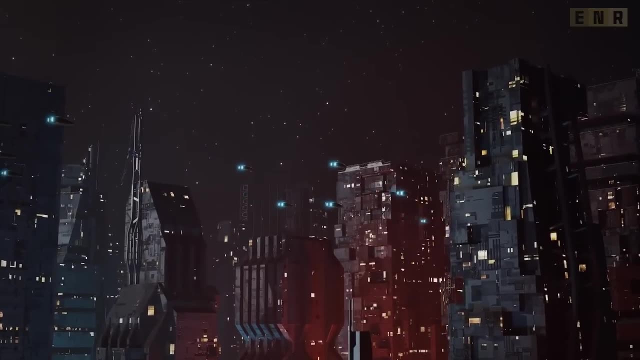 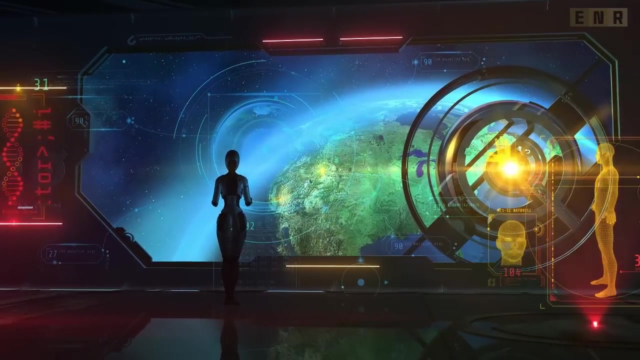 Others point out that any civilization advanced enough to travel through space would likely have a more sophisticated understanding of the universe and may be more peaceful and cooperative. It's also possible that aliens could be indifferent to us, simply observing us from a distance without any intention. 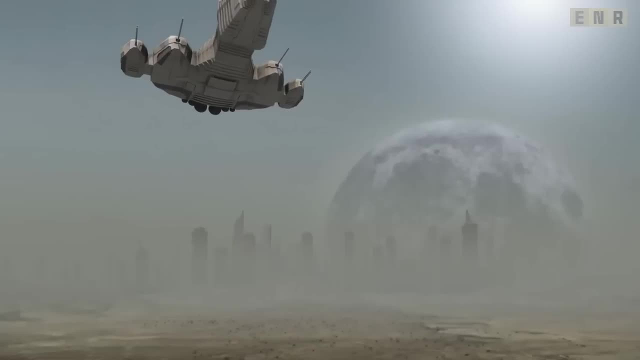 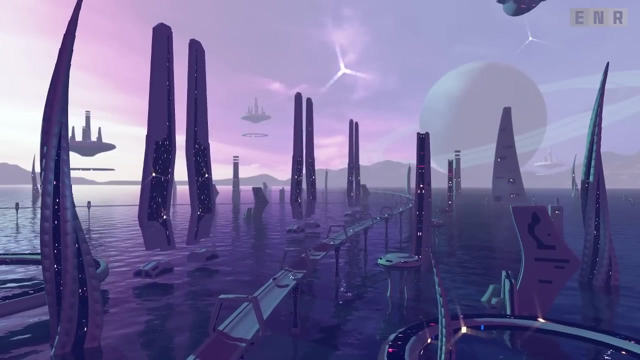 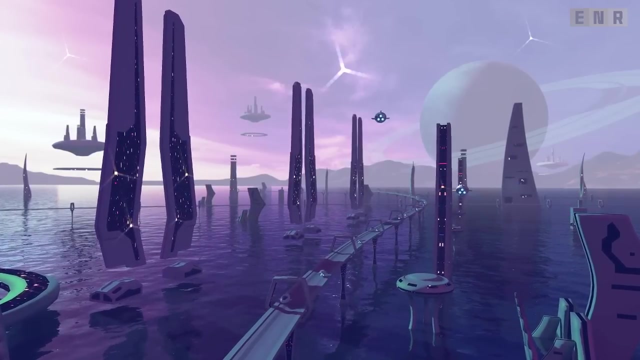 to interact with us at all. Overall, while it's fun to speculate about the potential dangers of alien life, the truth is that we simply don't know enough to make any definitive conclusions about their intentions or behaviors. The search for extraterrestrial life.